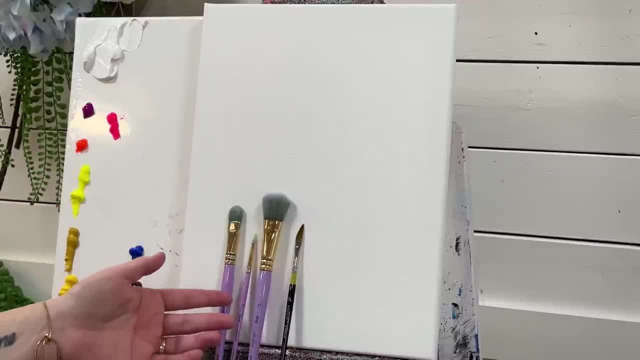 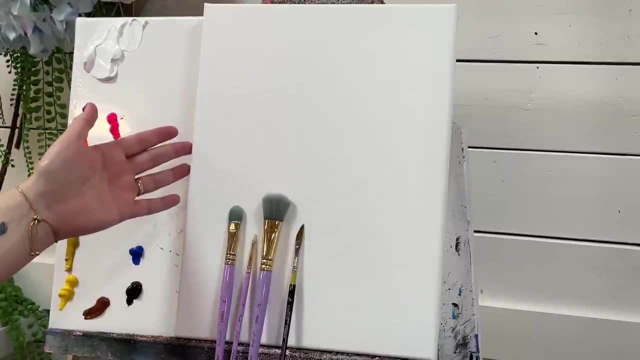 brushes here as well: 14 filbert, a number three round, a one inch mop brush and a quarter inch dagger brush. I'll be painting this on an 11 by 14 inch canvas and we're going to go ahead and paint the bottom of the flower. I'm going to be using a number three round. 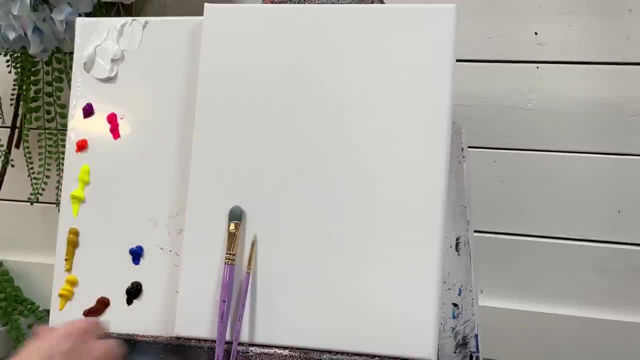 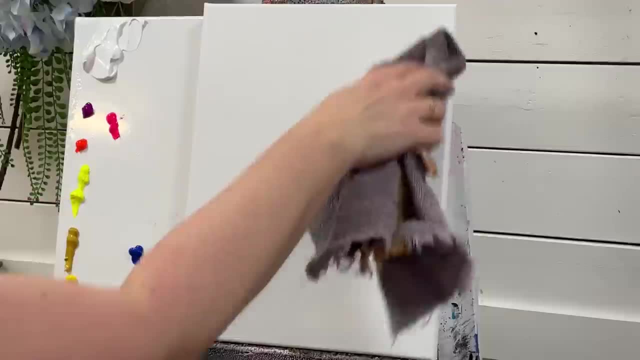 with the very first step Now. the first thing I'm going to do is just add a little bit of water to my towel here and I'm going to just apply it over the canvas. I'm just going to get the canvas a little damp first. that way it'll take my paint a lot easier. 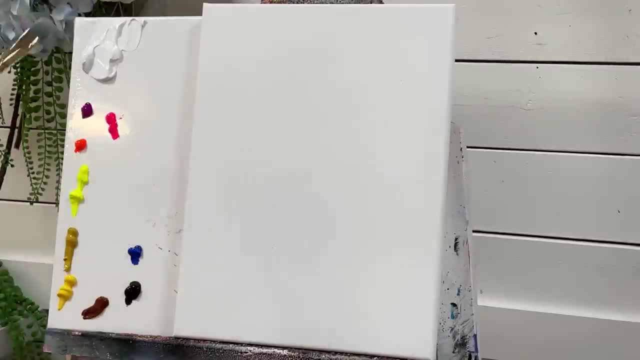 The first brush I'm going to be using, for this is my 14 filbert brush. What I want to do is add a lot of the darker colors. I'm just going to be blocking in colors at this point, darker ones, and then we're going to work our way up to our brightest. 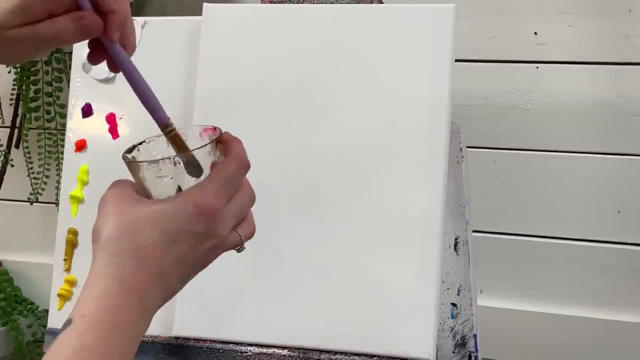 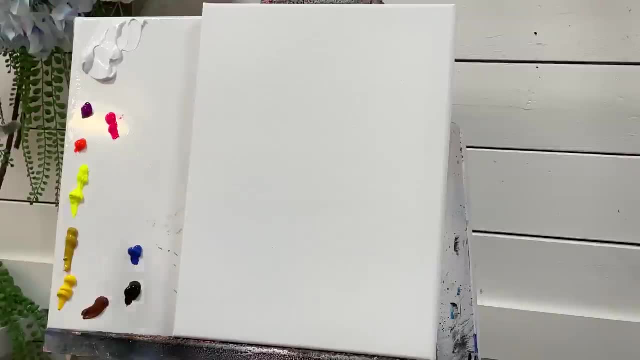 most vivid colors. So I'm going to use this filbert brush. take just a little bit of water. even though I've got water on the canvas, I want to moisten the bristle so the paint doesn't ruin the brush, And I'm going to start off with my violet here and I'm just going. 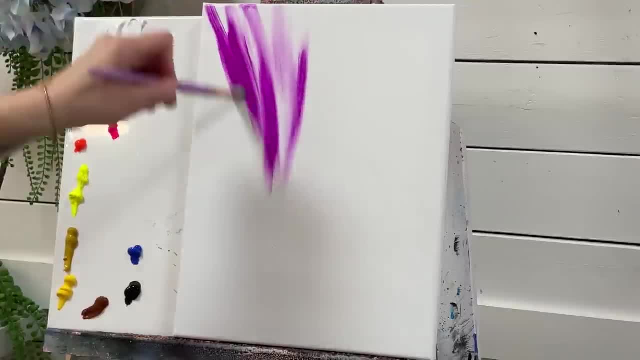 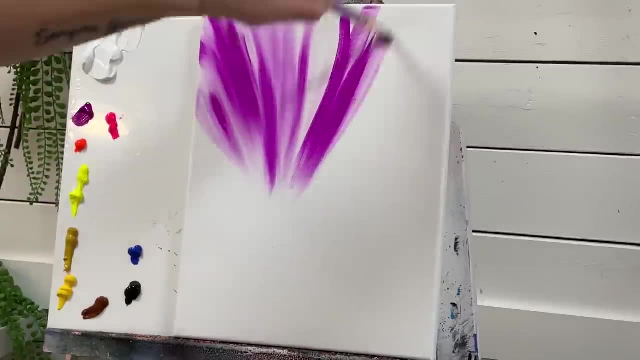 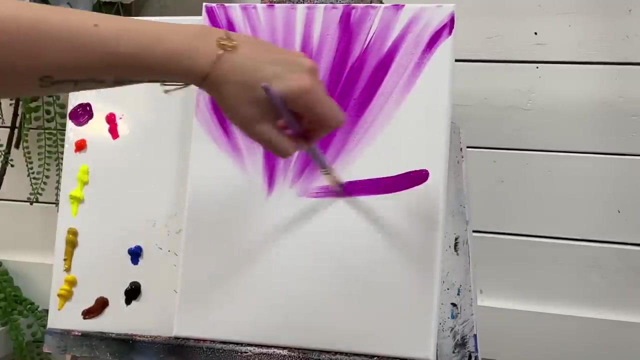 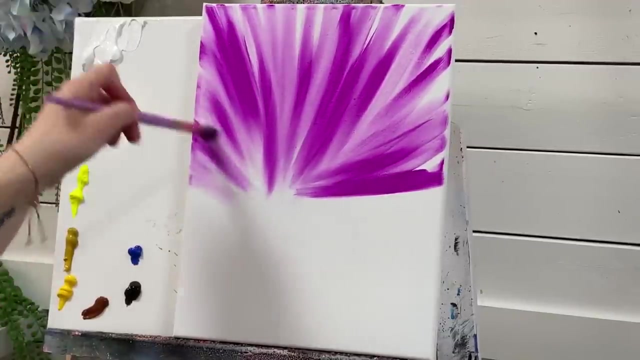 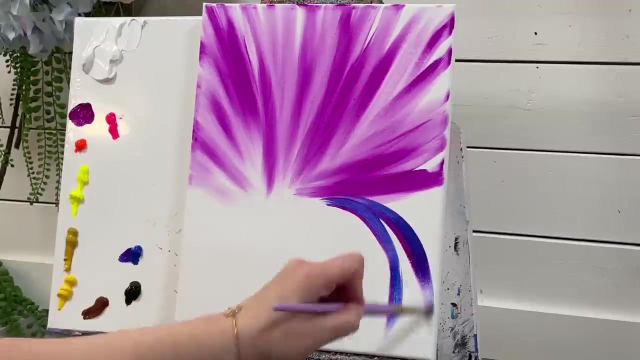 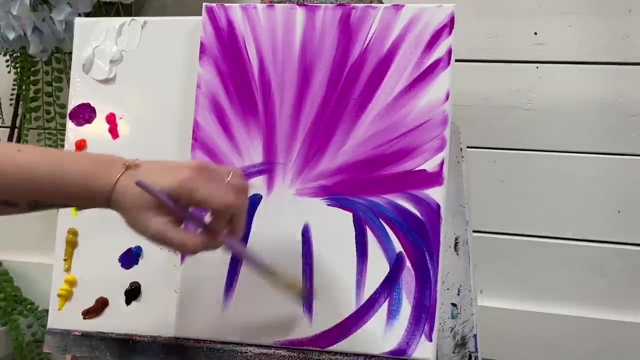 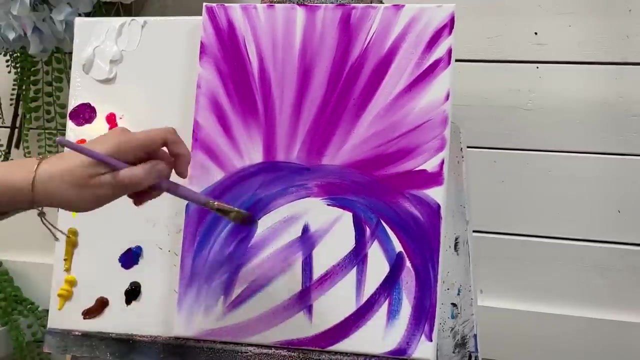 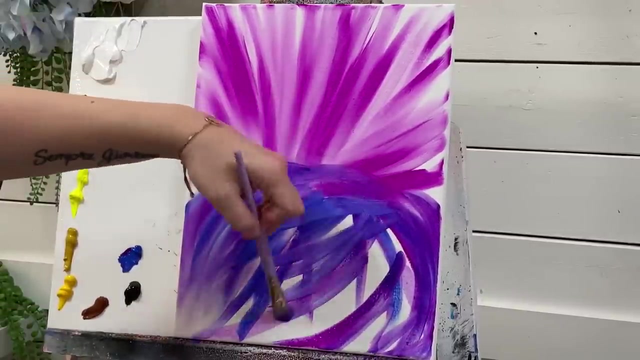 to start going kind of in diagonal lines and then bringing them around. I'm going to take a little bit of cobalt blue and I'm going to just start coming around creating the center of the flower, Bring it up and over. so we're painting a really big flower right. close up, so that we can really 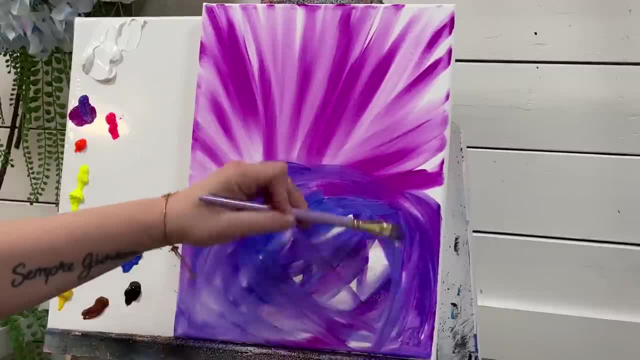 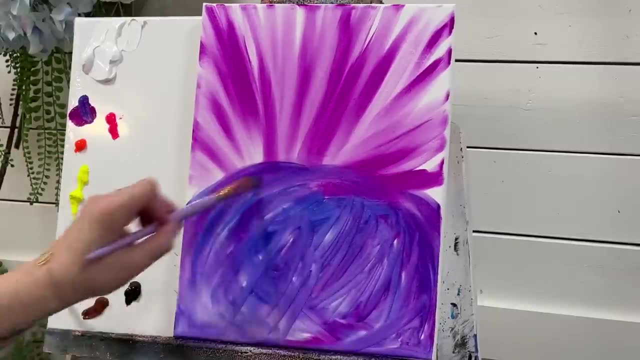 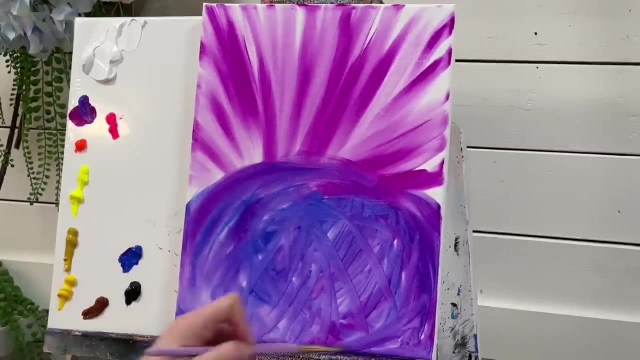 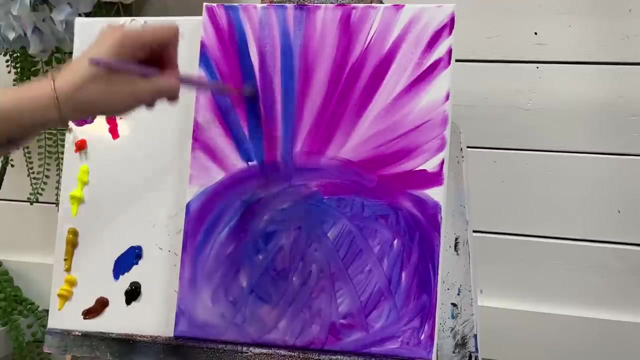 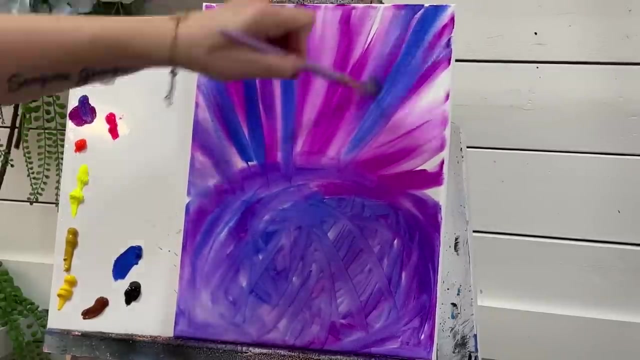 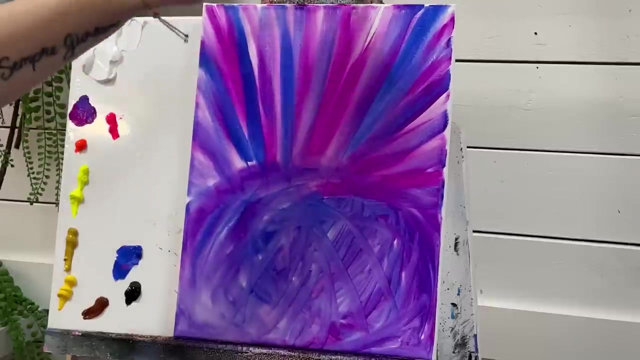 make that the backdrop and make the bumblebee in more details and make it the focus of our painting. I'm going to come in and add a little bit of the blue now, A little bit more of that beautiful violet. So because I'm going to be using a lot of orange and yellow in this flower, 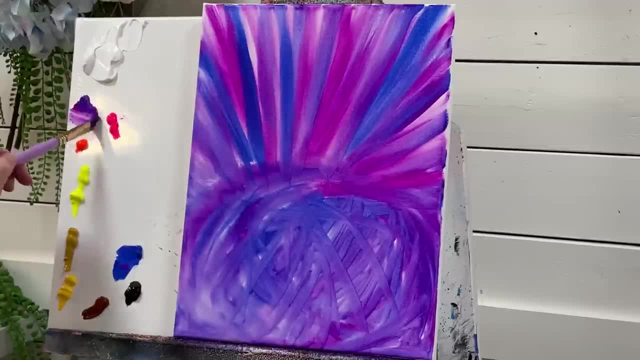 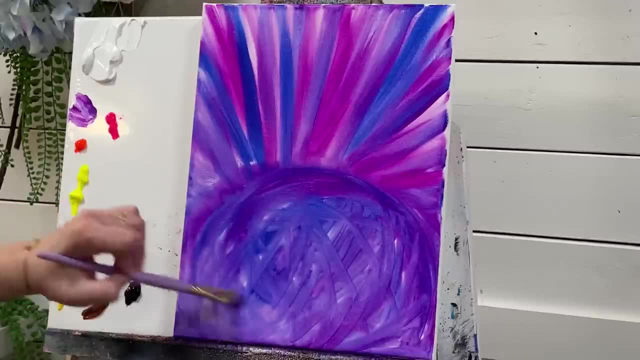 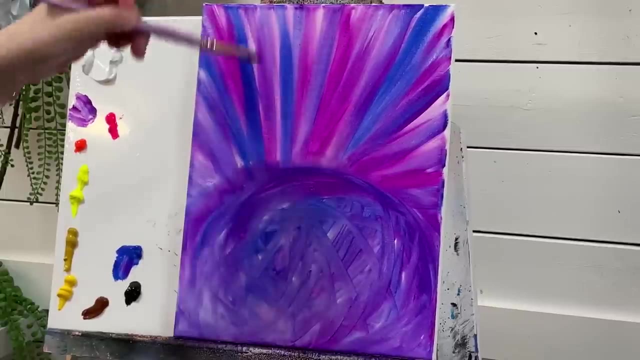 it's nice to have some complementary colors. I want to really bring it all together and that's where the blue and the violet and all these shades of purple that we're creating will really help to set off and complement all the orange and peach and yellow. And if you're not sure about what complementary colors are and what goes together, 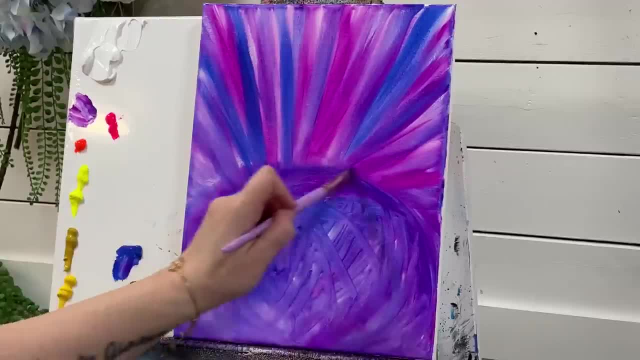 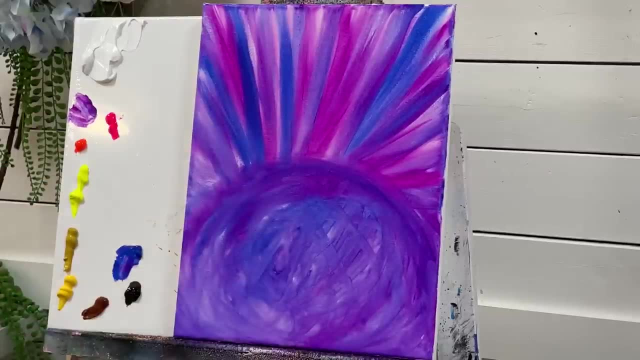 you can just google a color wheel online Or purchase them inexpensively at art stores or online as well. I'm going to dry this layer off and then I'm going to start coming in with a little bit of burnt sienna and some of my yellow ochre. 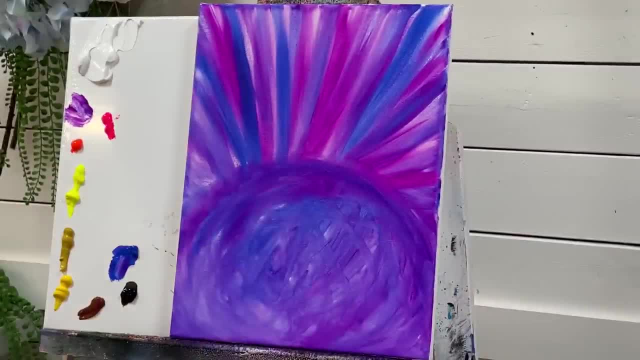 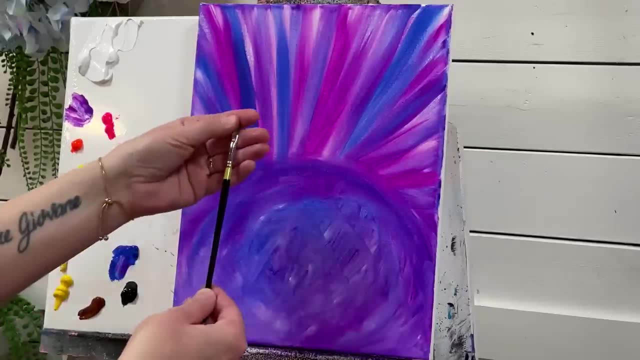 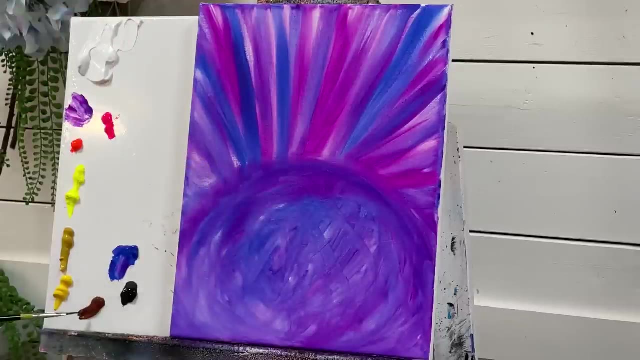 Now that this is all dried off, we're going to start coming in with the next colors, and I'm going to be using my dagger brush. I'm going to get it a little bit wet And I'm going to take some burnt sienna and a little bit of yellow ochre. 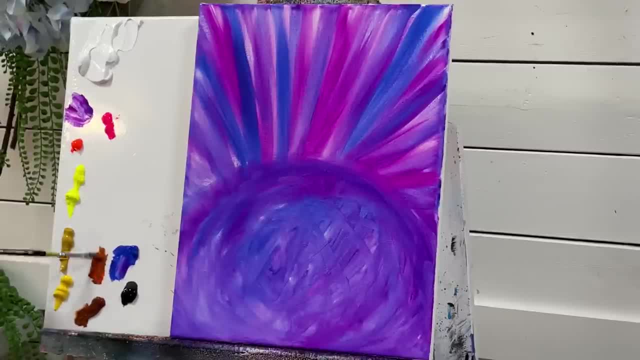 Take a little bit of orange as well, Maybe a little bit of pink too. It's all about having fun with color. today I'm just going to come around. I'm going to do it in circles And then take the little beads on the warning of the circle here. 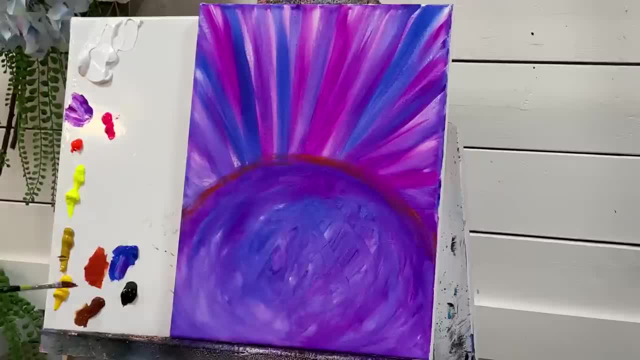 This is the center of the flower. Take those colors again. It's so easy to draw this in. It's really a long way to go. It's a long way to go. It's a small piece and I just can't do it all at once. 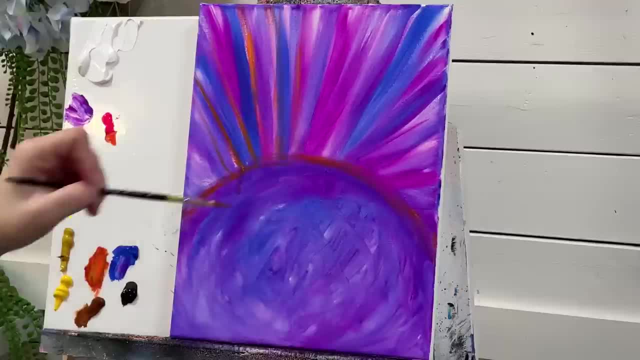 And I'm going to take some of these. I'm going to put this in my palette and then I'm just going to line them out. I'm going to like my pad, I'm going to use the look of this look. I'm just going to get my palette and just take the two of them and set them aside. 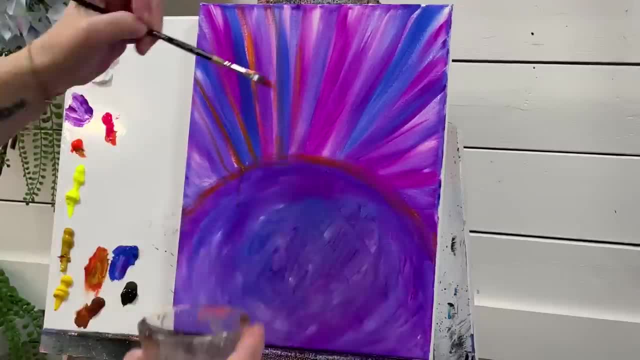 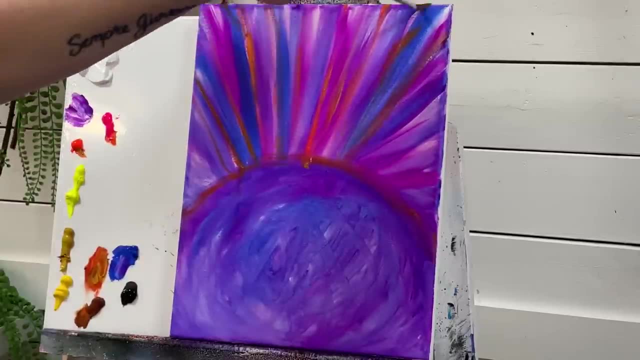 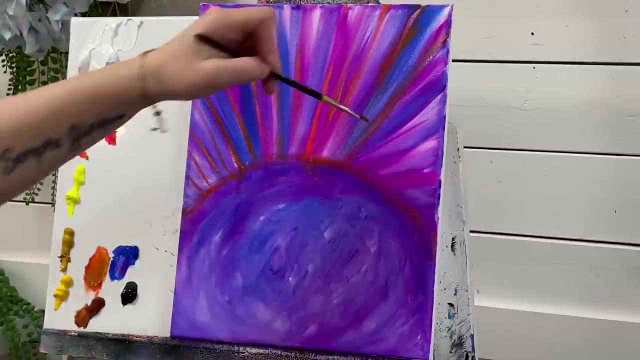 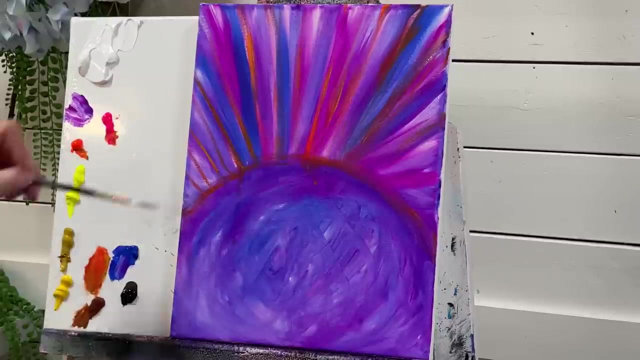 And then I'm going to go ahead and enlarge it. I'm just going to go ahead and put it in my palette And then I'm going to take a little bit of red. We're going to go in between the petals, so really just adding some lines here. 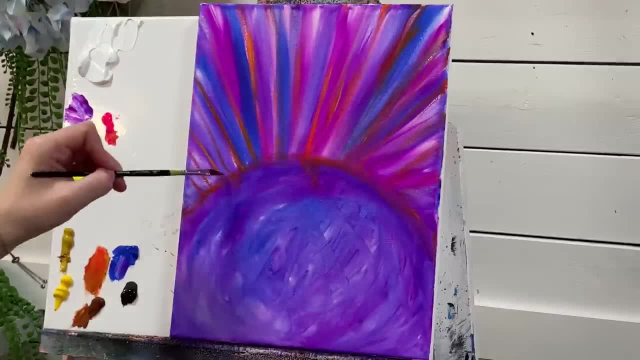 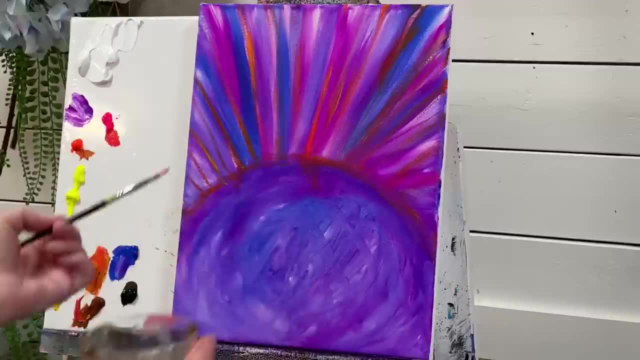 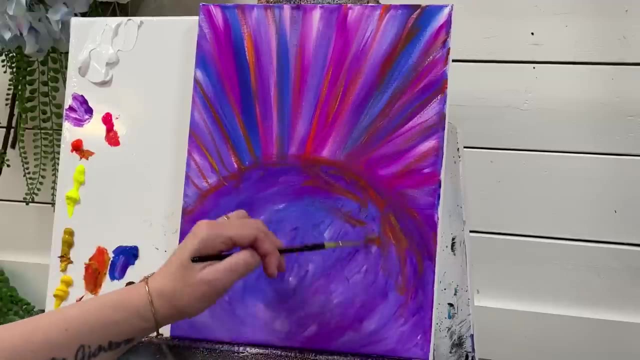 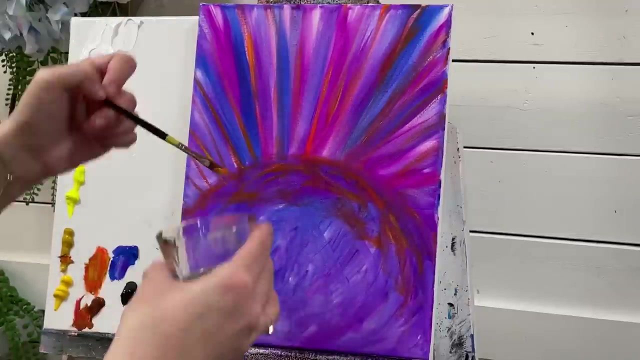 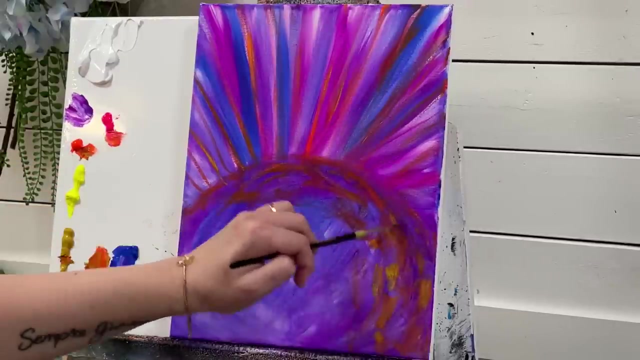 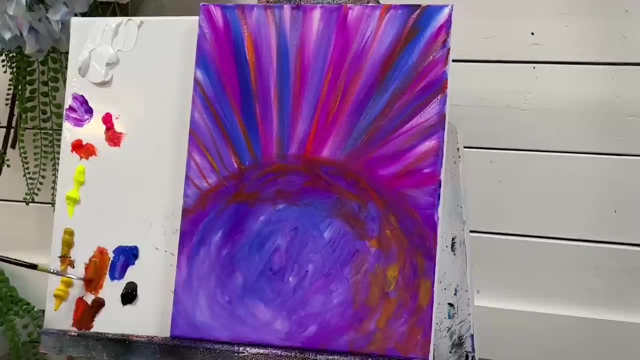 Okay, let's take those colors again. a little bit of water, and I'm just loosely brushing over Sort of flat with my brush. Okay, This is so. we can not completely cover up all the colors that we have underneath and it gives it more of a looser, abstract feel. 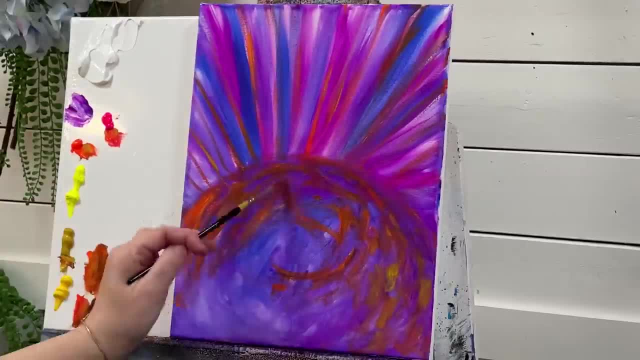 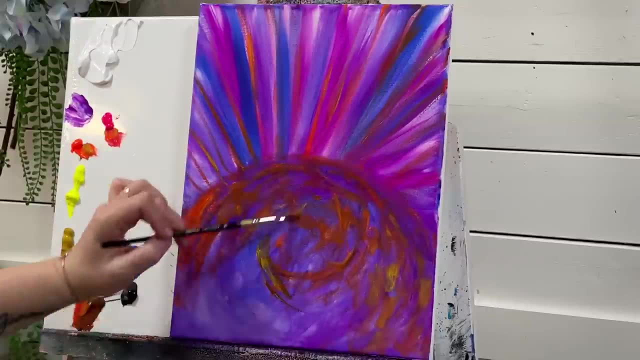 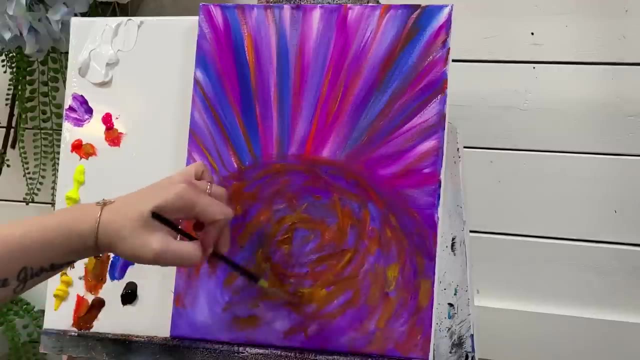 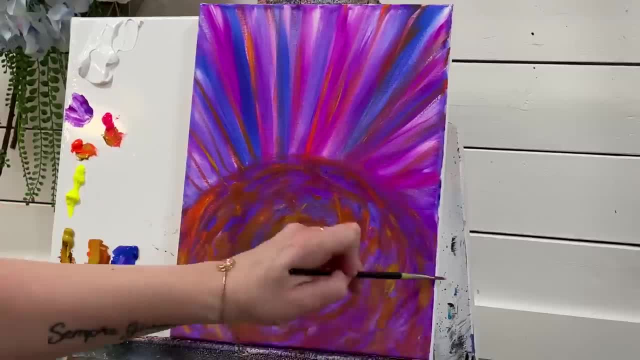 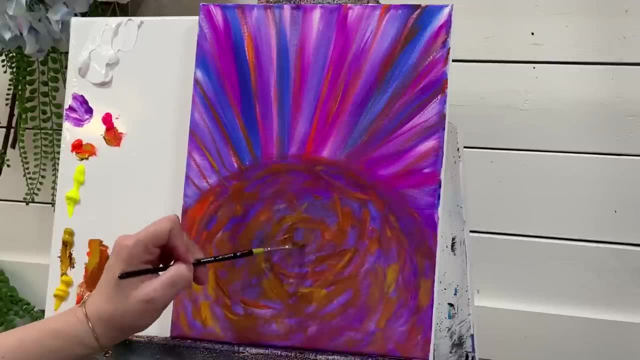 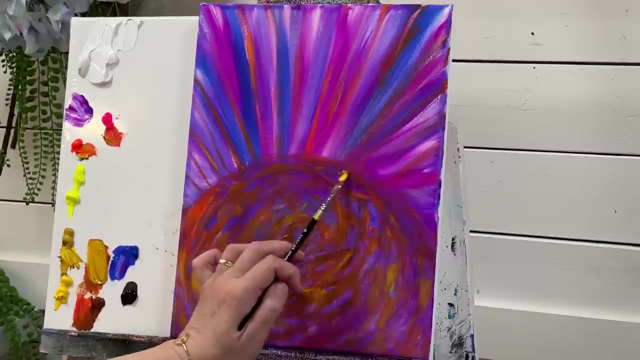 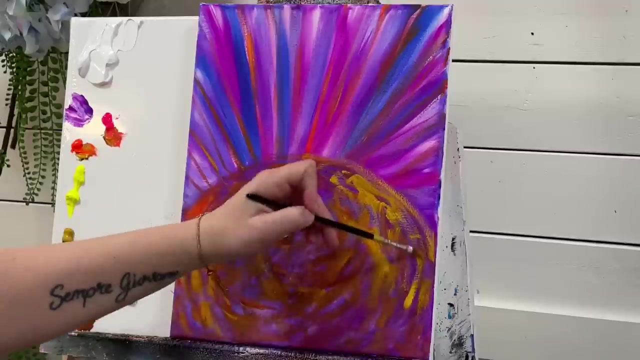 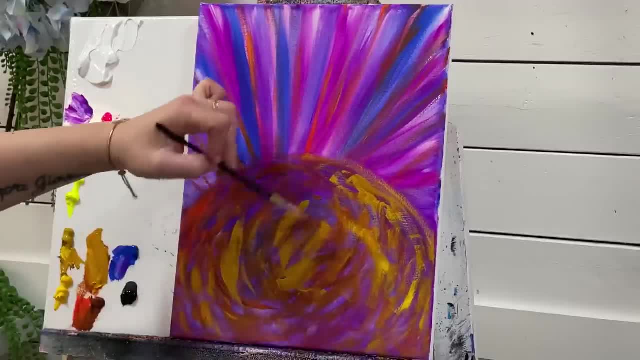 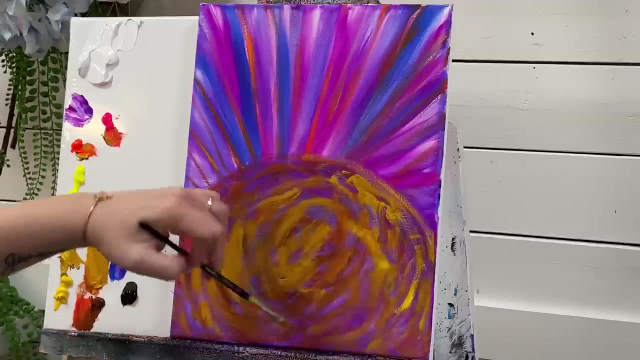 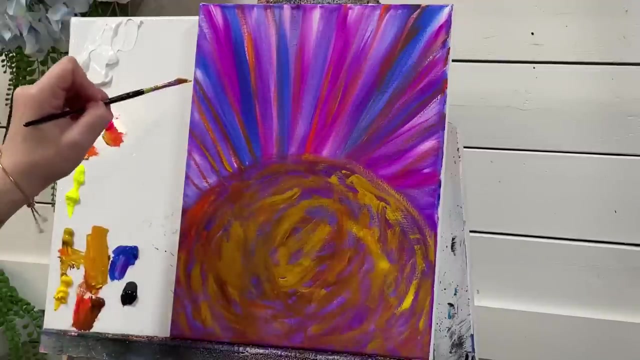 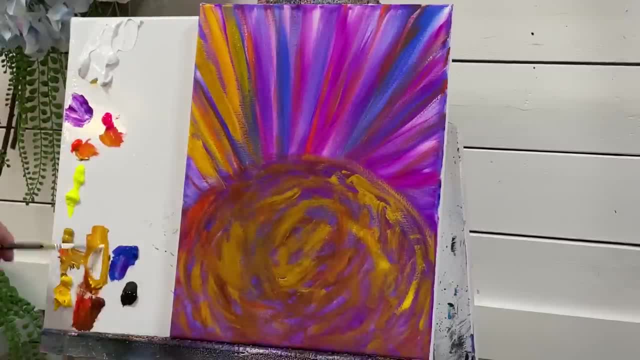 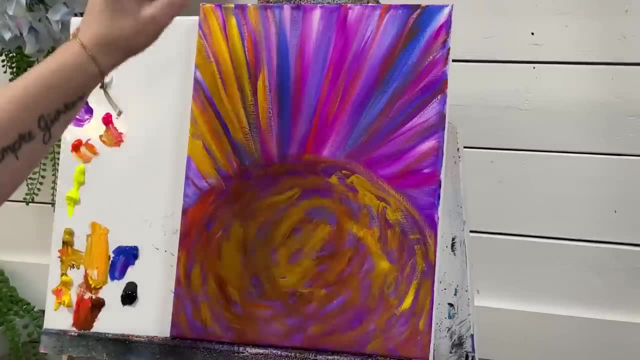 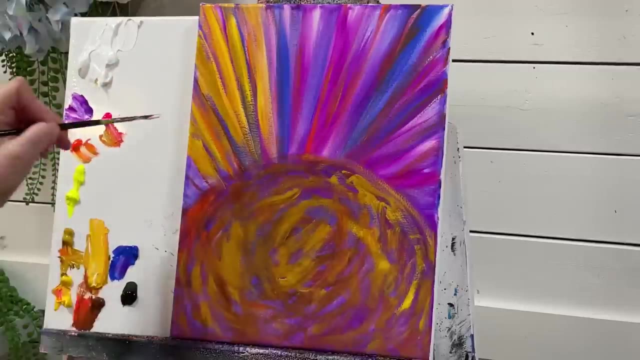 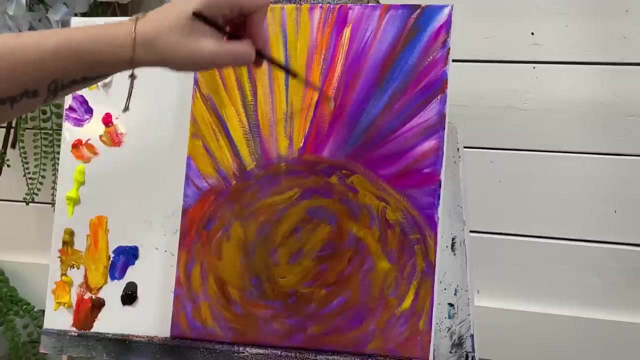 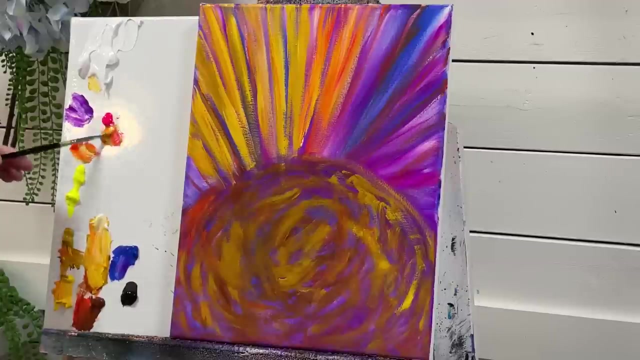 And we'll just start adding a little bit of white as well and pull in a few lines, So I'm never making just one solid color. This way you get so many different shades. Just a little bit of pink and yellow here over the blue. 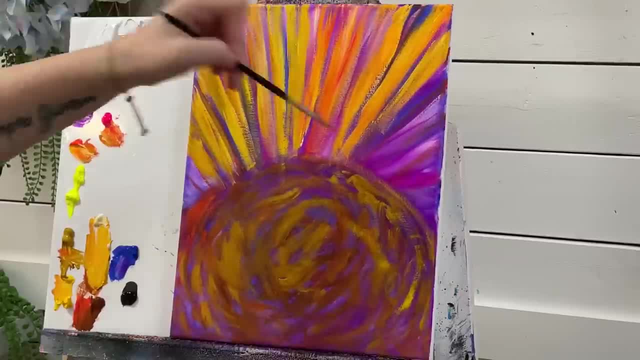 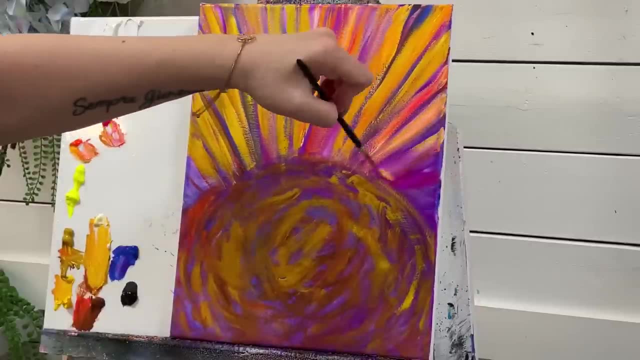 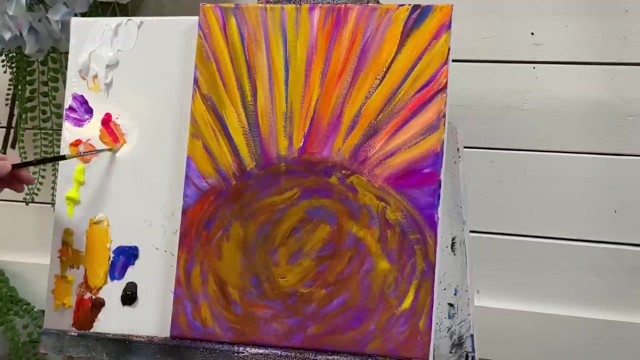 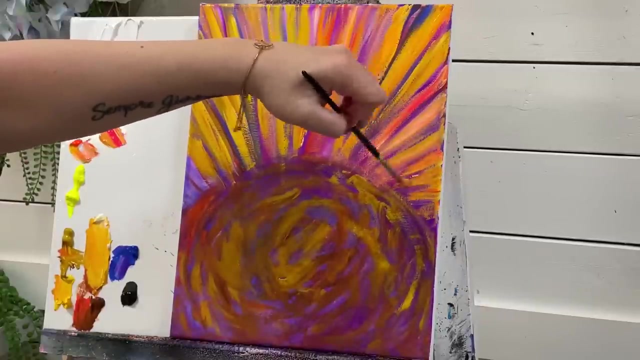 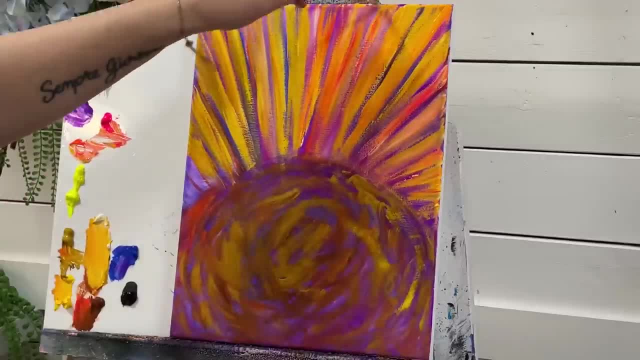 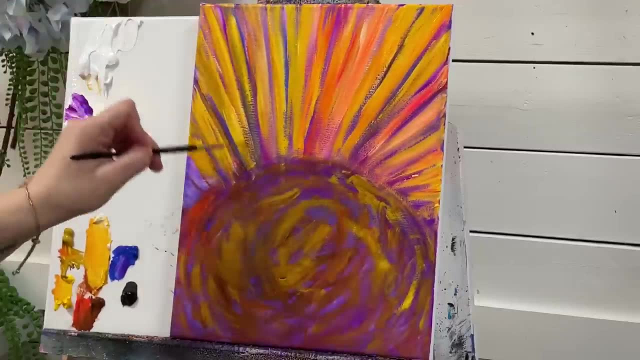 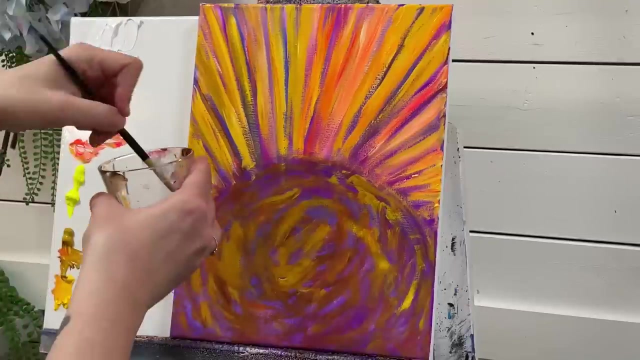 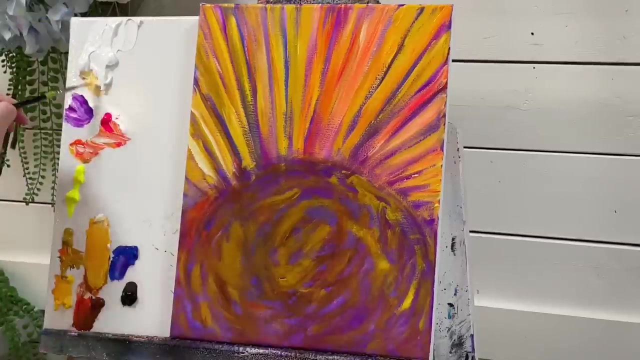 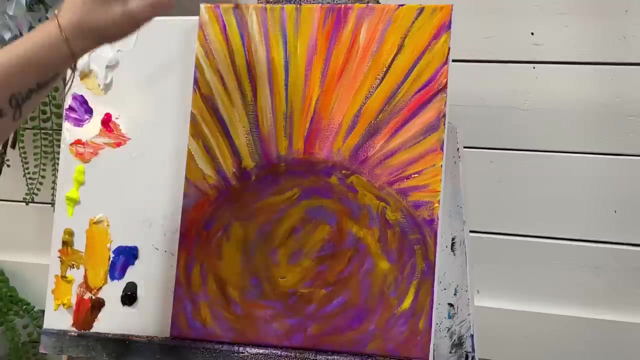 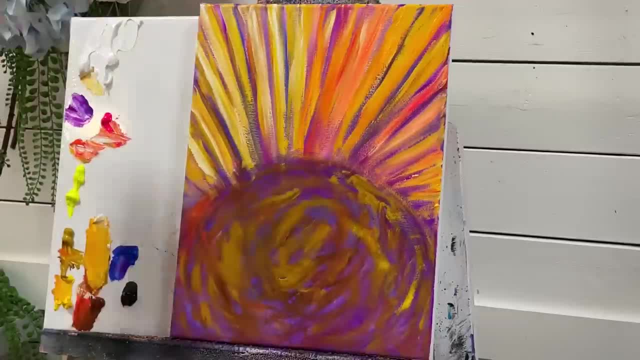 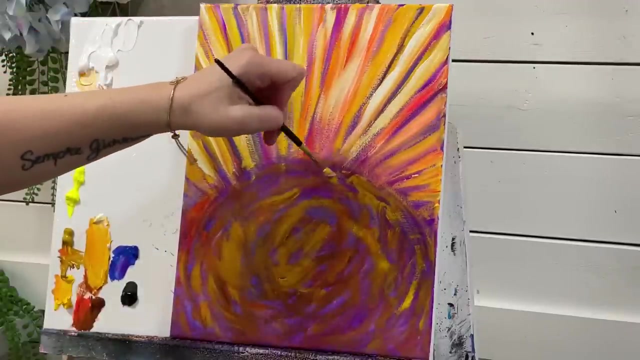 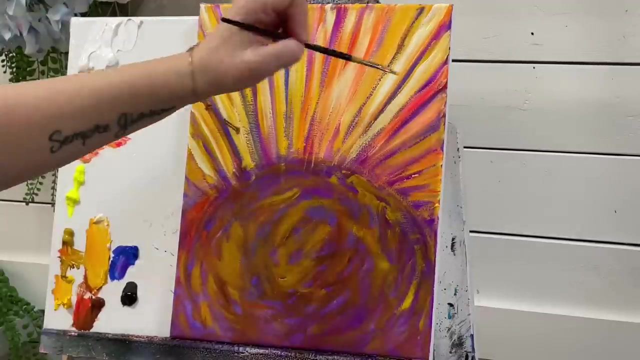 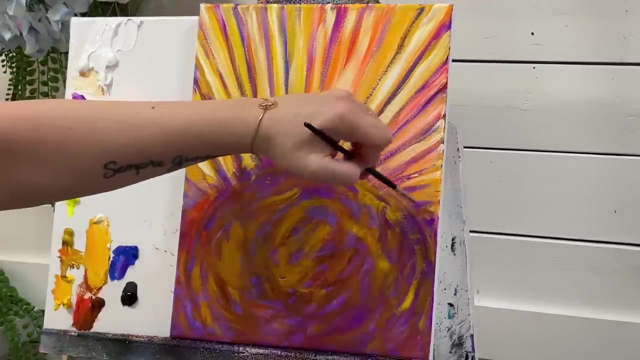 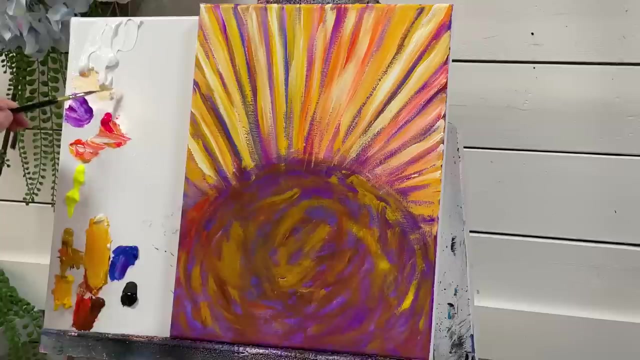 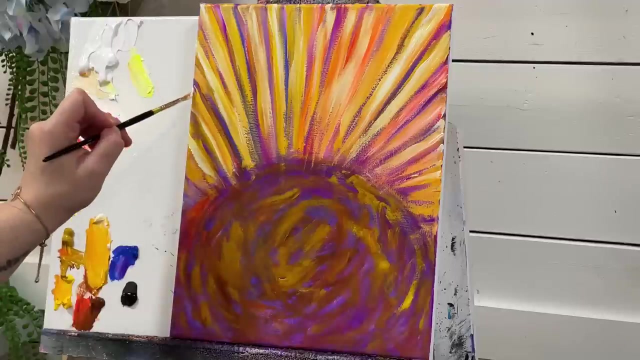 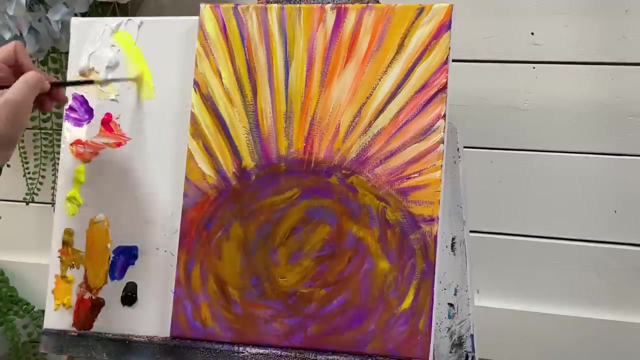 so we can make some softer shades. It's really important to add this white if you don't want your painting to dry too dark. Okay, now I'm going to take a little bit of my lemon yellow with white and add a little bit of this. 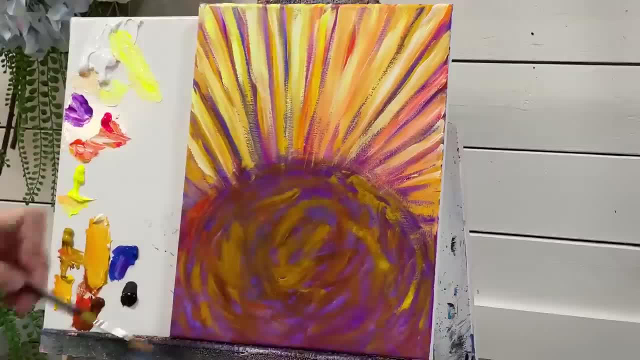 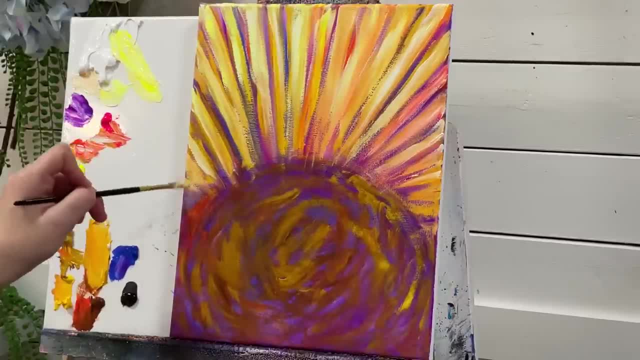 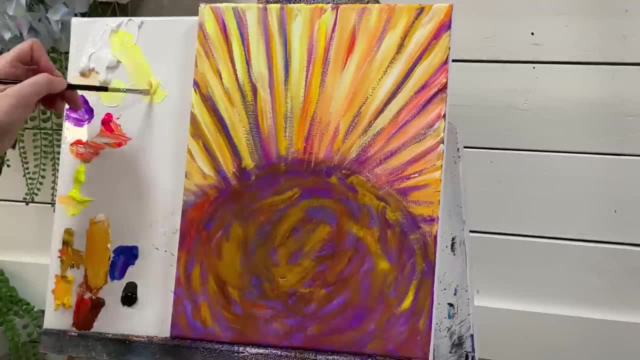 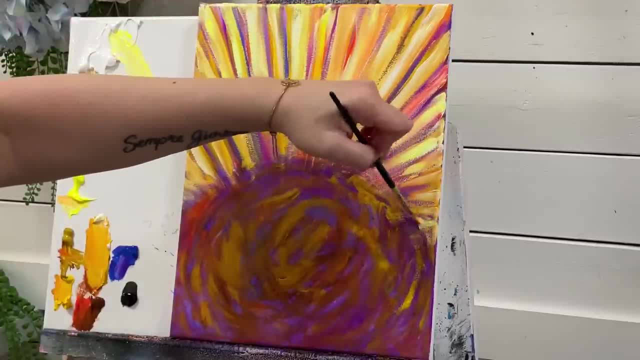 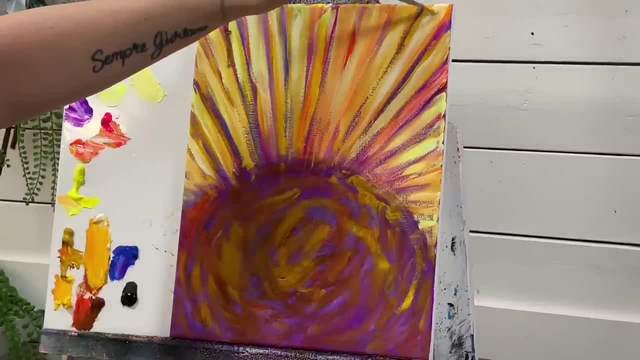 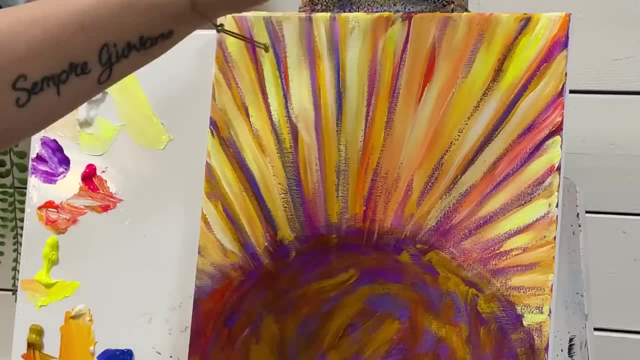 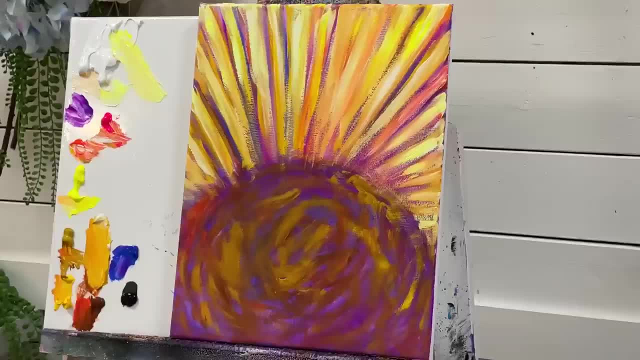 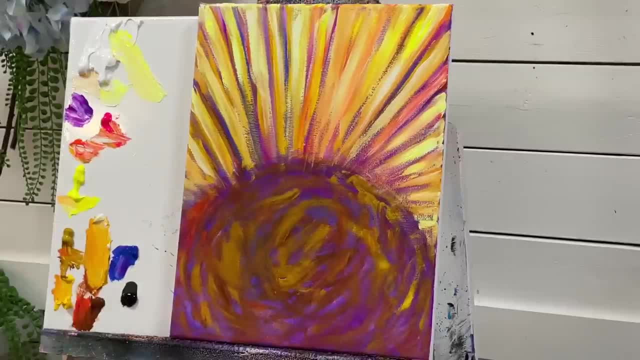 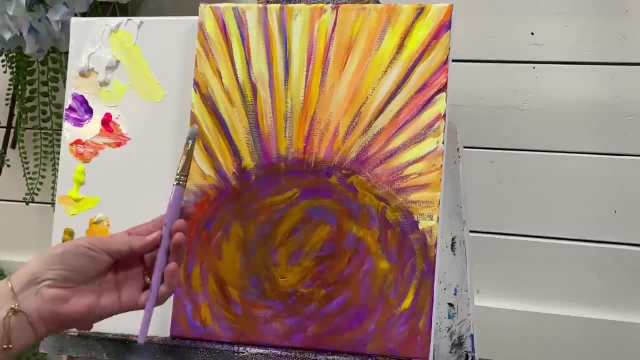 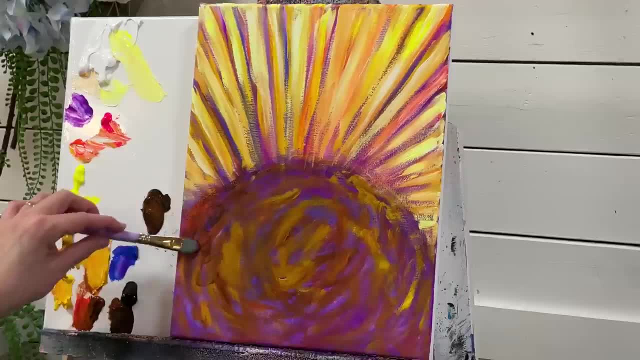 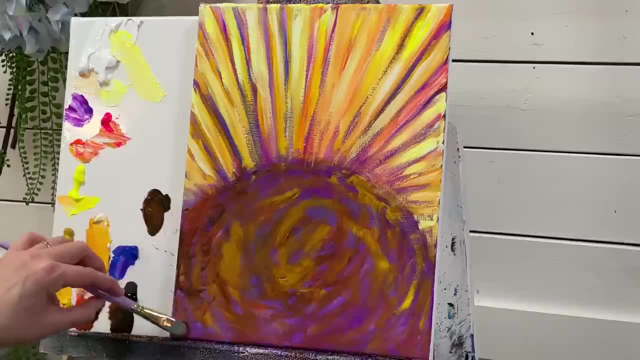 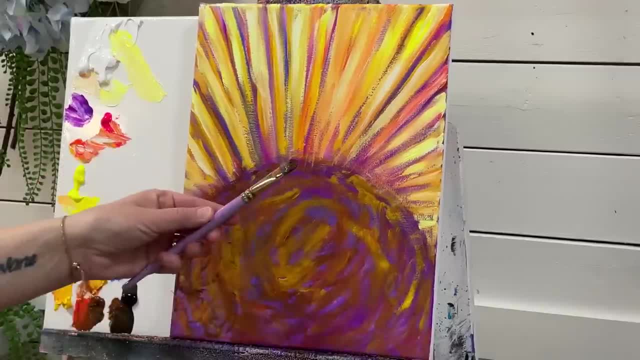 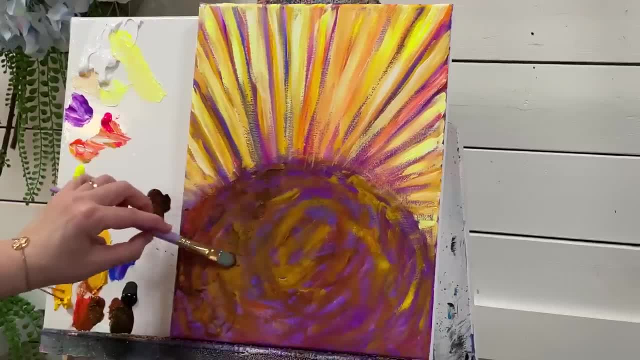 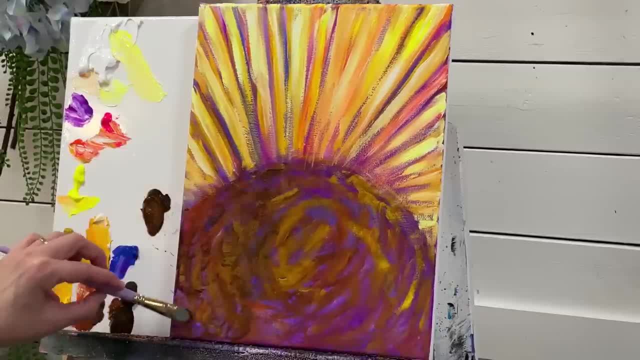 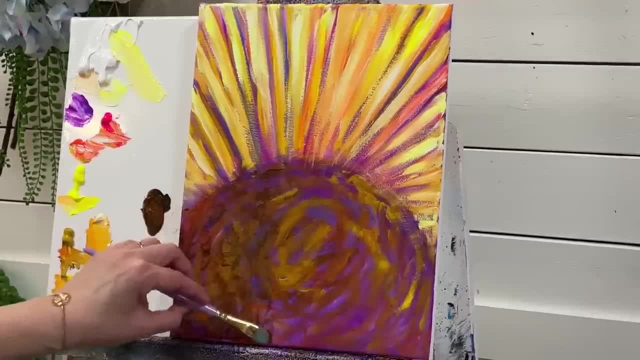 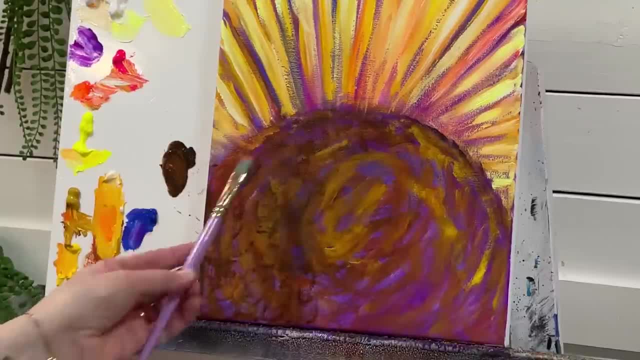 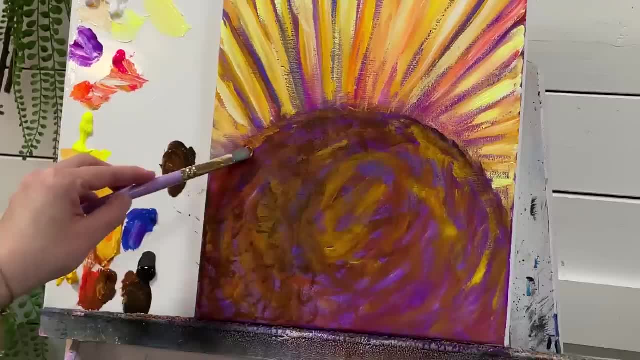 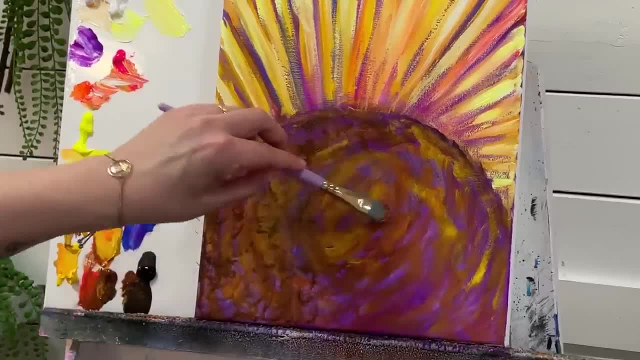 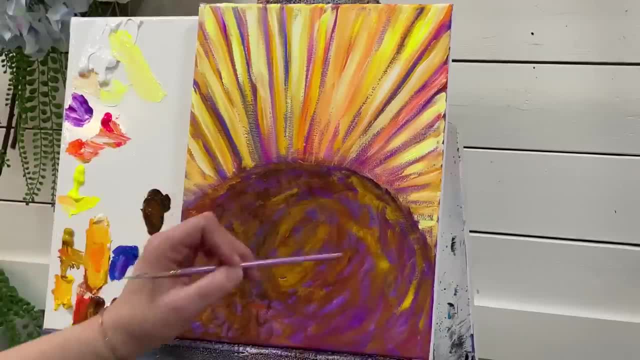 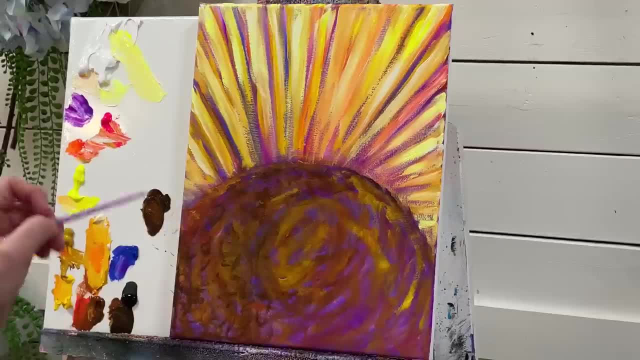 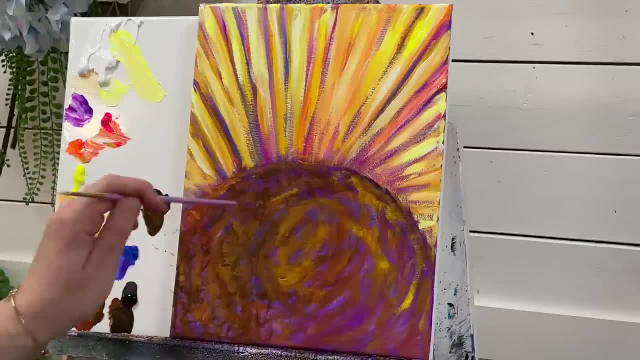 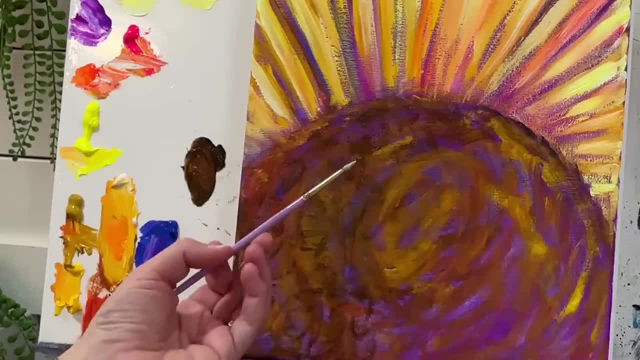 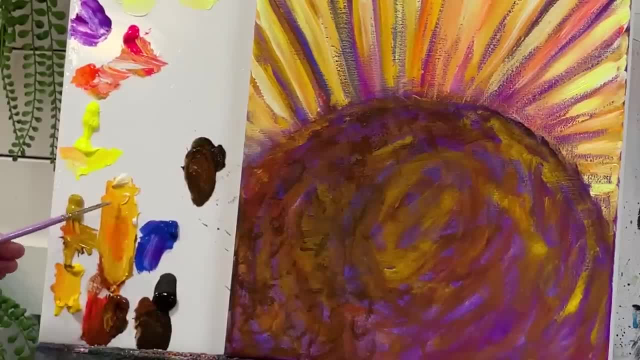 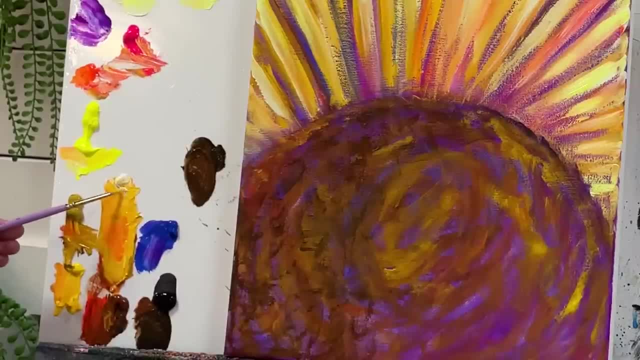 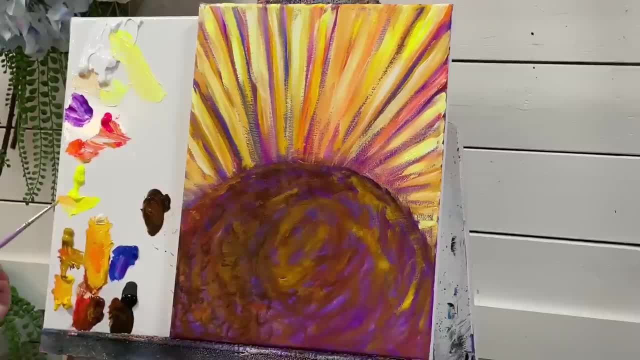 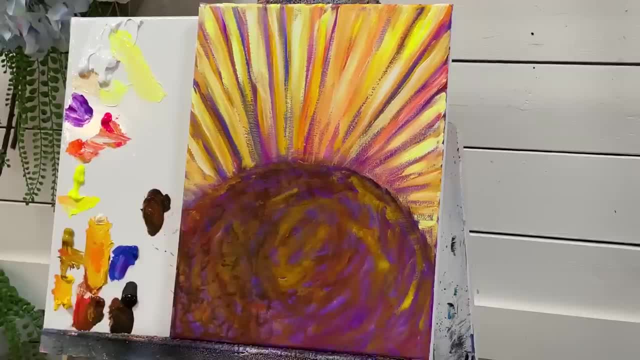 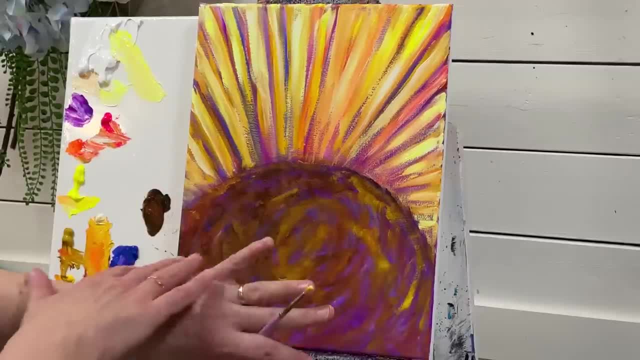 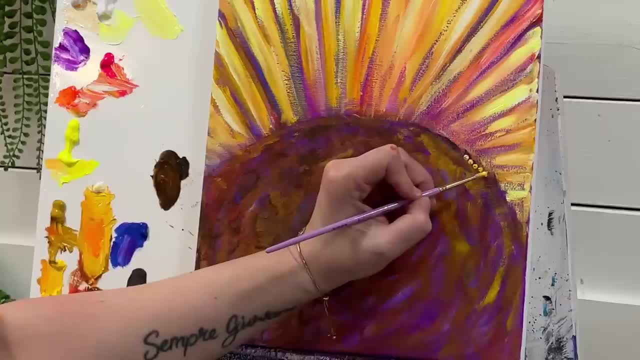 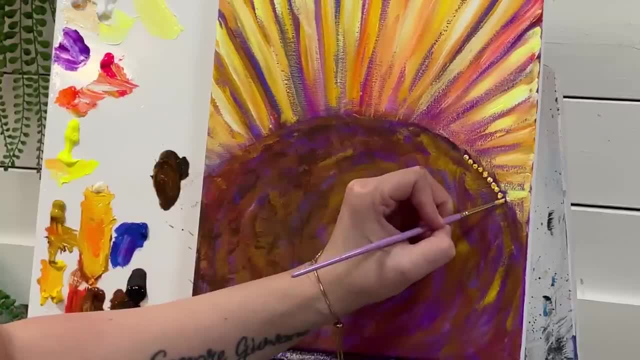 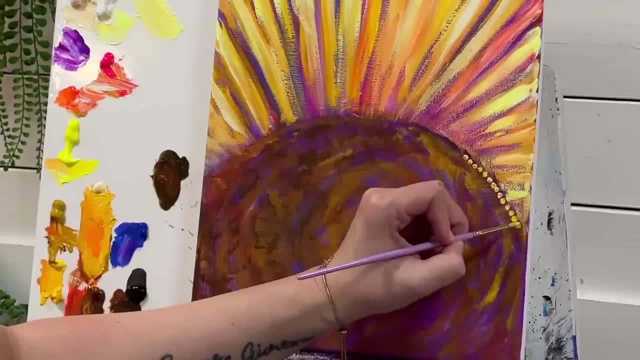 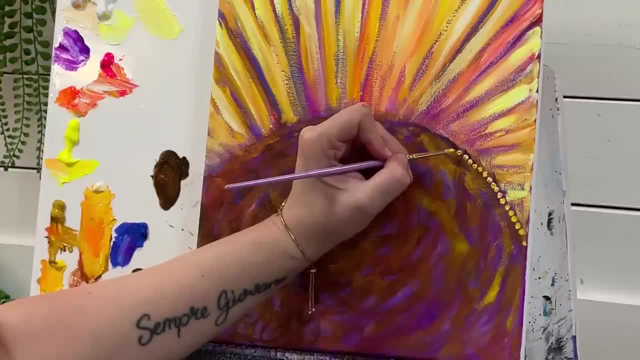 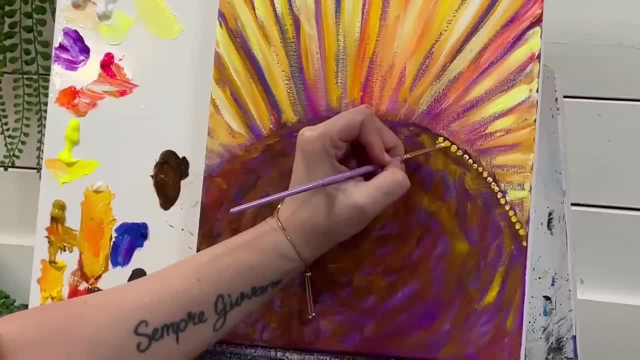 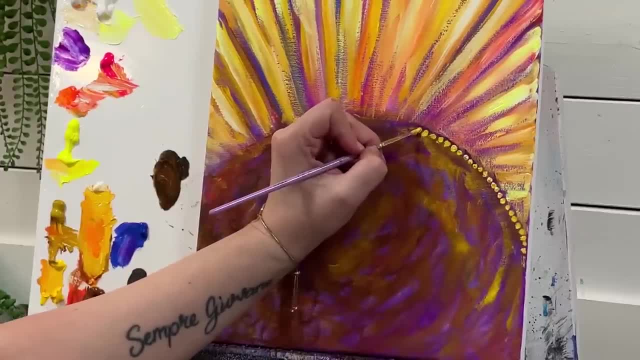 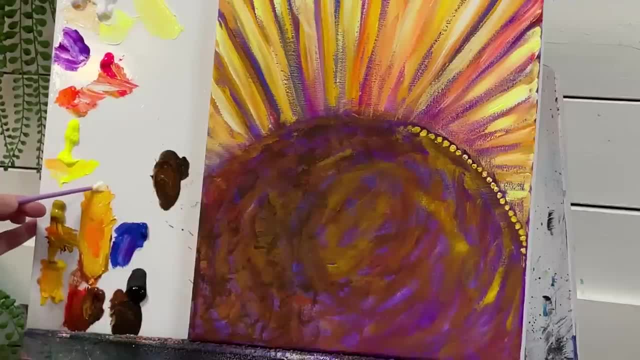 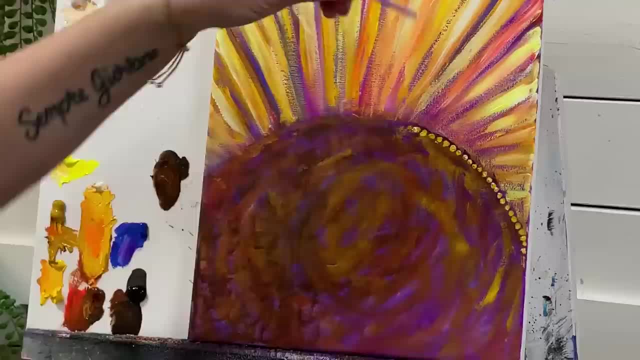 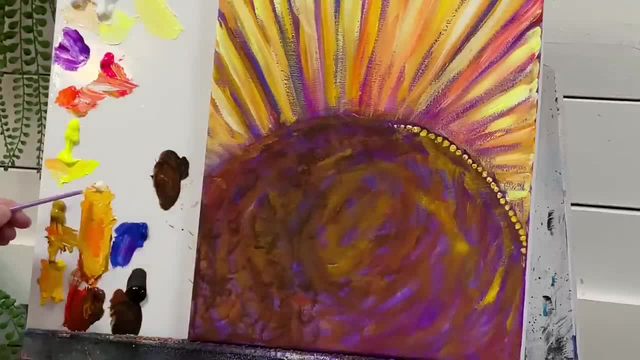 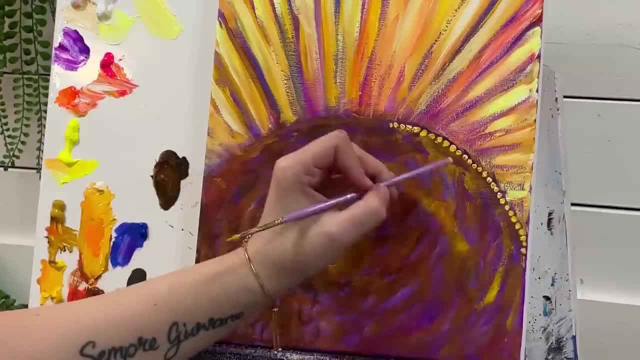 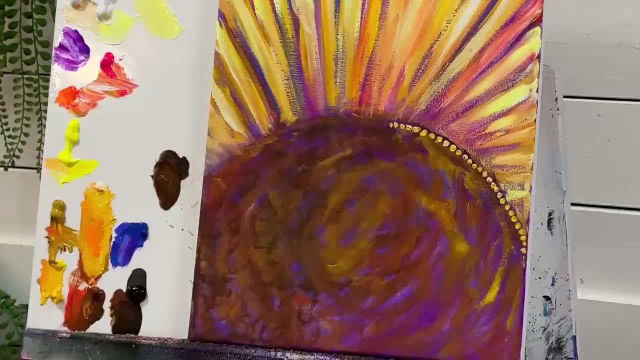 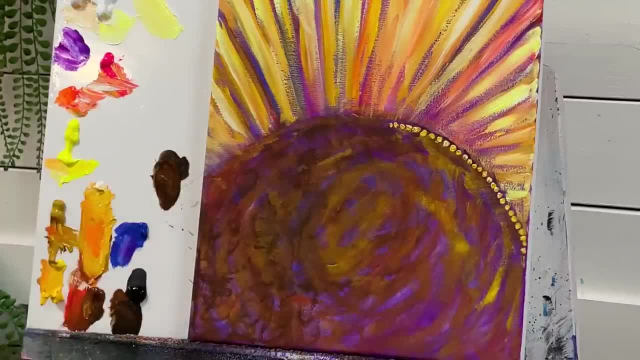 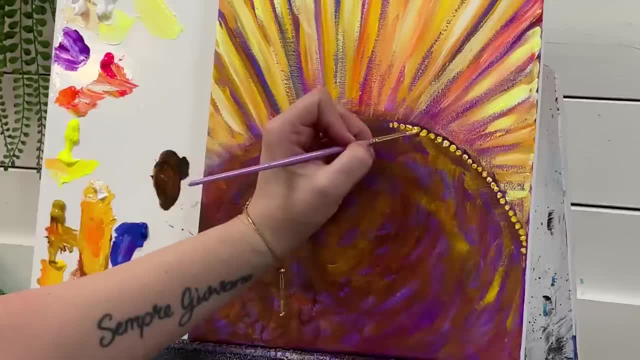 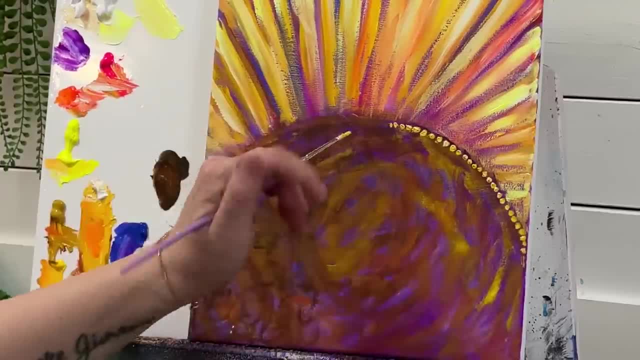 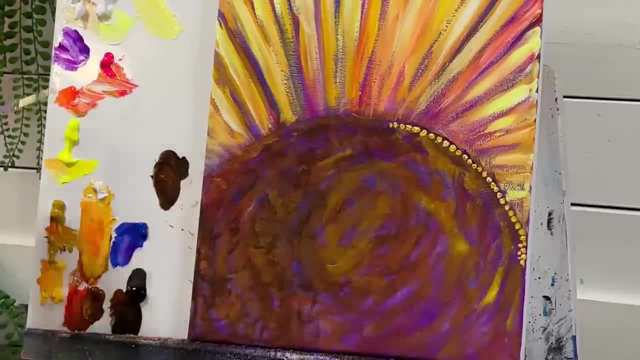 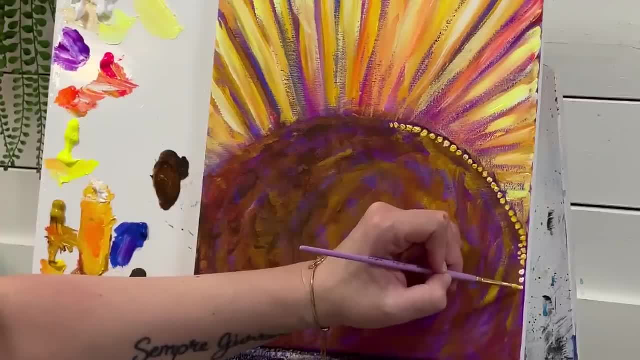 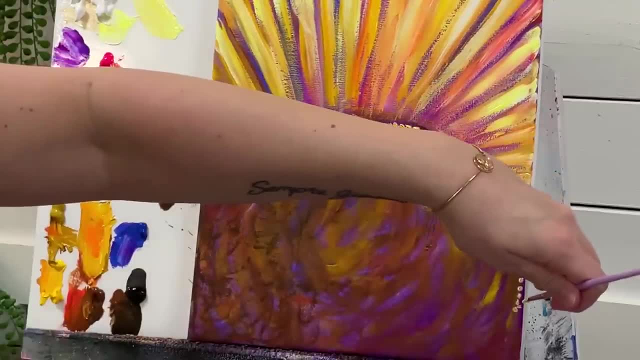 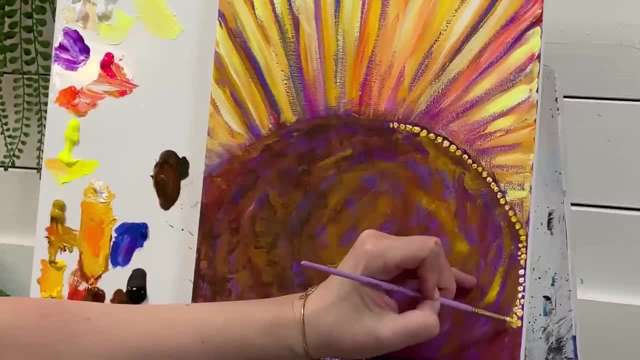 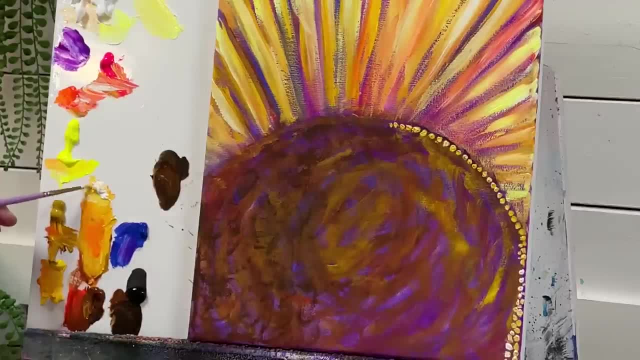 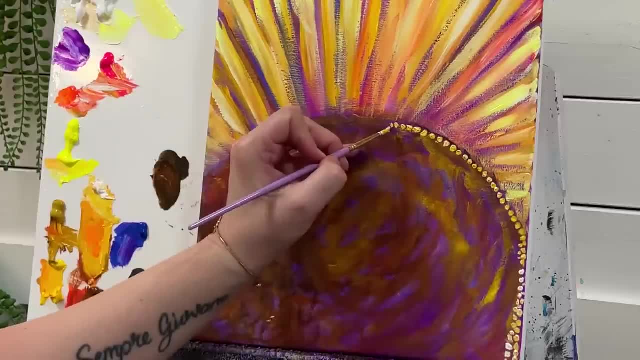 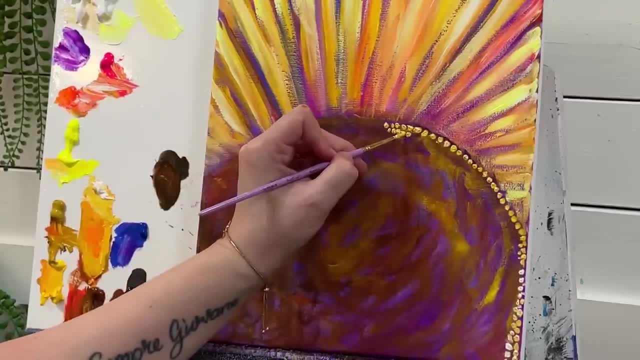 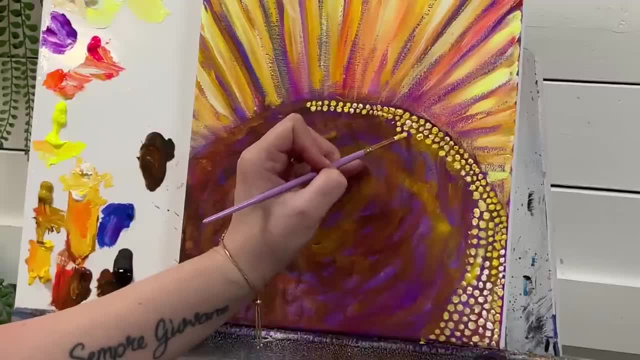 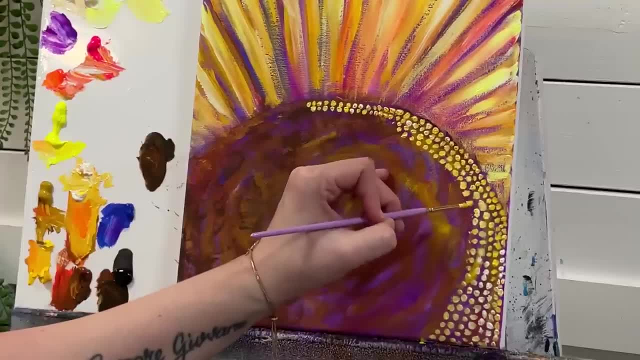 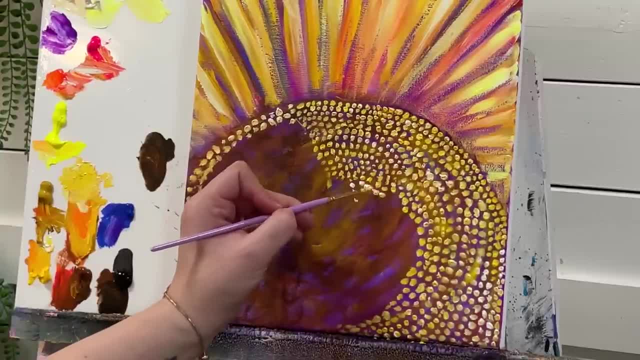 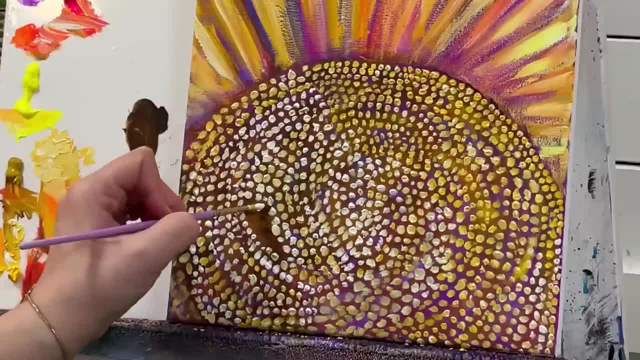 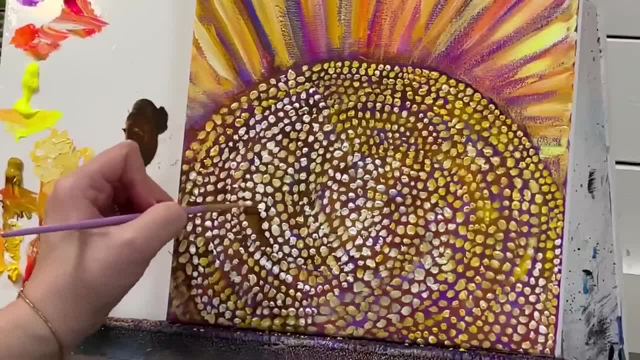 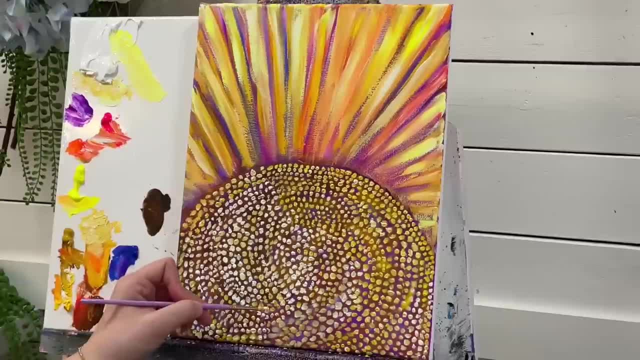 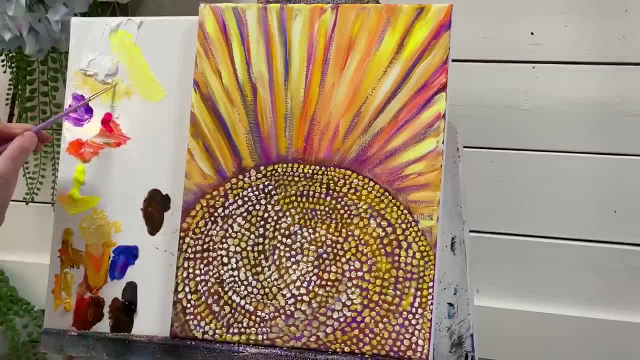 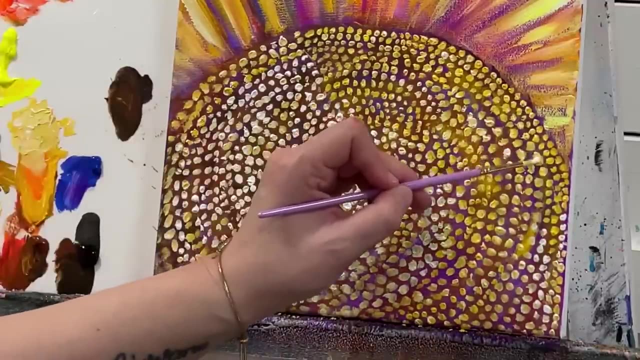 Okay, so I've just finished up the dabs and the dots here, or the little seeds inside the flower or the center of the flower, And I'm just going to go back and add a little bit more white to some of them before I completely dry this off. 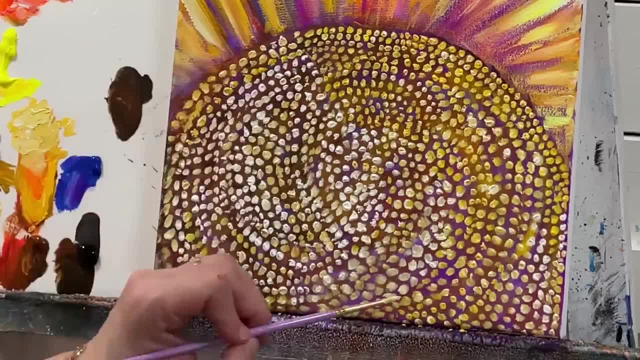 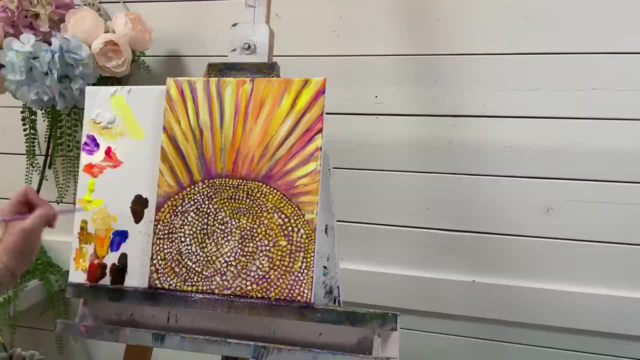 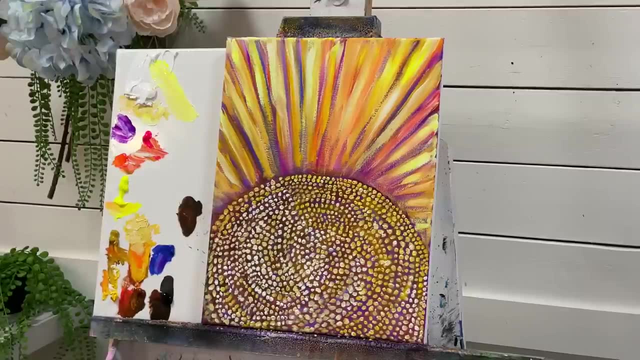 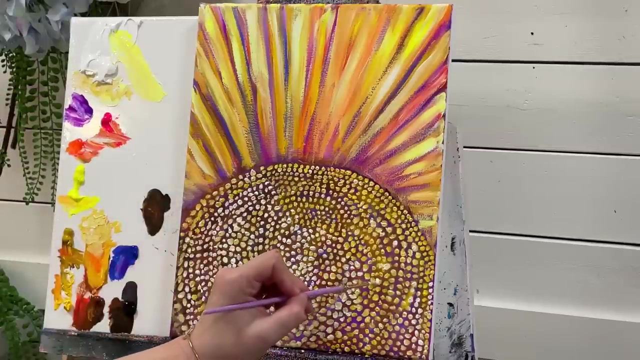 And then I'm going to show you how we're going to glaze over, once it's all dry, with some colors. We're going to use some of the orange pink and the navy blue, And then we're going to use some of the orange, pink and the navy blue. 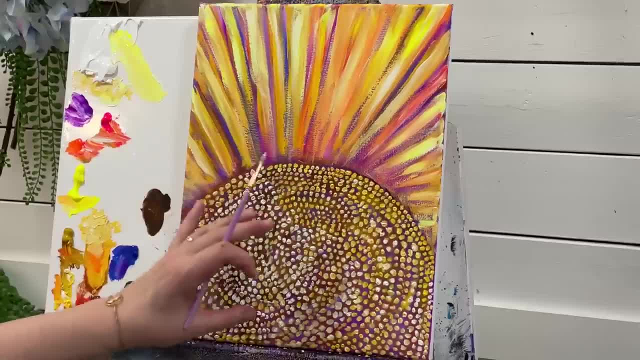 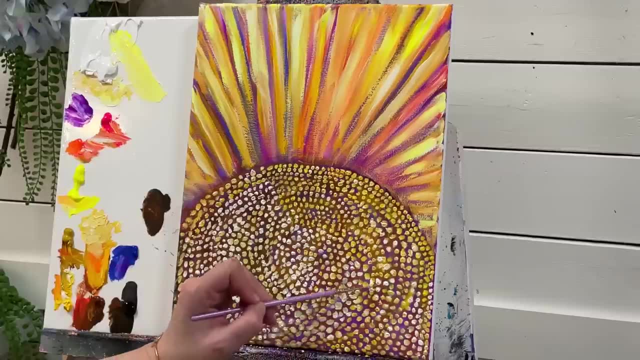 Now, even though we're going to have our bee cover up some of this, I still wanted to add all the dots because I'm not really sure where our bee is going to be, where our bee is going to be So, and I find it really relaxing. 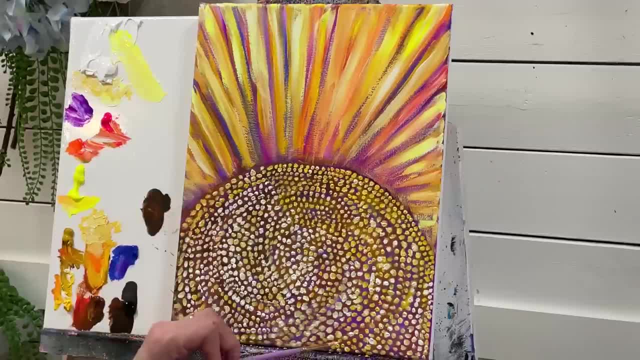 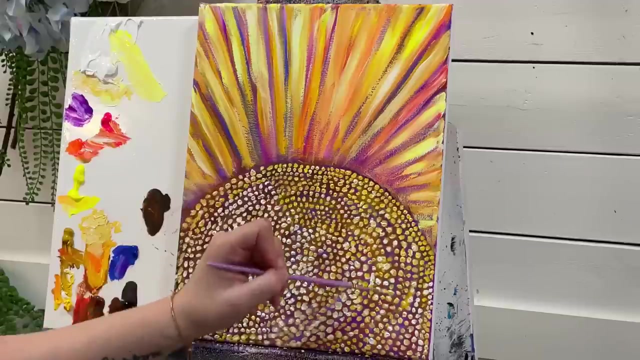 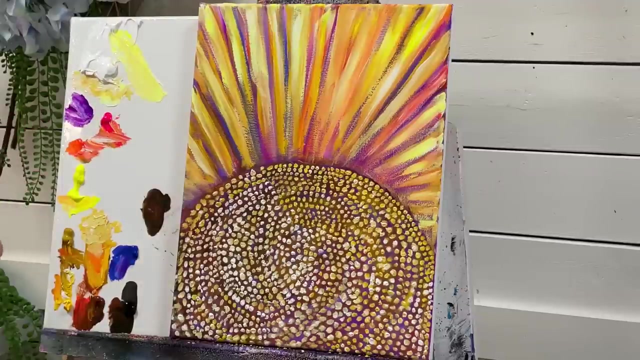 Adding all these little dots kind of forces you to slow down a little bit and calm your breathing, calm your mind. It's very meditative. Okay, so I will completely dry this off. Actually, just one more step before we dry this off. 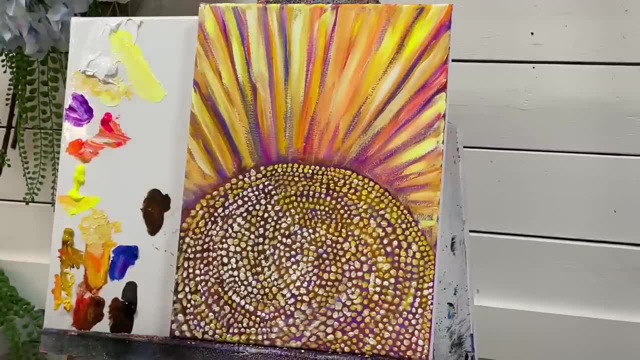 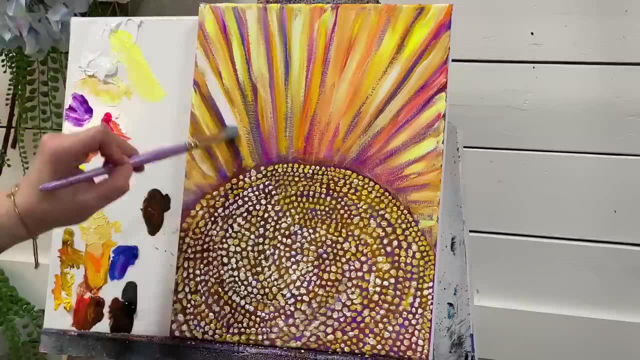 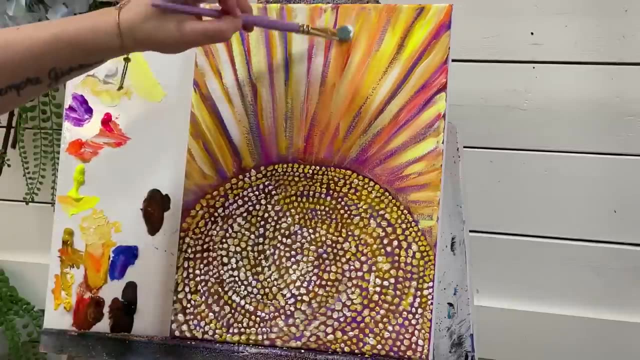 I want to come over here with a little bit more of my white as well. I'm going to use the filbert brush, I'm going to take some white and I'm just going to add it to a few areas on the petals. All those other colors will still be there. 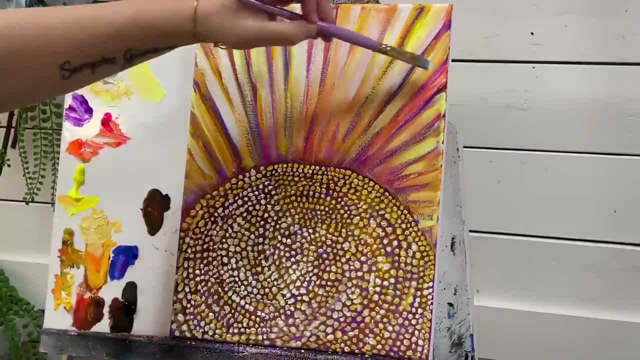 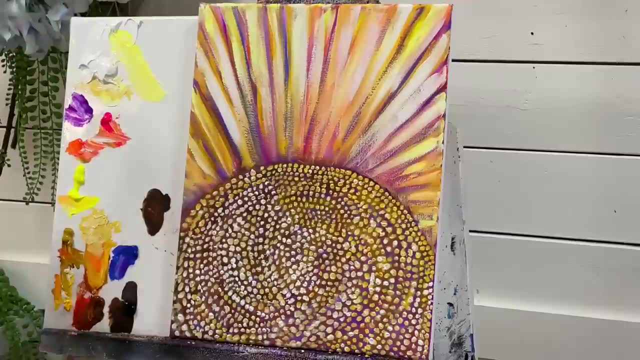 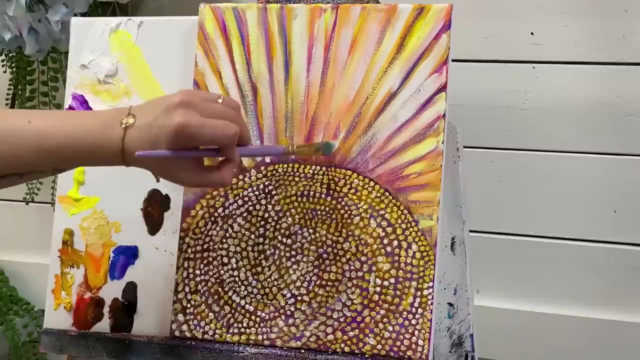 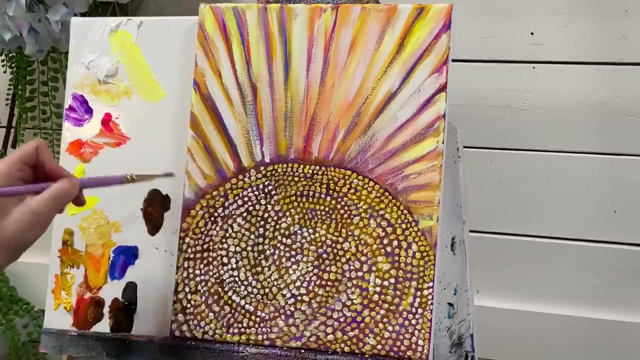 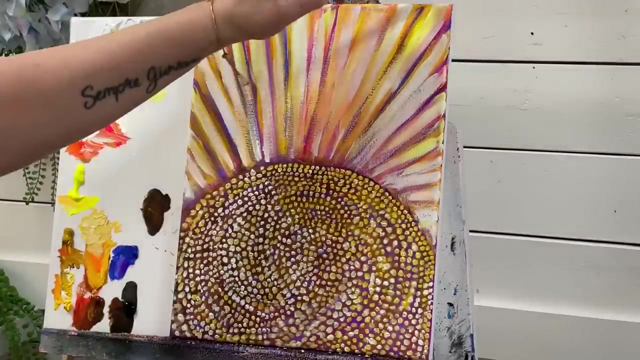 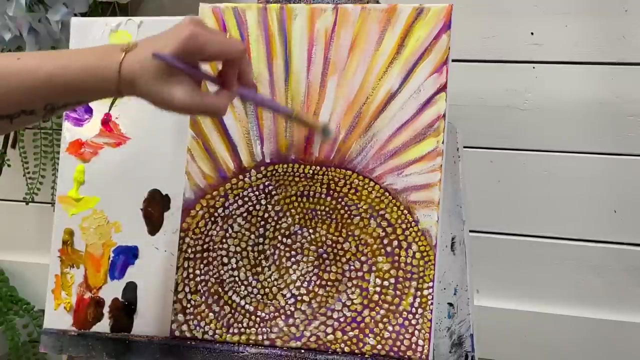 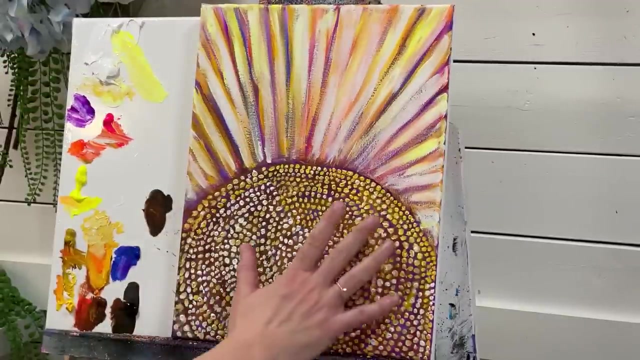 We're just going to add to them. By adding this bit of white here, we'll be able to get some nice, bright, luminous lemon yellow to really show up. Okay, so we want this part of the flower, the flower itself, to be just a little bit out of focus. 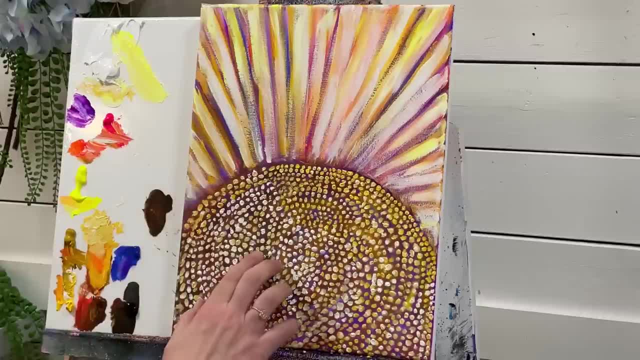 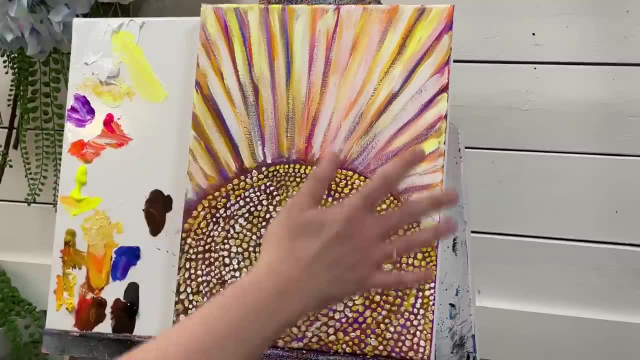 in comparison to our bumblebee. So some of these are a little bit thicker when I applied the paint and they're not 100% dry. So I'm expecting, when I come and glaze over this, to pick up some of that, But that's going to kind of make it look a little more abstract and out of focus. 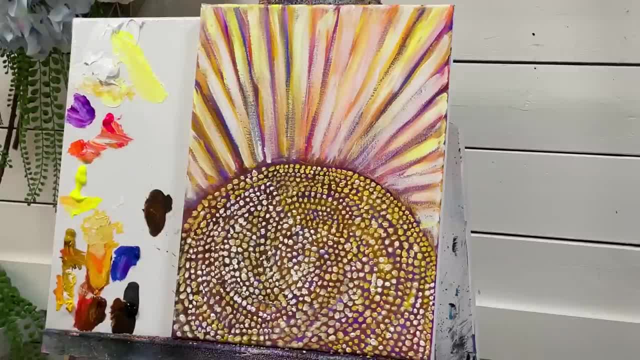 So I'm excited for this next step And I'm just going to be using my filbert brush to add the glaze over. I'm going to start with the bright lemon yellow, And my brush is just a little bit damp from rinsing it out. 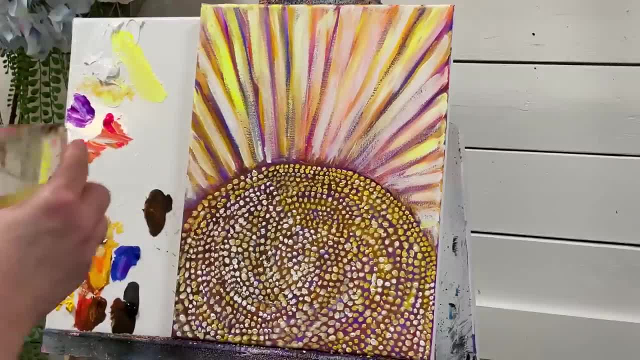 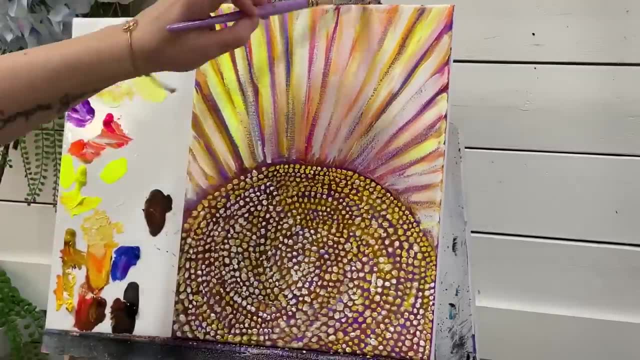 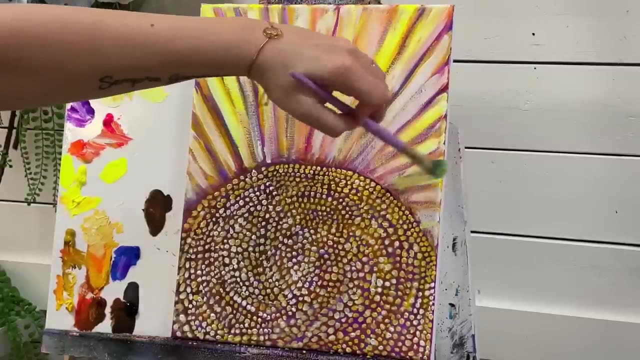 And I'm just going to come over And I might need a little bit of just a tiny bit of water in here to help release some of that out. But look at that color. So I'm going to add some yellow to a few areas. 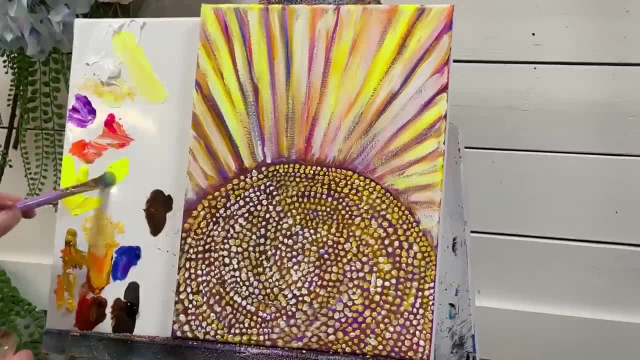 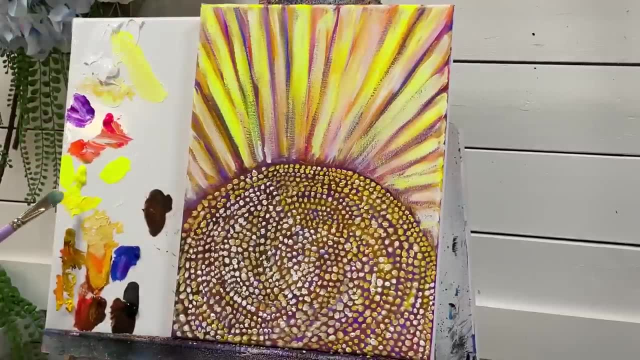 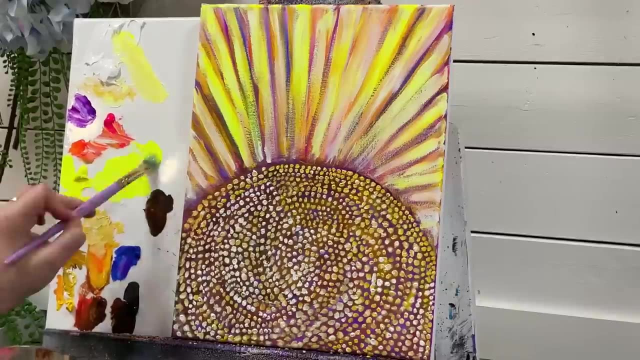 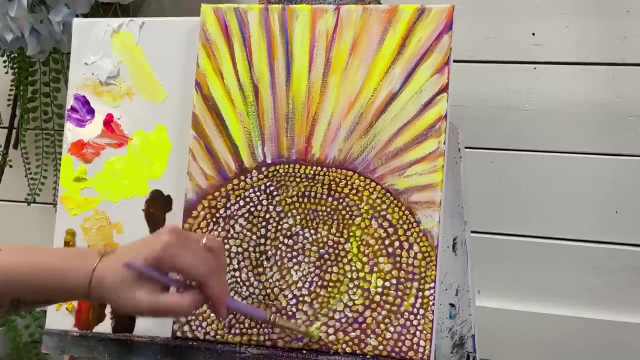 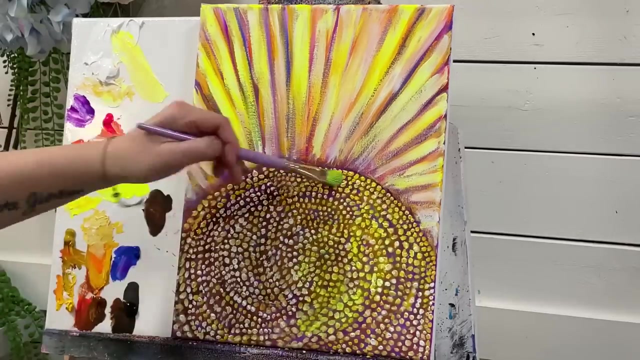 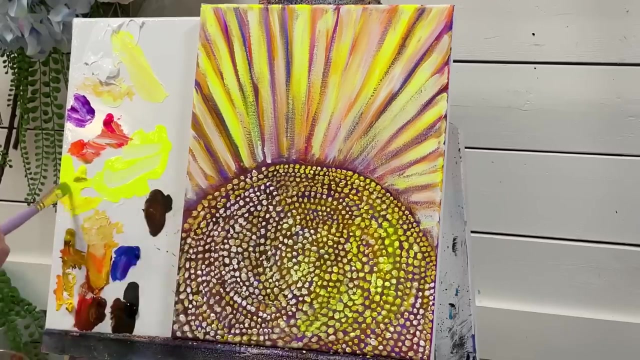 And then I'm going to come in and add a little bit of all of the colors. I'm going to take a little bit of water again with the yellow, So we're just going to very lightly, Don't press too hard. Okay, so we've got some nice yellow on there. 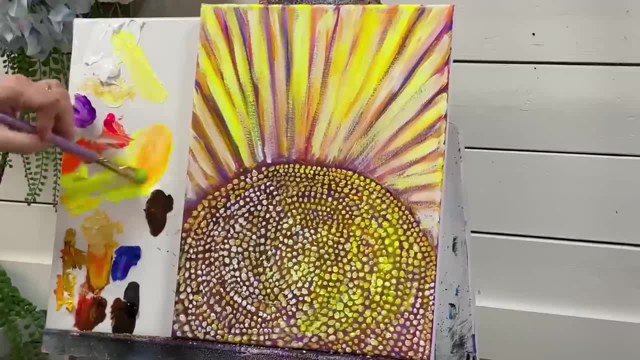 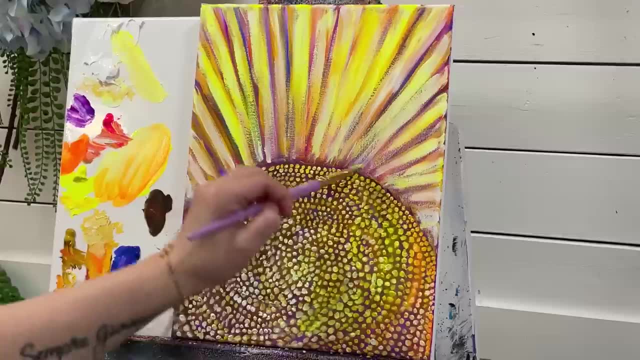 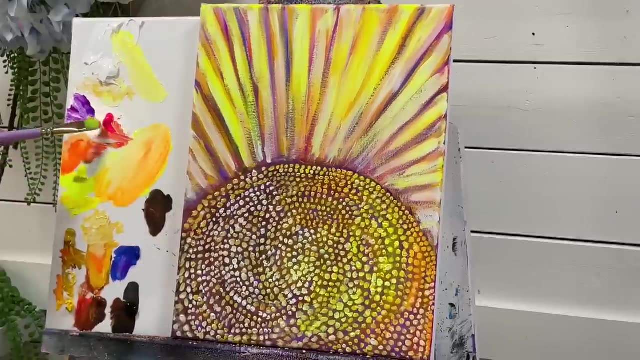 The next color I'm going to take is some orange. I'm just going to add that in with the yellow And I'm going to come around here- Look how pretty it looks with that magenta or the violet. I'm going to take a little bit of pink and yellow. 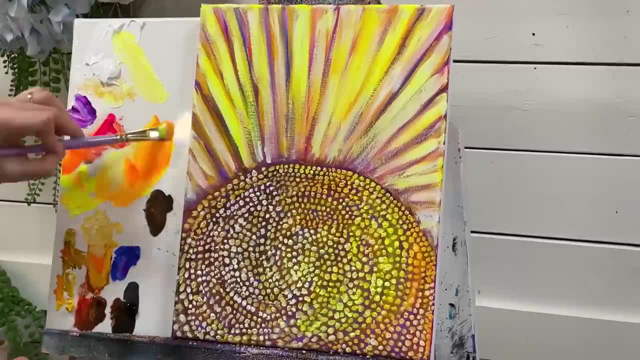 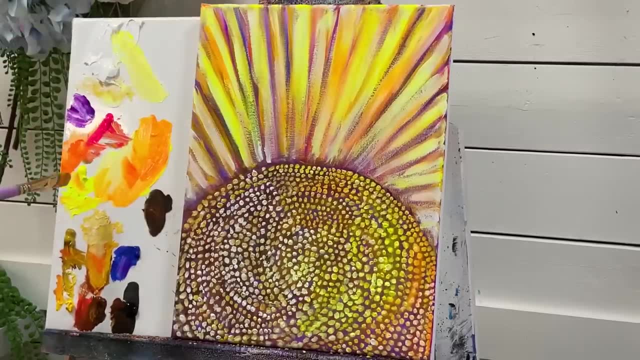 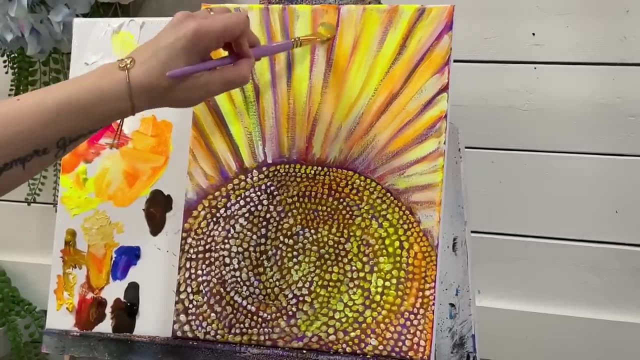 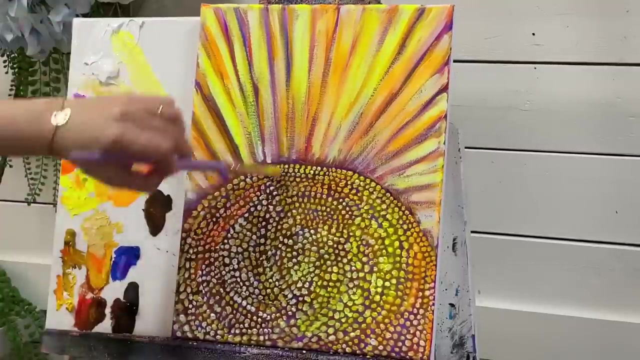 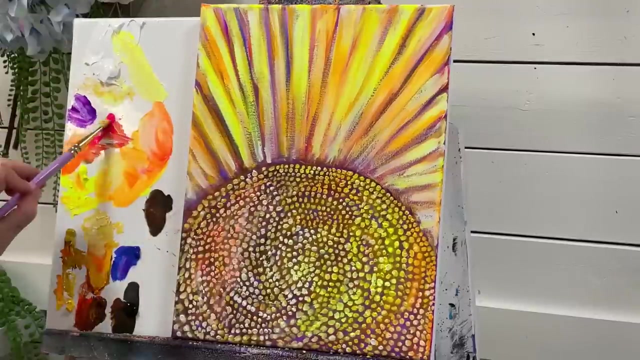 Make orange As soon as I'm kind of running out, We're going to bring this over some of the petals as well. A little bit of water, There we go. You can see I'm starting to pick up some of that white. 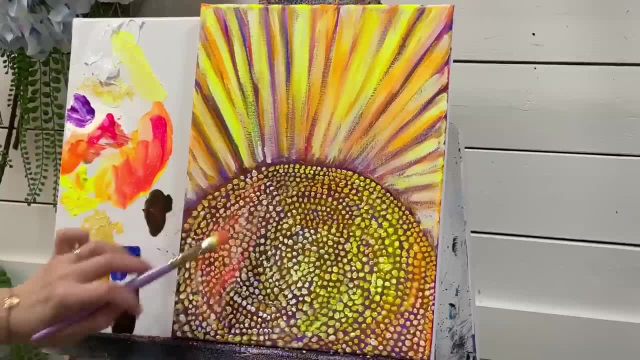 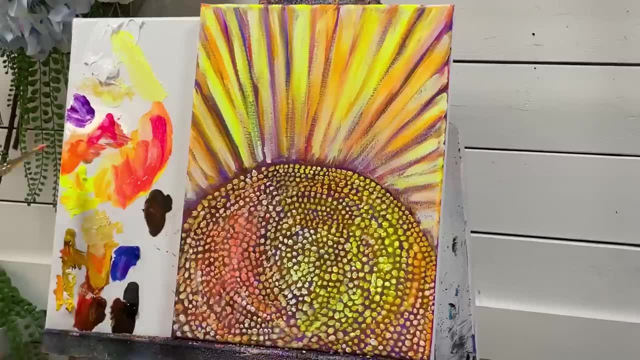 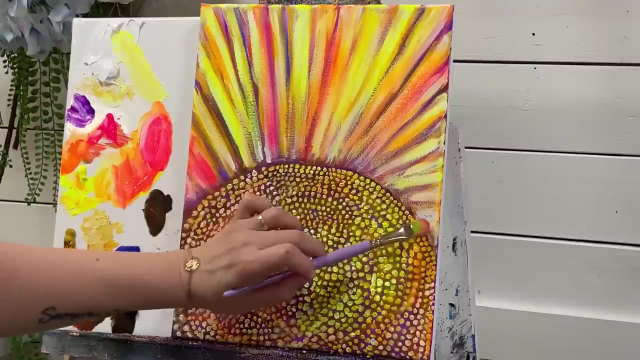 But that's Can help make it look a little bit Glurrier and out of focus. Look at the paint. Oh, so fun. I hope you guys are Really Excited to use color for this painting. I'm telling you there's something really healing about color. 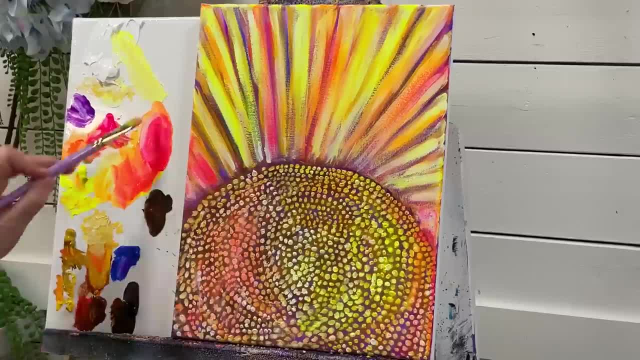 I've been doing A lot of limited palette paintings lately And I like to do that and kind of go Back and forth. I'm using a lot of color To minimal, limited palette. It's really fun, Okay. So I'm going to take a little bit of my. 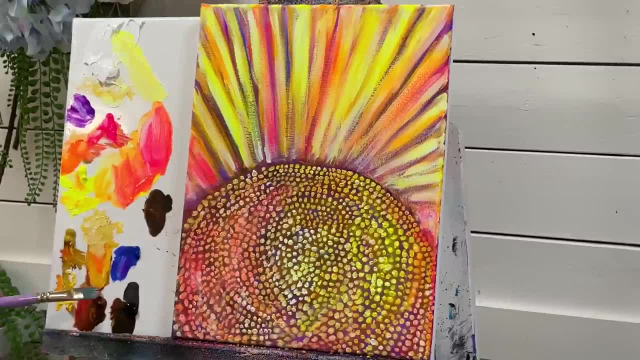 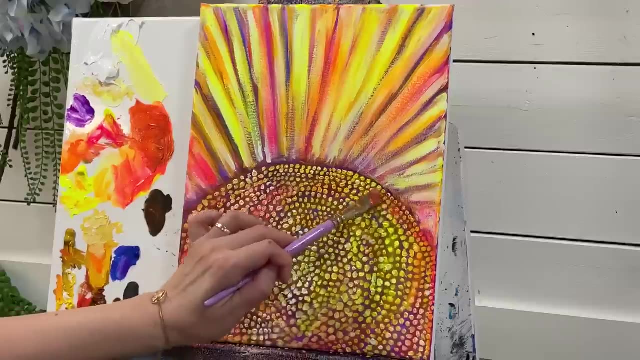 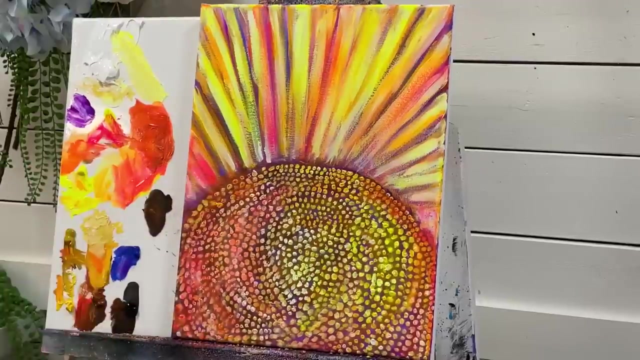 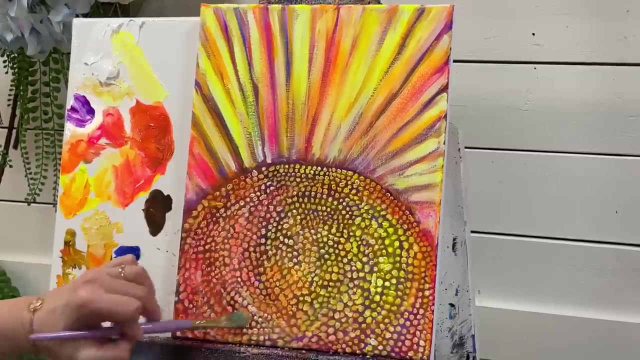 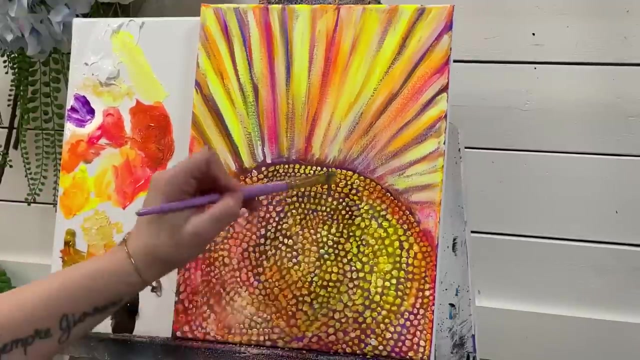 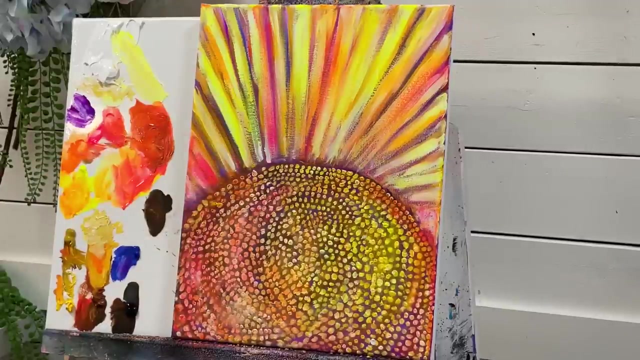 Burnt sienna, here with yellow And the rest of The pink. I'm going to add that over some of the areas here. a little bit more yellow and pink, again a little bit of water And now we're ready to start coming in with our bumblebee. 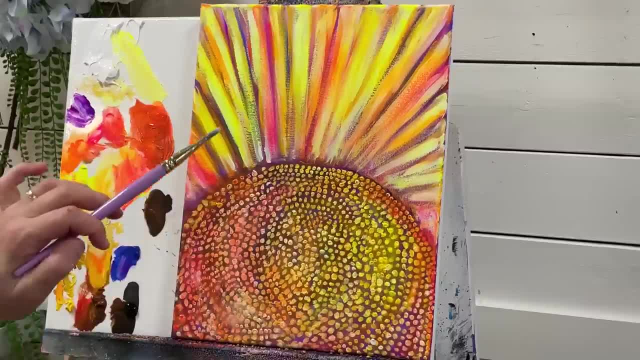 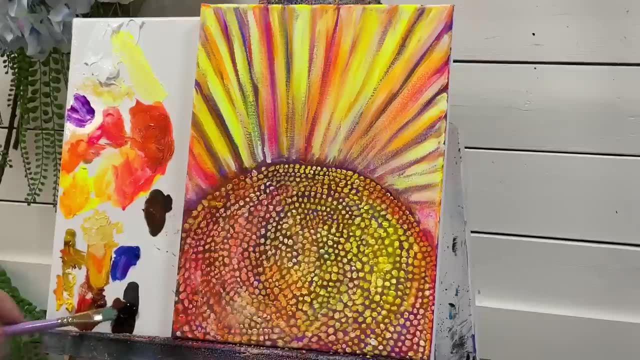 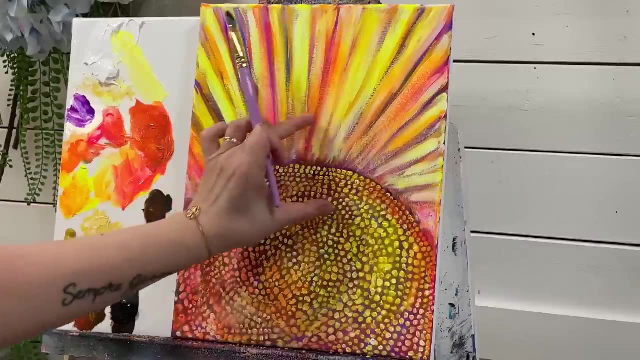 I'm so excited for this. I'm going to be using the filbert brush again for the main shape of the body And I'm going to start with some black And I'm going to add the bee right about here. I'm going to add the front part of the head. 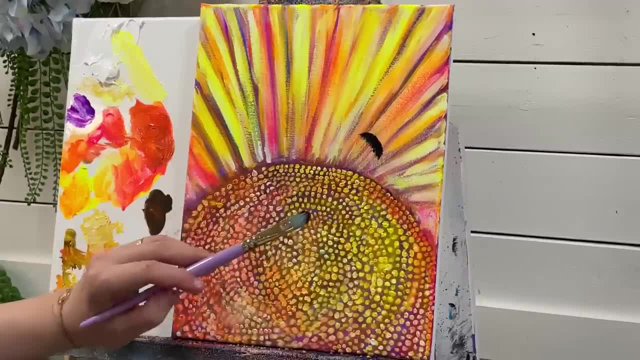 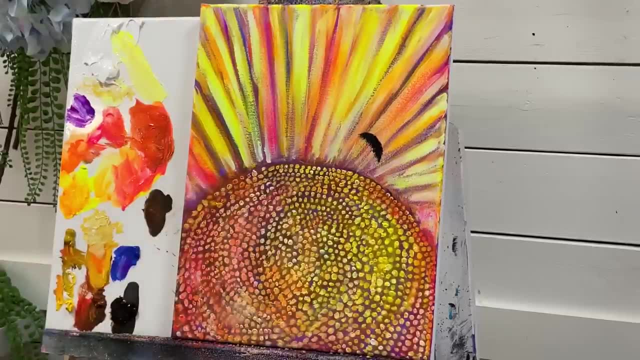 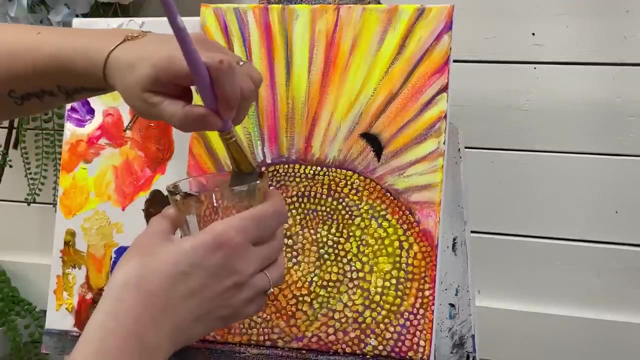 so just like a crescent moon, kind of half circle like that. And then, before I do anything else, I'm going to take my dry mop brush and, gently, I'm going to do this again with a little bit of water on it and we're going to catch the end and 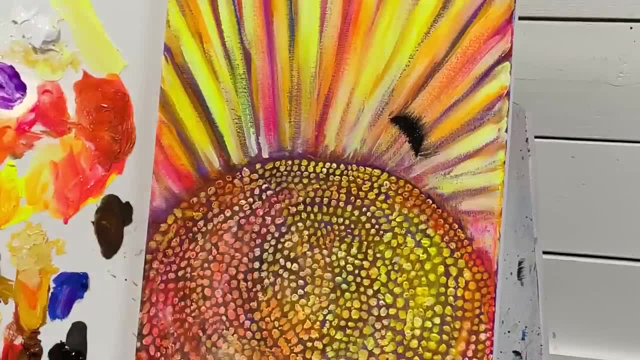 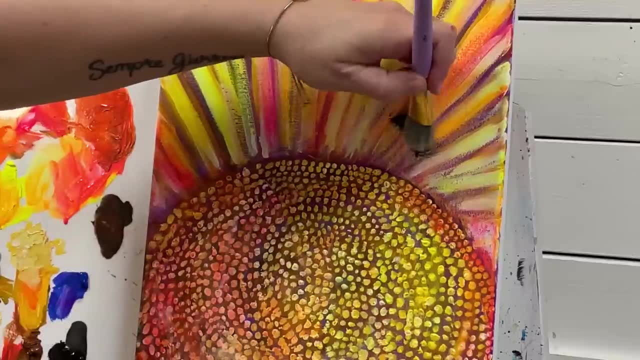 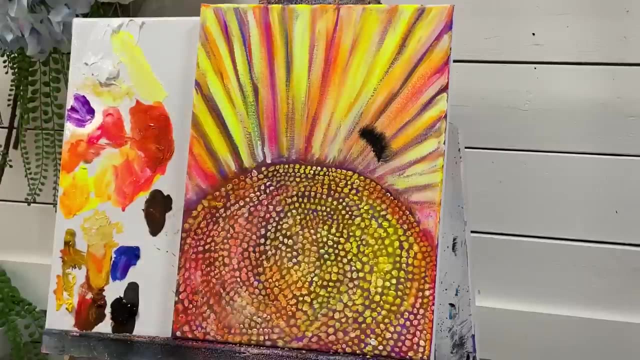 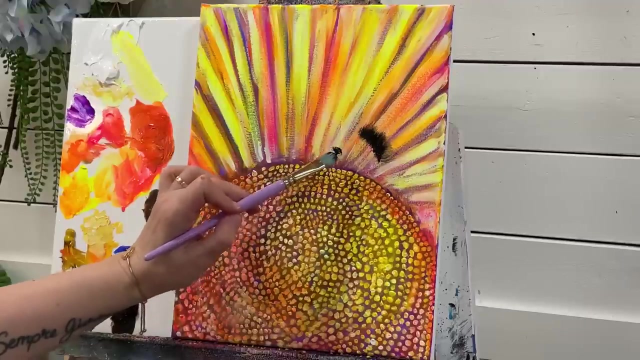 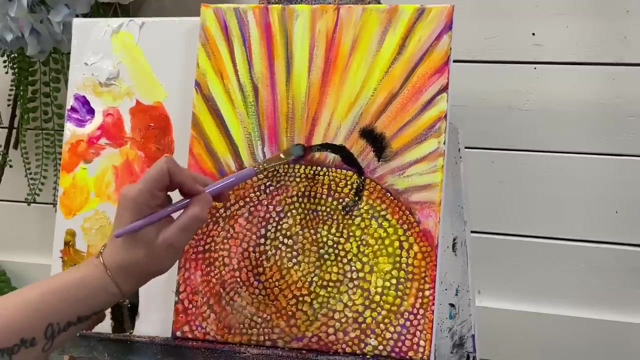 lightly pull with a brush like that To make it kind of fuzzy, Okay, Fuzzy and fluffy, Okay. then I'm going to add, I'm going to skip a little area there and we're going to come in here and add sort of a circle. 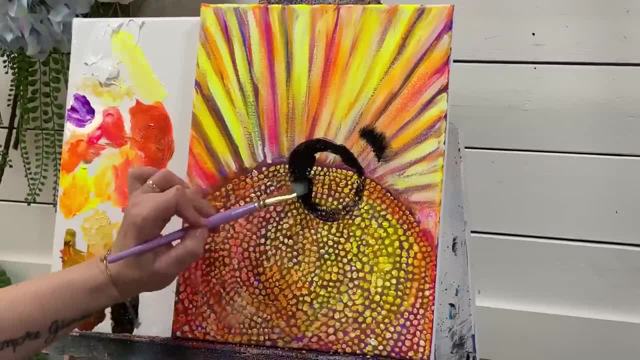 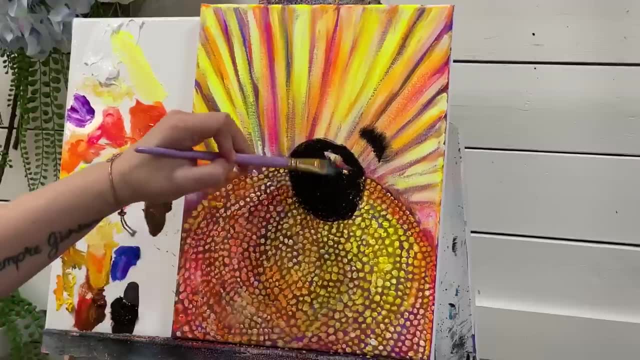 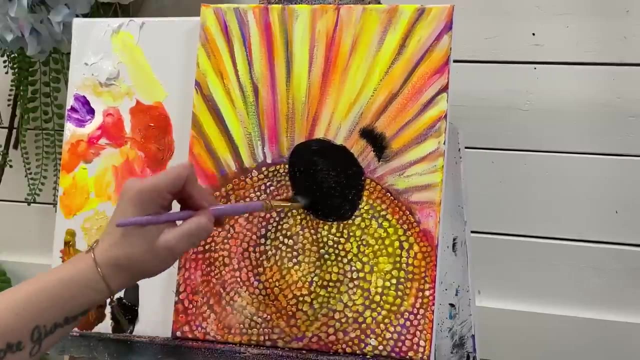 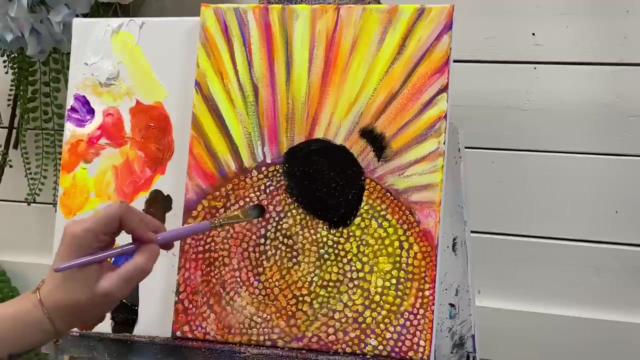 And we're going to add all this black inside covering up that part of the flower. We're going to leave another space. I'm just going to gently come in here A light little flick. We'll give it a little skinny space like this: 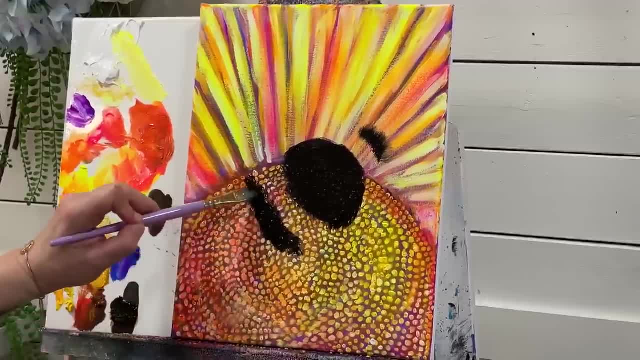 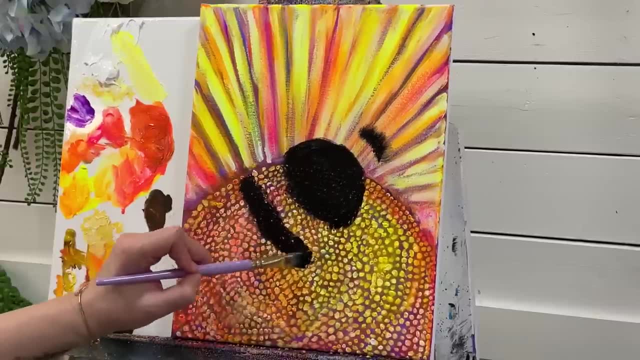 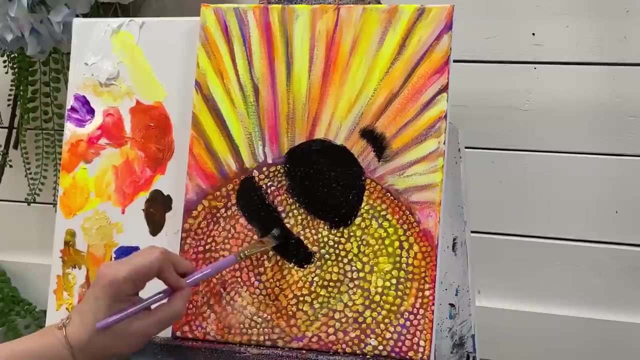 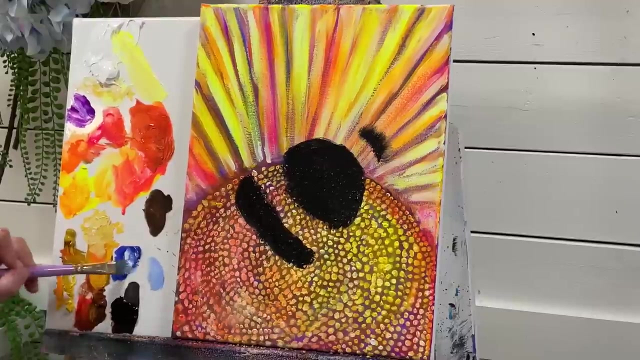 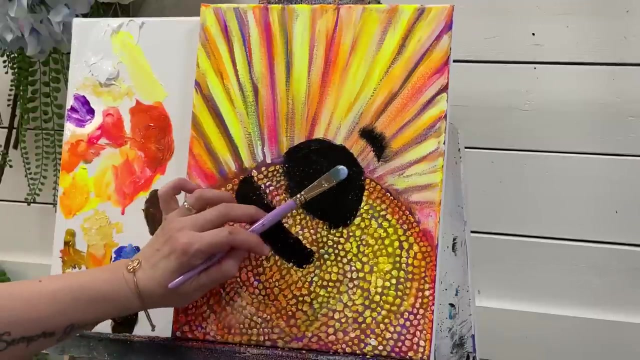 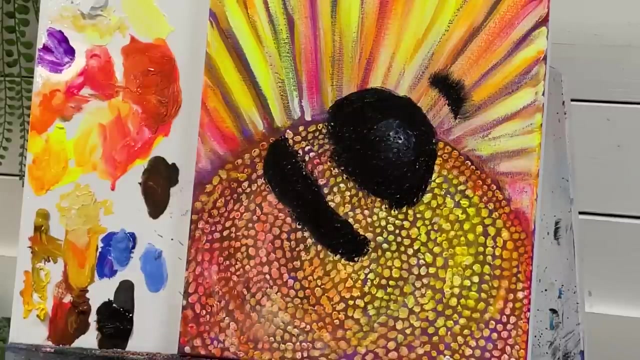 And then come in again and make this a little narrower. Going to take a little bit of white and a little bit of cobalt blue, Let's see, Okay, and I'm going to add a little shine right here Now, as that dries, I might add a little bit more. 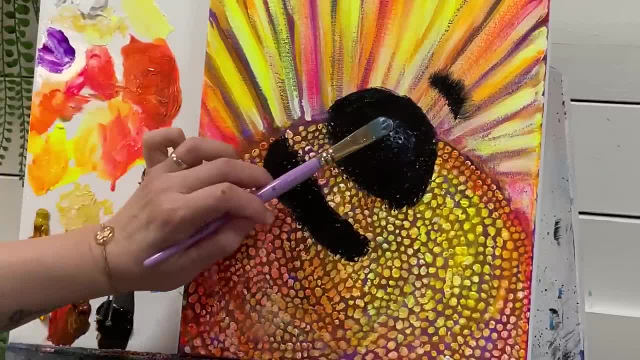 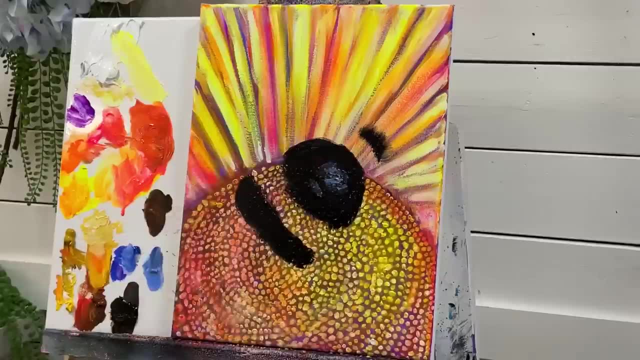 or you can just use very little pressure and add a little dab there and a little dab there where there's kind of got a little bald spot. Okay, for our next color clean brush, we're going to take some burnt sienna, a little bit of white and a little bit of yellow ochre. 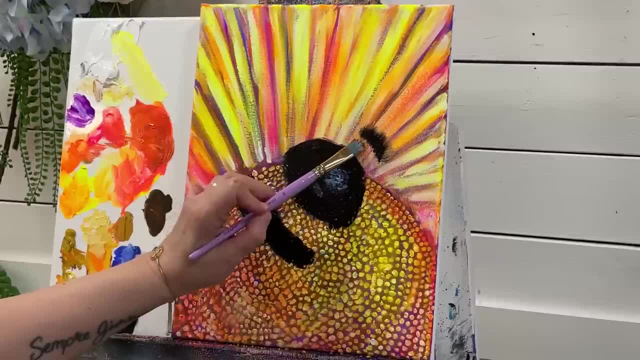 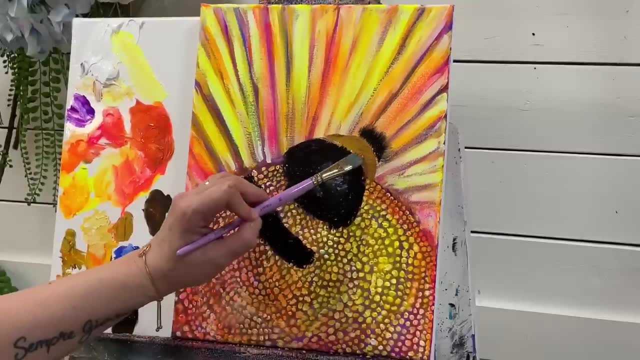 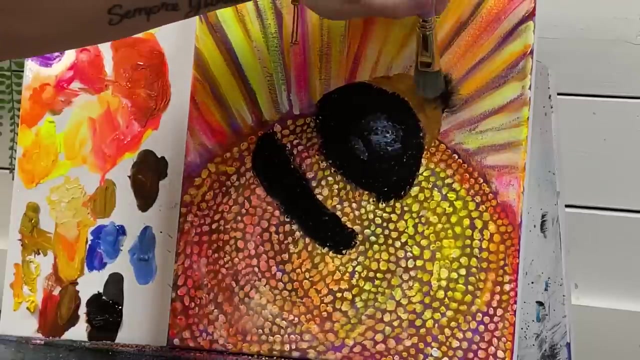 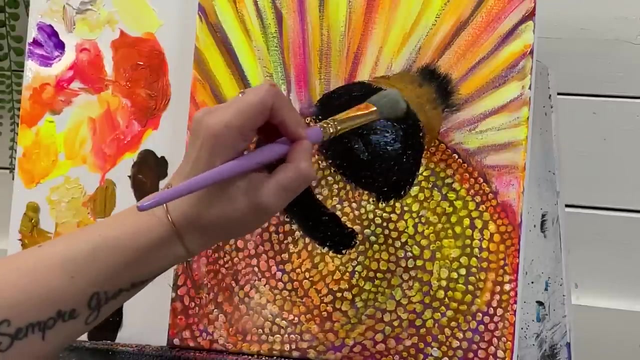 and I'm going to dab it in here in between the black areas. I'm going to go over to my mop brush again: gently flick, flick, flick. we'll flick a little bit this way too, and then a little bit this way, so we get a little bit of that. 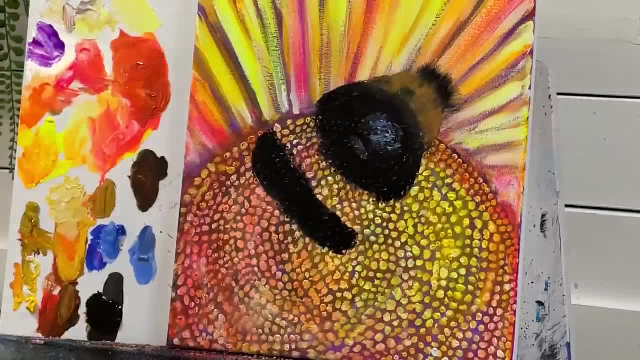 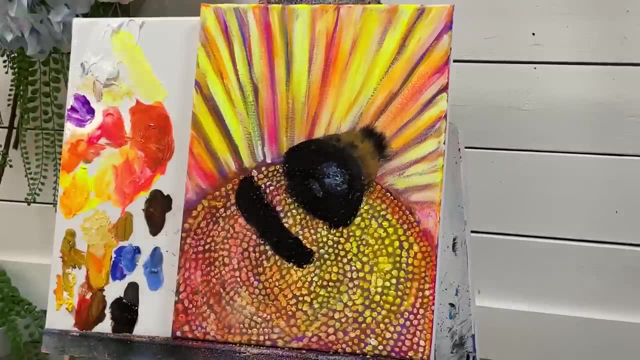 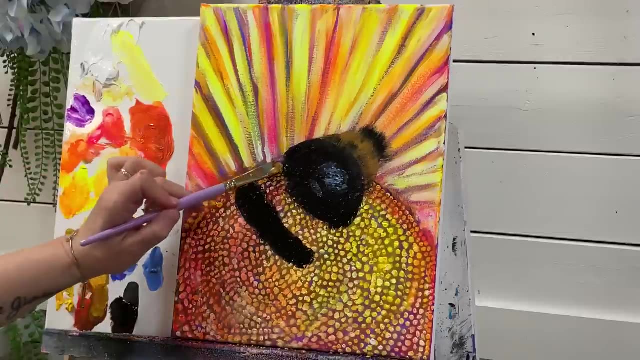 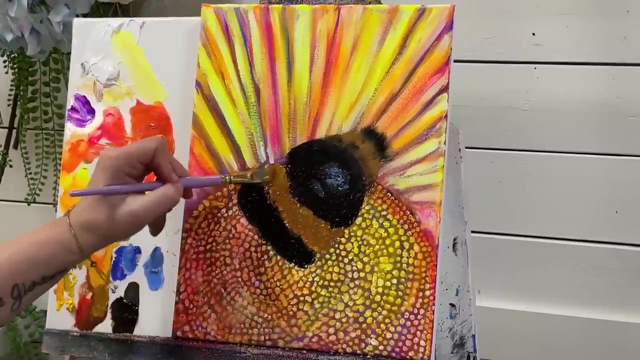 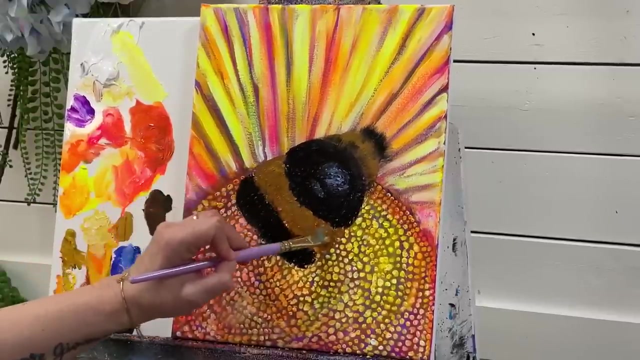 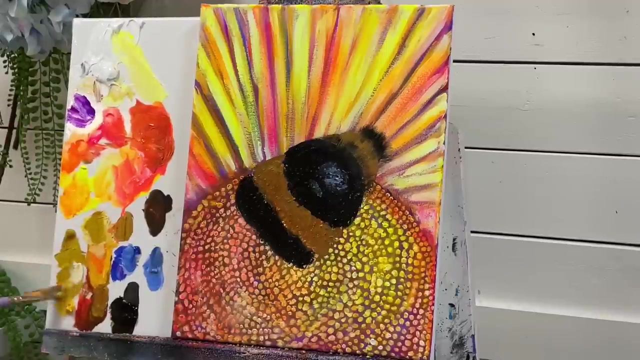 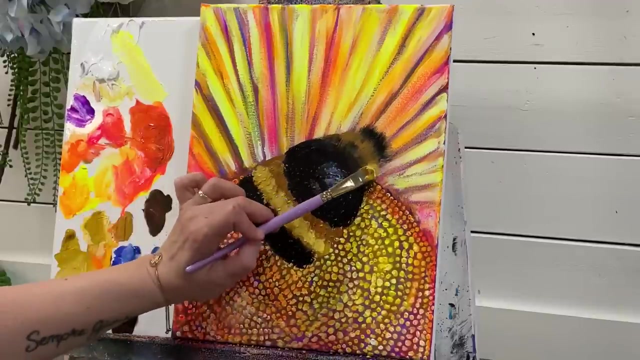 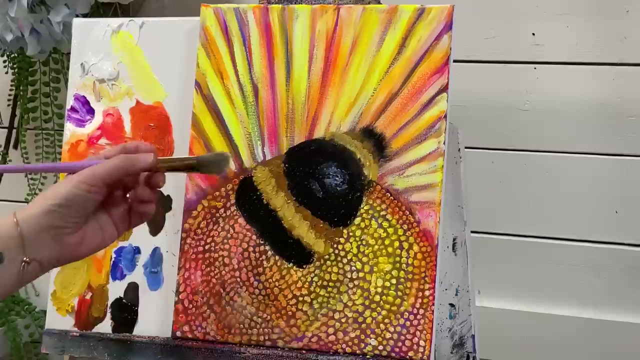 black in there, pick up a little bit more, okay, and now we're going to add some in here and then a little bit of yellow, ochre, white and cadmium. We're going to add the lighter part down here and then right here. Okay, I'm going to take my brush again and I'm going to lightly. 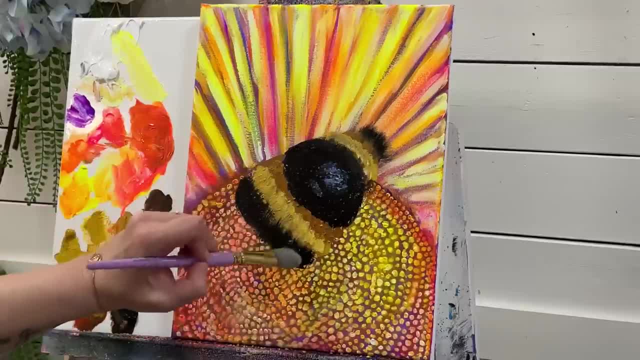 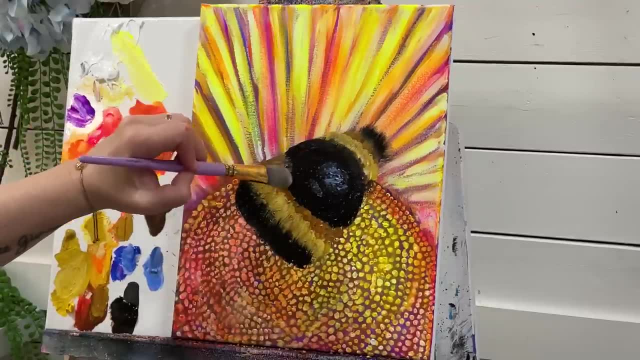 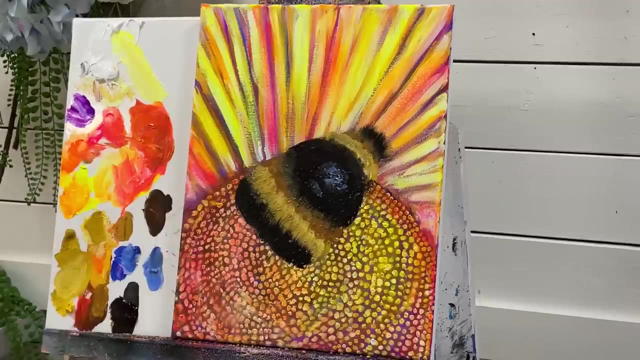 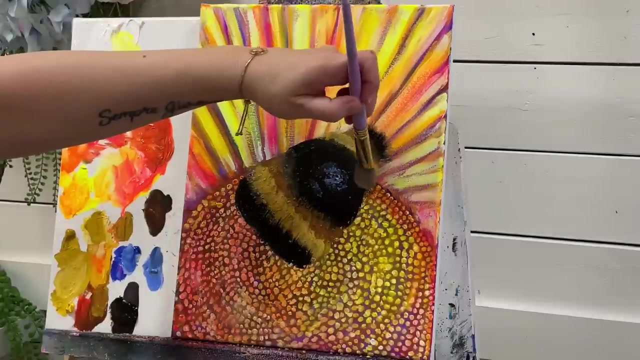 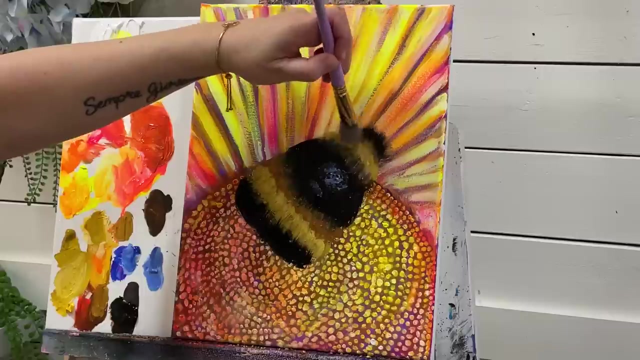 pull, pull, pull and flick Off of the black and to the browns and so on and so forth. Just a light little blend. Just be gentle, Just go in there, Just blend everything in. Just blend everything in. I'm going to go ahead and just tap this all over. 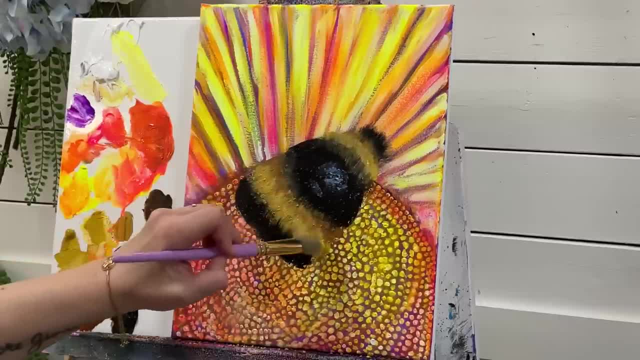 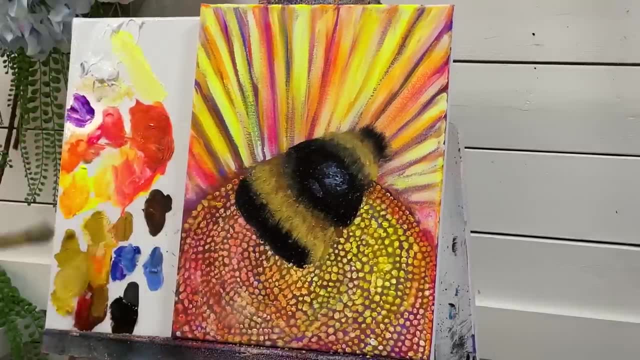 I need to add a little bit of white to it. I'm going to go ahead and just mix this up. I'm going to go ahead and just mix this up. This is just one of those really easy ways: put a little bit of yellow and white on there. 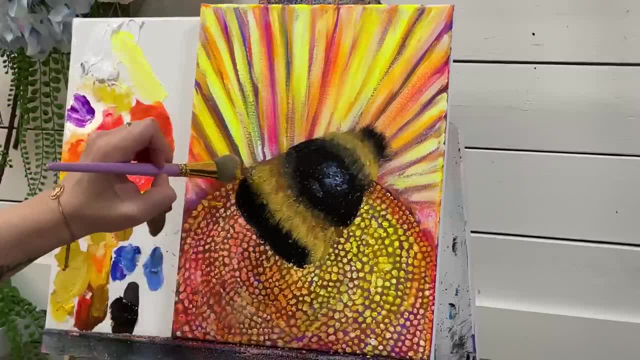 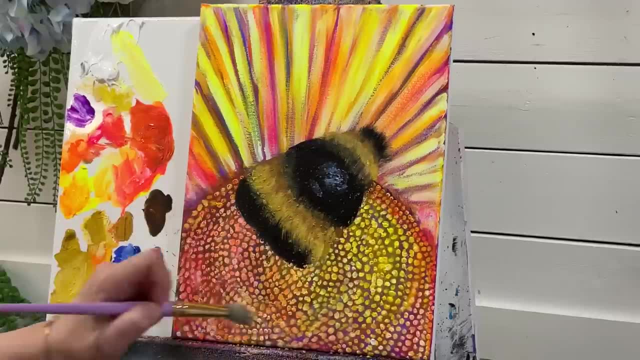 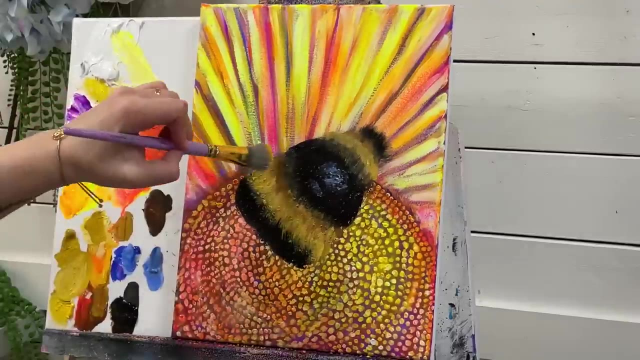 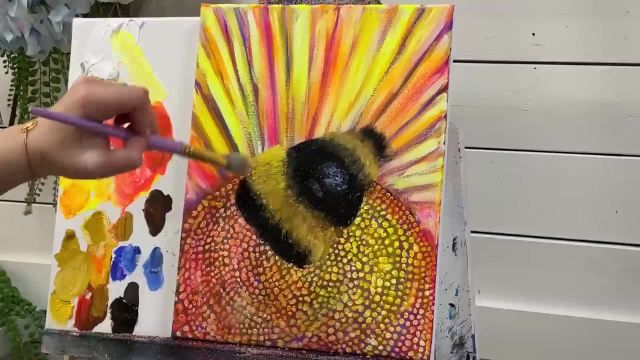 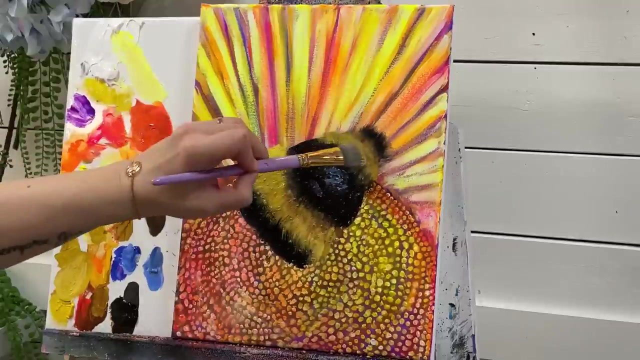 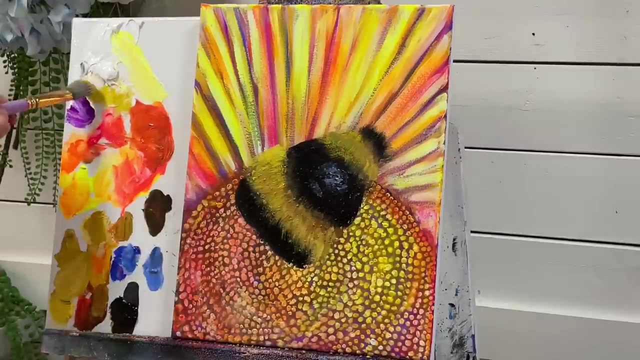 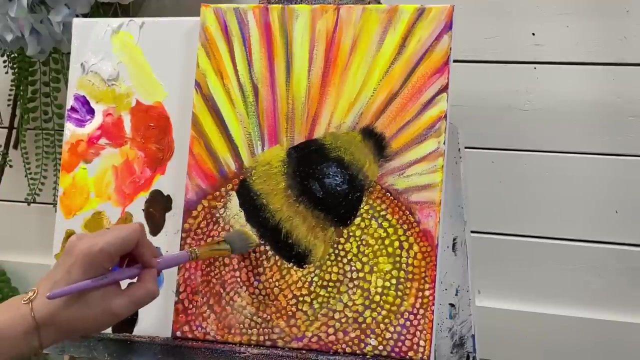 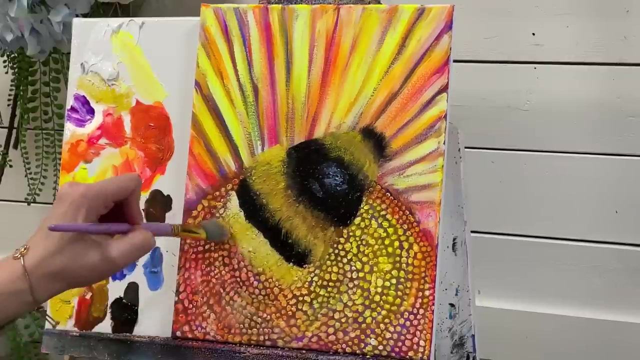 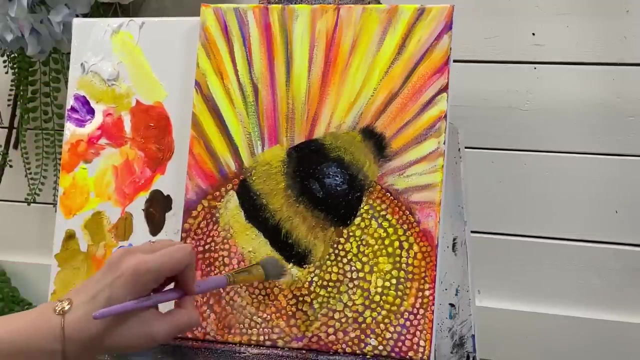 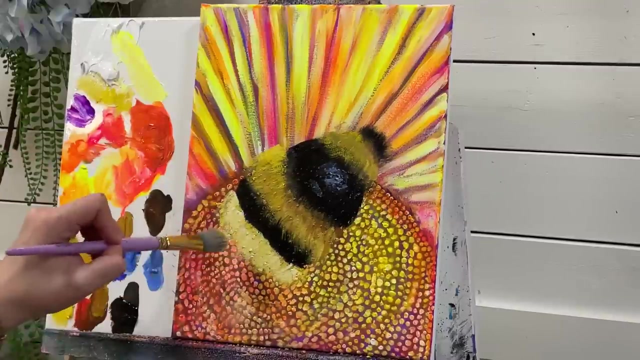 Those easy ways of adding fluffy fur. Okay, now we're going to get this area here. it's going to have a little bit more white on it, So I'm just going to gently pull and flick. Okay. Okay, Now adding more white. 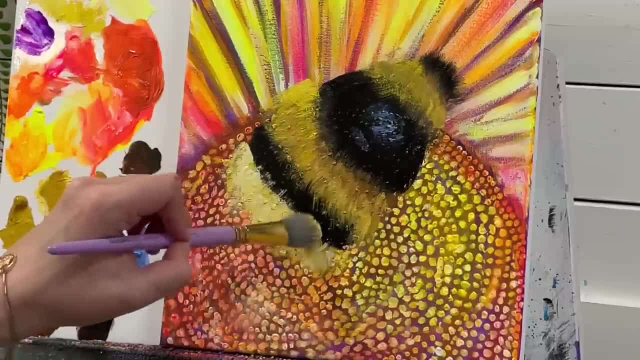 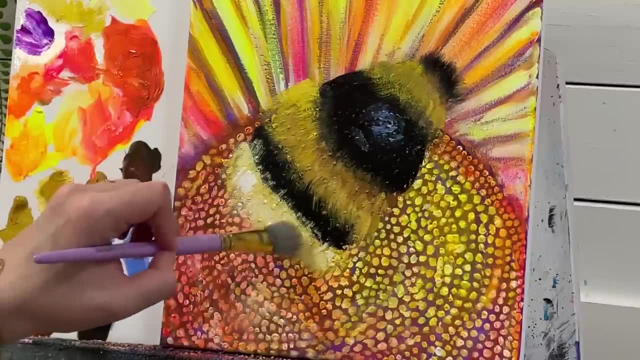 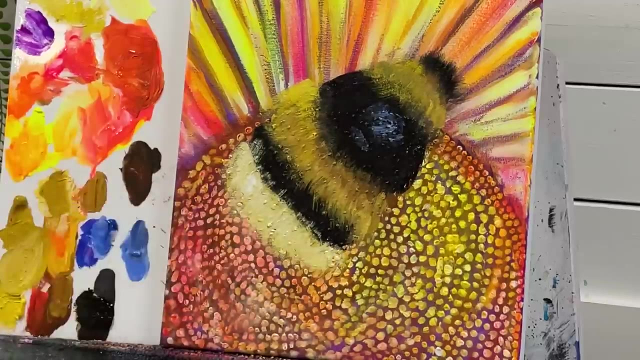 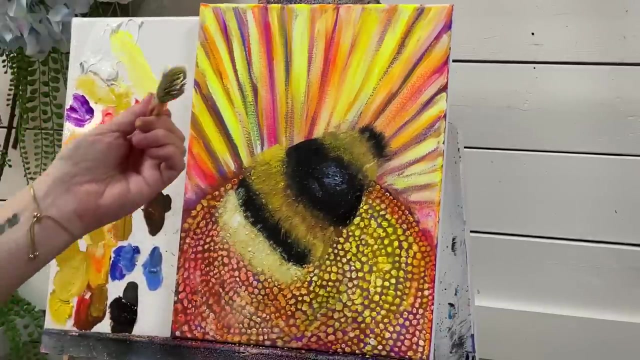 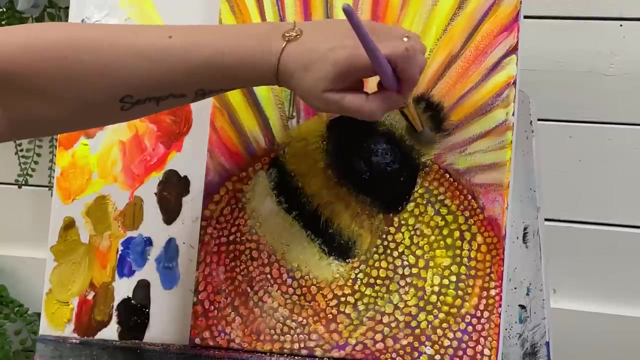 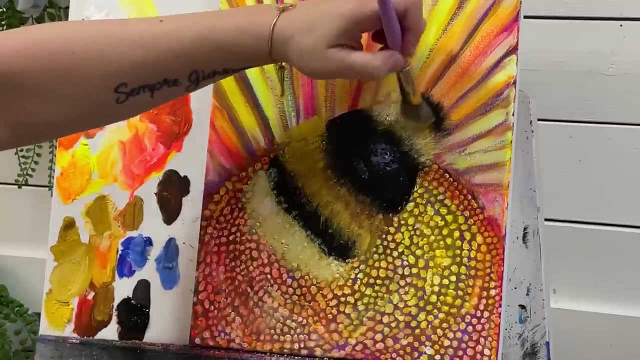 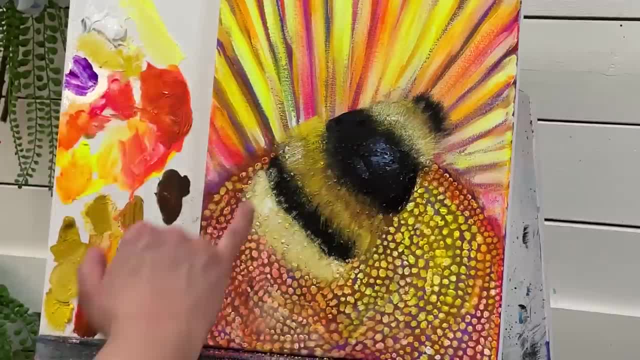 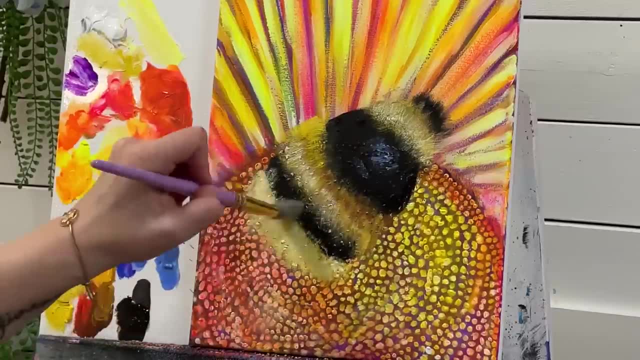 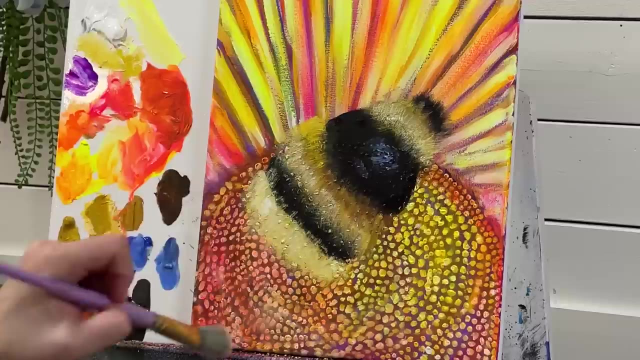 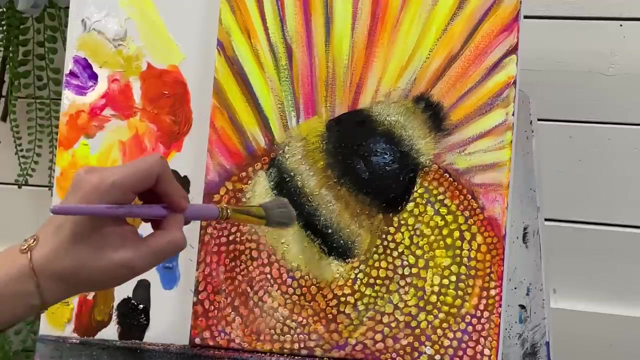 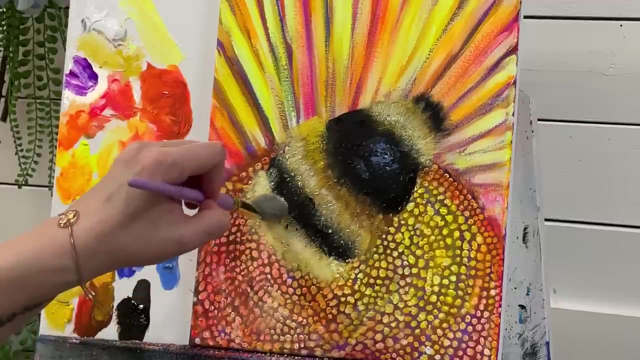 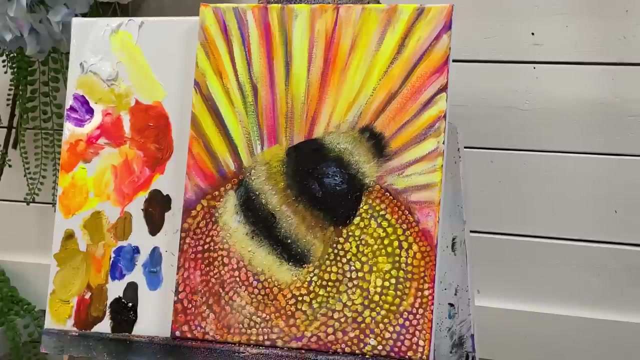 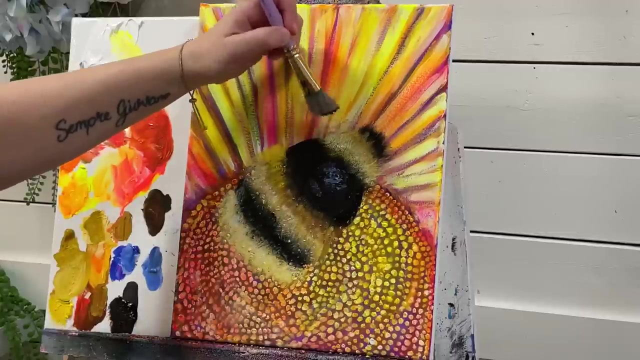 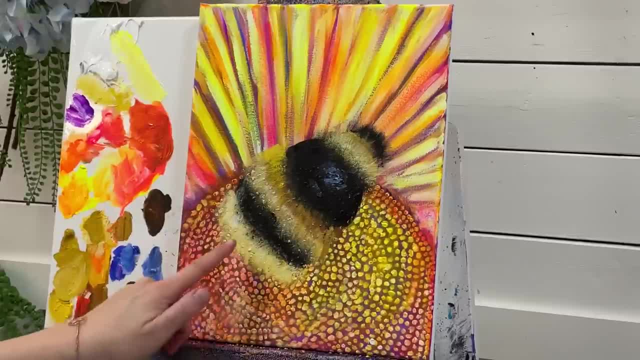 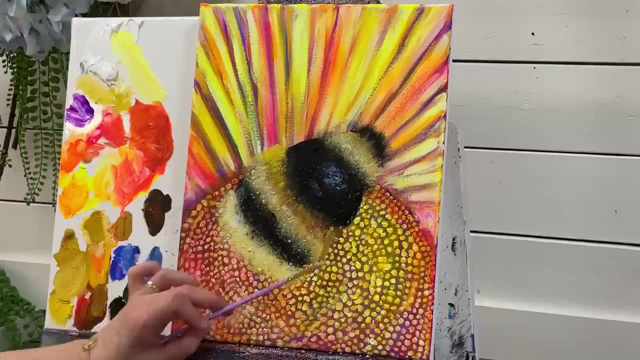 Okay, so the next thing that I want to do- before I add the black, I want to make sure that I add the final highlights to the end- is I want to come in and add shadow, a shadow around the body of our bee, and I'm going to use my round brush. 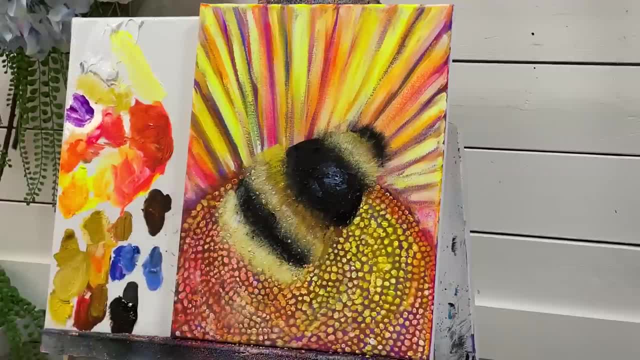 You can use any brush you feel comfortable with, whether it be the dagger we used earlier or the filbert brush, and I'm going to take my burnt sienna a little bit of black. I'm just going to bring it over here, make sure that it's not too thick, and I'm going to 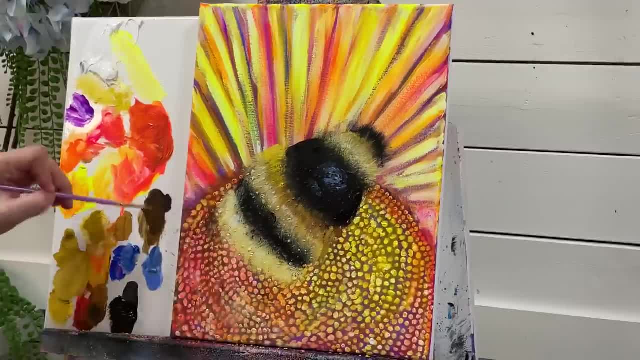 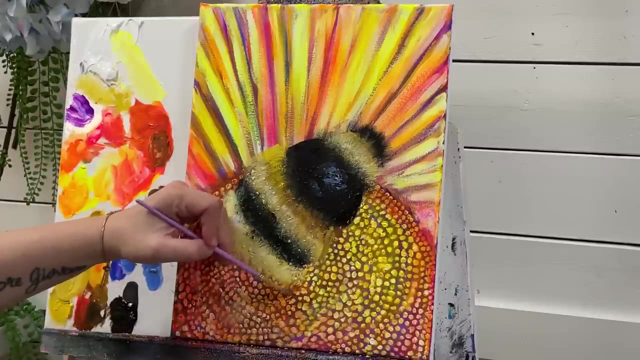 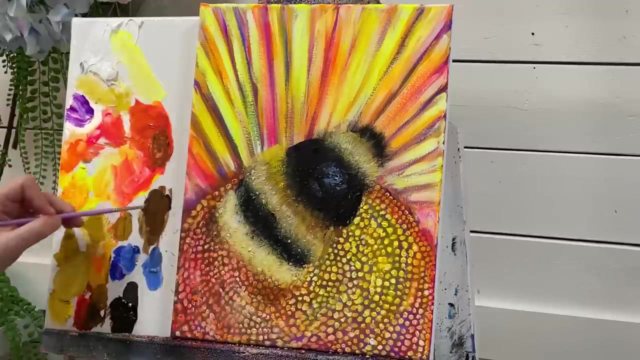 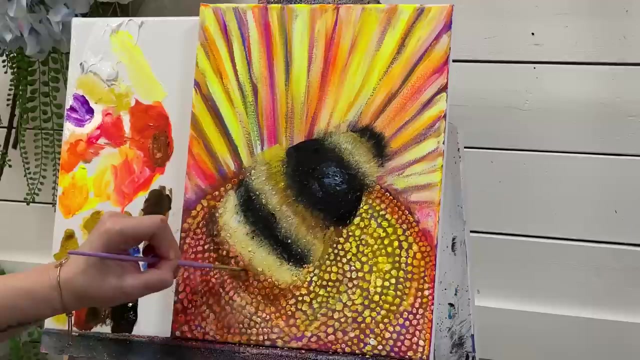 come around. I'm going to use some of this pink and orange in here as well and just lightly come over here. I'm just going to dab around the spots very loosely to give them a little bit more depth. Now I've got a really cool brush that I didn't show at the beginning of the video, but I want. 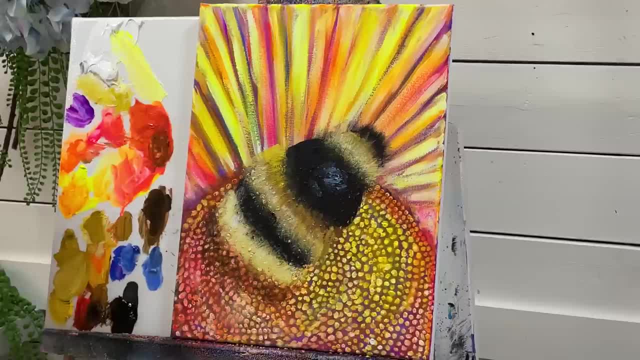 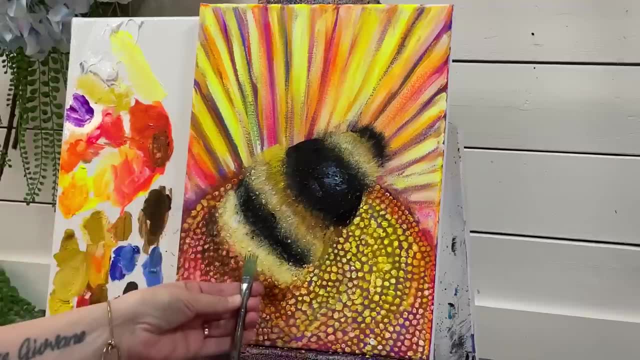 to show you guys. now I'm going to demonstrate how to use an eventail filbert brush. There you can see it better like that. So it's like a filbert brush, but it's had sections snipped out of it so it looks kind. 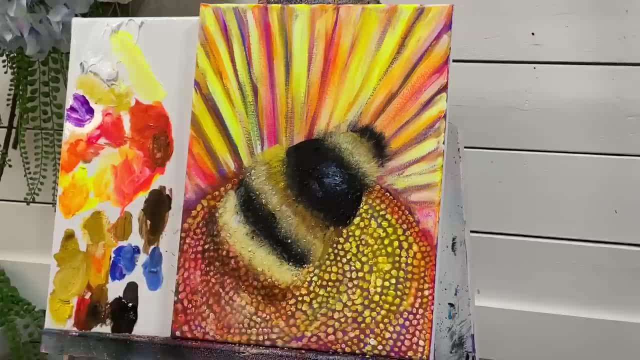 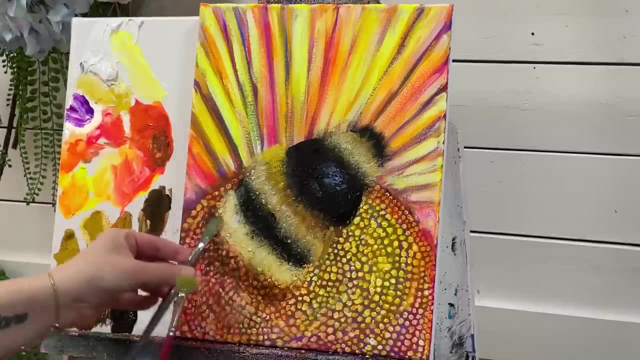 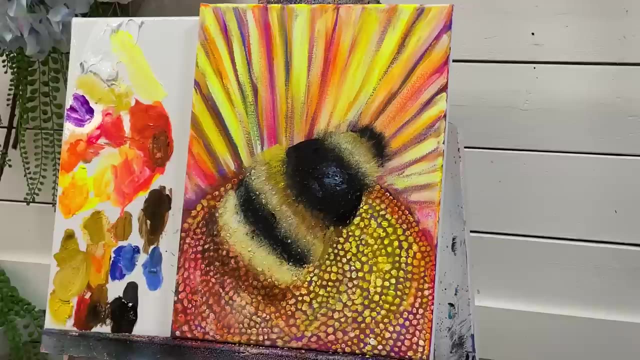 of like a rake, and I also have a fan brush that actually looks like a rake and it's a fan brush, So I'm going to do the same kind of thing, but this I'll have a little bit more control with, for the final hairs and little highlights before we start our wings. 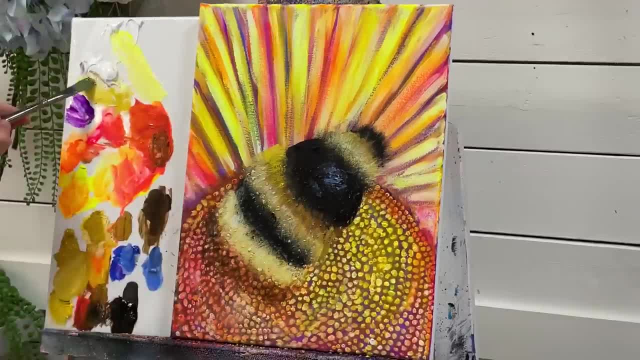 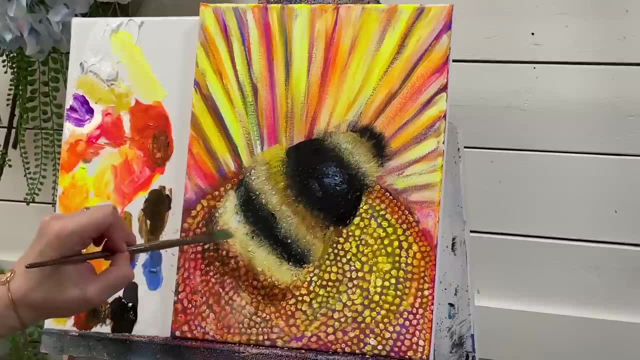 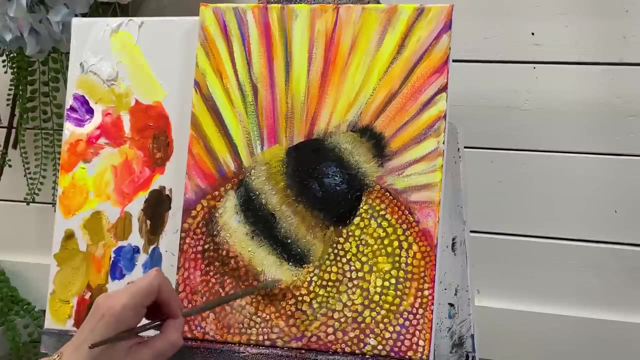 So I'm going to get my brush wet and I'm going to pull into a little bit of white and I'm just going to come and add this a little bit thicker, but this will get a little bit thicker and it's going to give us the spaces that we need. 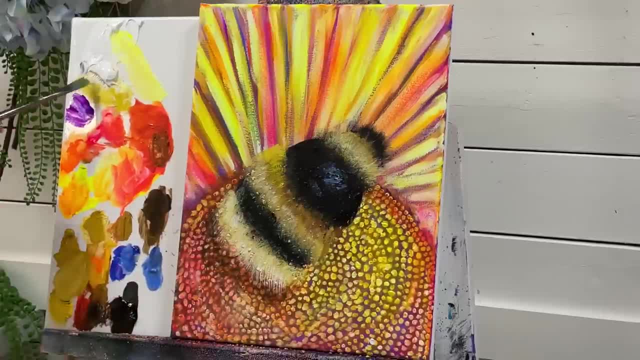 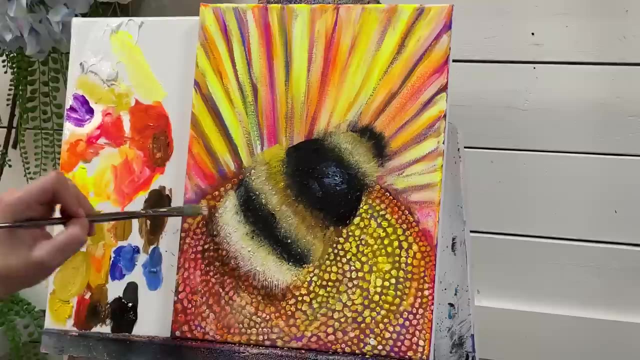 You can do this with the mop brush too, but I just want to show you guys and introduce different brushes that I think are amazing in helping you learn how to apply these brush strokes with them, so that you can learn how to paint hair and fur. 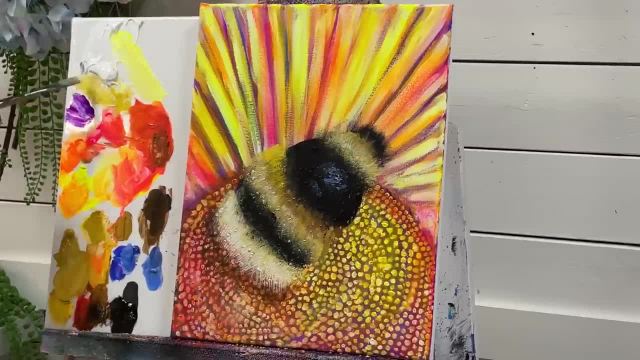 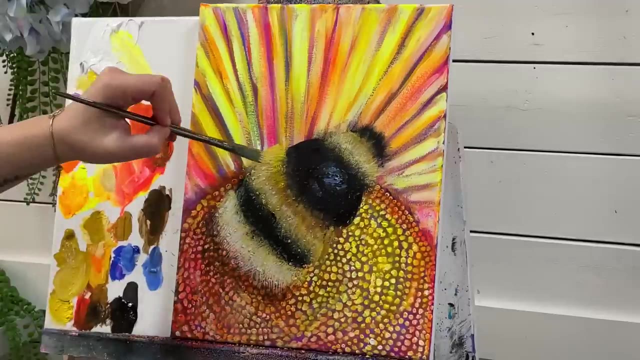 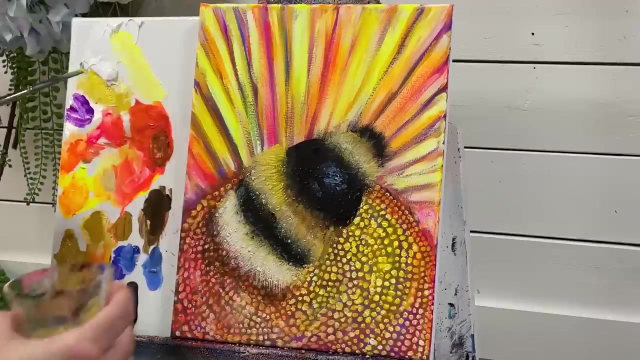 Okay, so now I'm going to take some of the yellow ochre along with the white. I also want to add a little bit of cadmium yellow. Get a little bit more yellow in here. So what happens is that I'm just taking a little bit of water here. 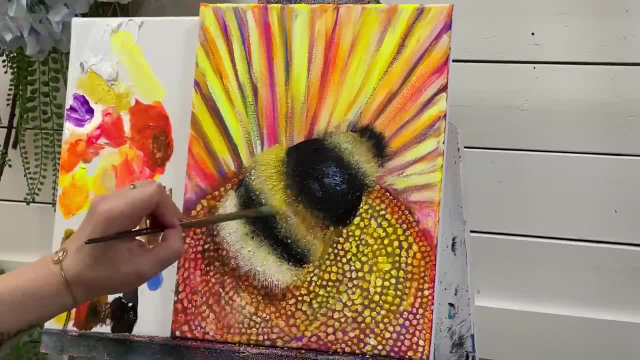 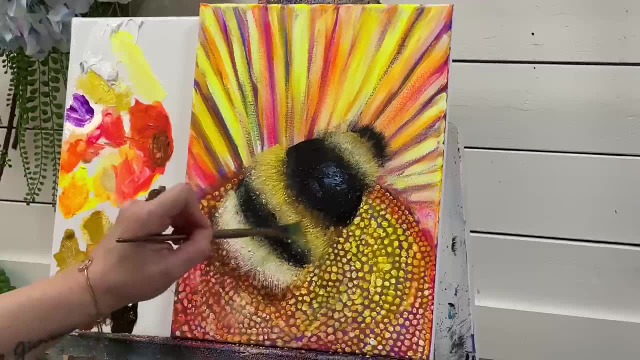 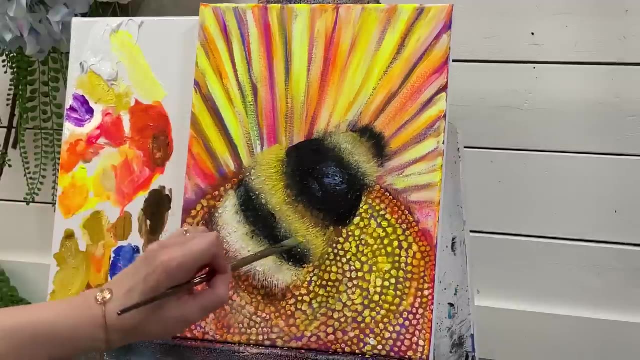 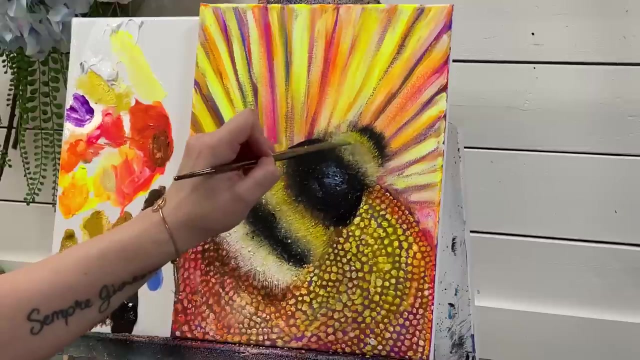 What happens is the acrylic dries a little bit darker, so it's normal to lose your highlights after the first application once it dries, And then have to come back and add some more, maybe a little bit heavier, with my yellow in here. 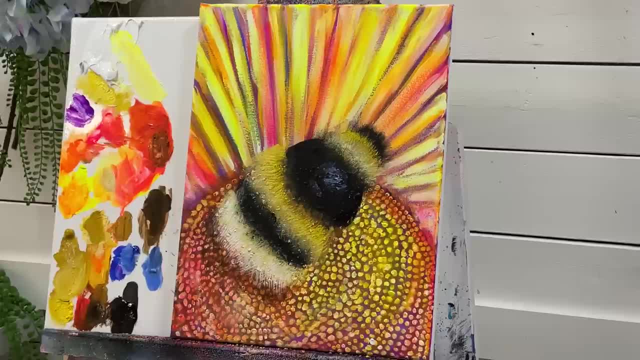 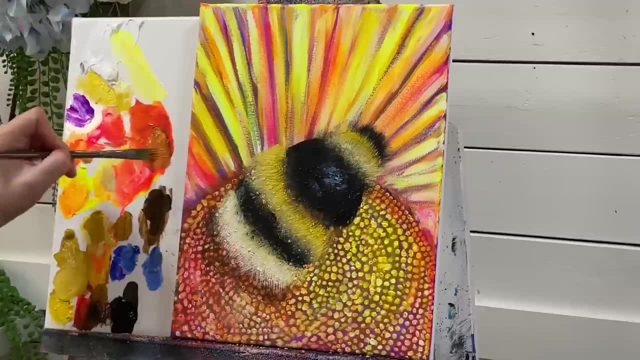 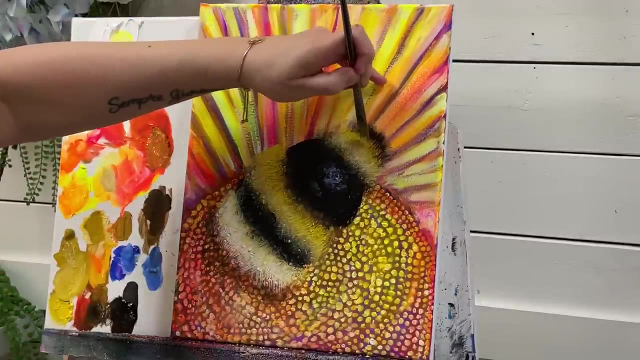 I think this bumblebee is looking pretty cute and furry and fluffy already. Okay, now I'm going to go into the pink and orange and yellow- kind of like burnt sienna- and Okay, Okay, I'm going to go in here and just layer this. 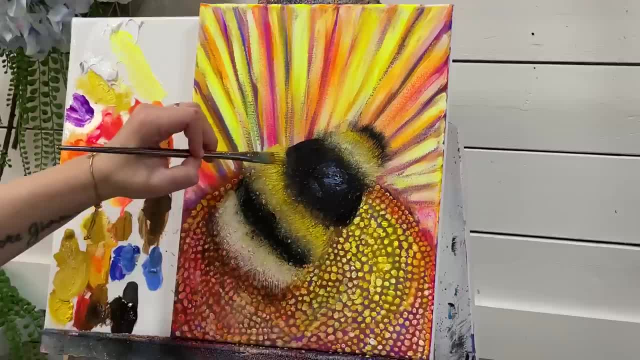 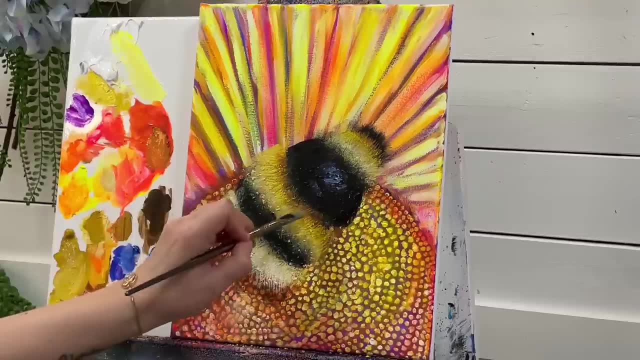 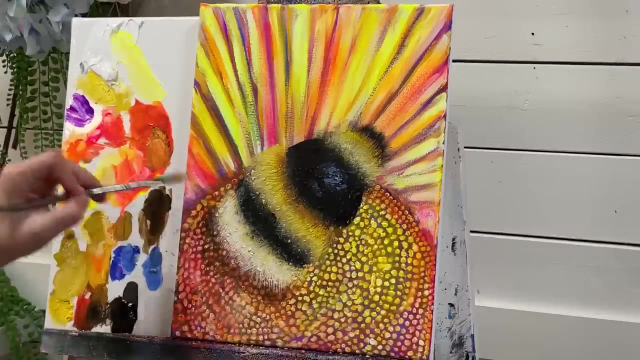 Just placing my pinky here to help guide me. So I'm going to add a little bit of this in between the black and the yellow, where we added more of the burnt sienna at the beginning, And then we're going to have just a little area in here. 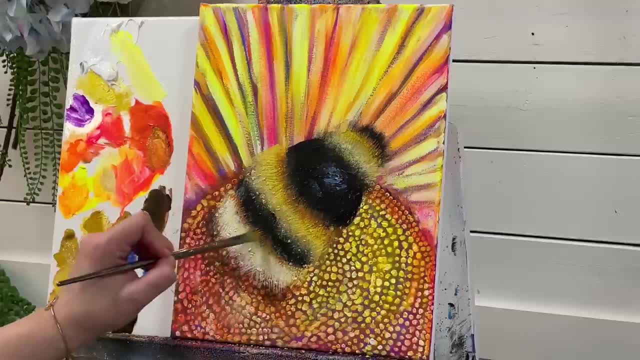 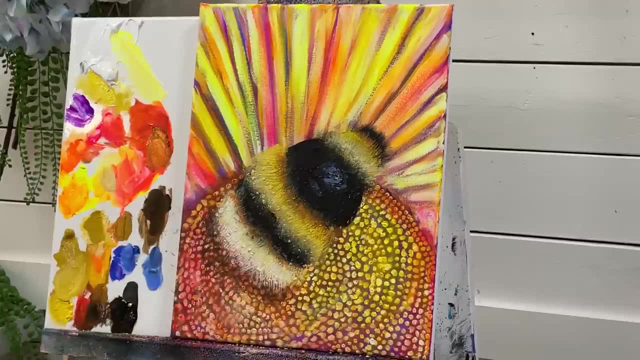 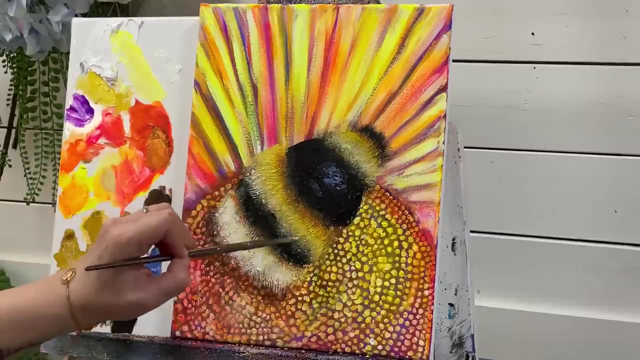 Tiny little area, Okay, between the white and the black, okay, so i'm gonna just add a little bit more, um, a little bit more white before we work on our wings, so i don't even want to thin that out just for this little area in here. 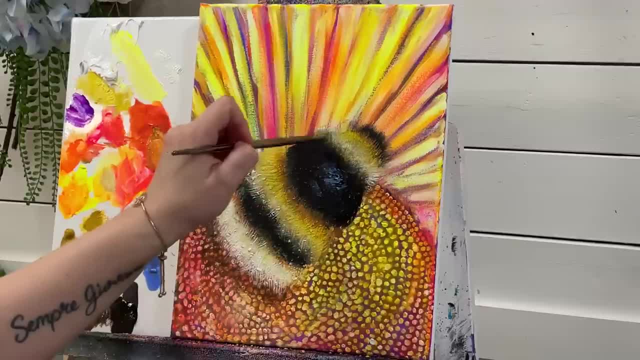 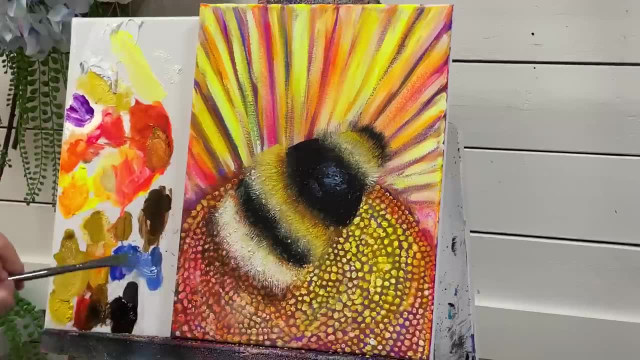 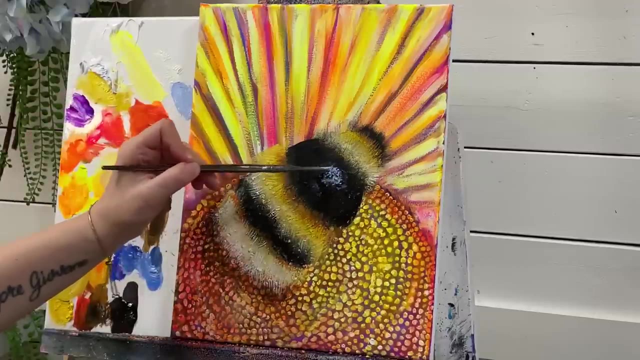 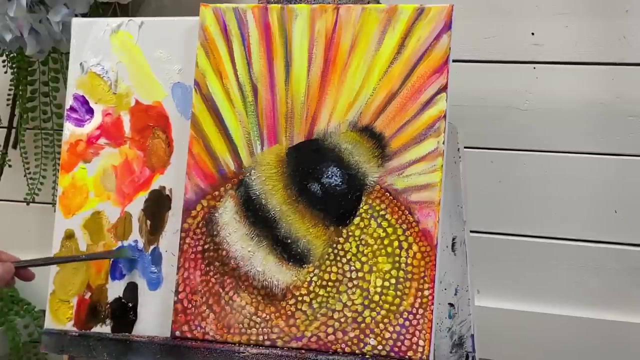 catch a little bit there on the side and then i'm going to, just, i'm going to, just i'm going to use this brush along with some white. you can use any brush that you want- a little bit of white and blue. just go over those little highlights again, because i'm using a lot of color and enjoying. 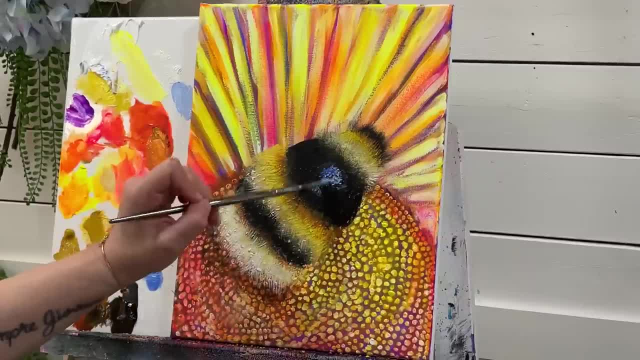 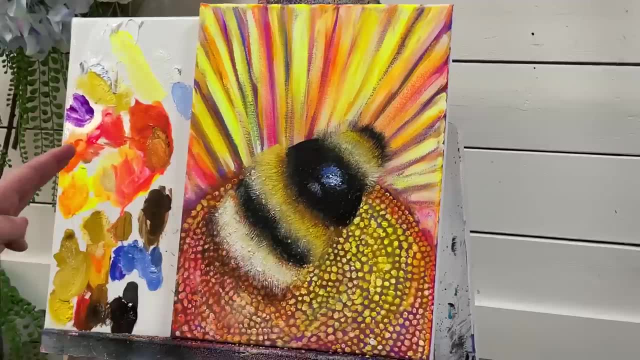 color in this painting. i'm going to be a little heavier with the blue now and just add that there now we're not going to see the um legs of the bumblebee, we're just: it's, it's, we're not able. those aren't going to be visible in this painting, so we're going to leave those out. 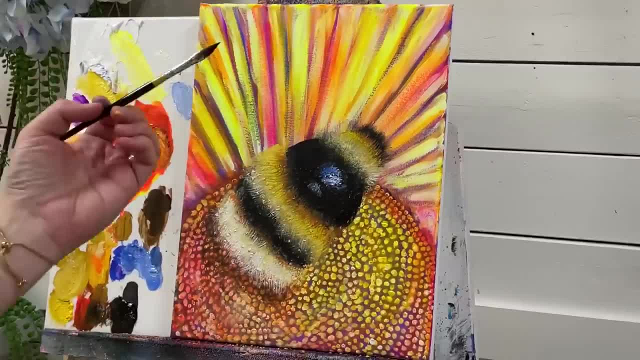 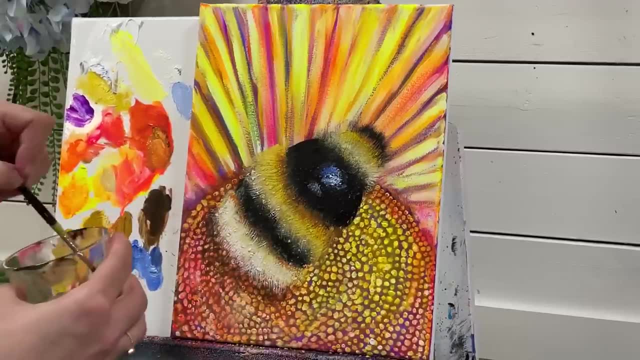 and just start working on our wings. now, the wings i'm going to be painting with the dagger brush. if you don't have any of these brushes, just use any brush that you feel comfortable with, and i'm going to start off with a little bit of white and blue. 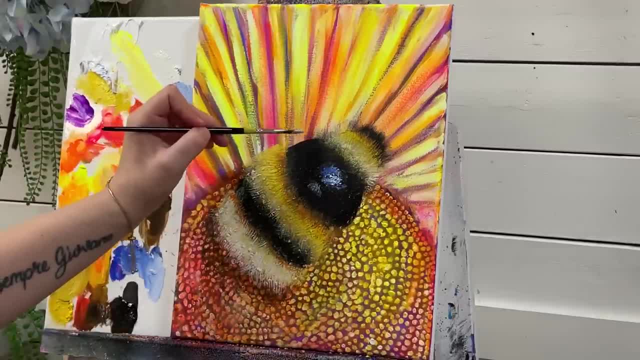 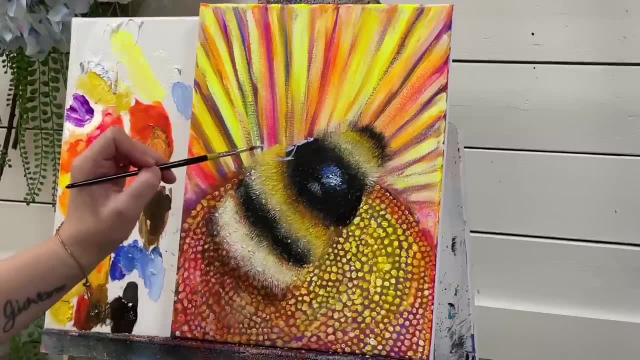 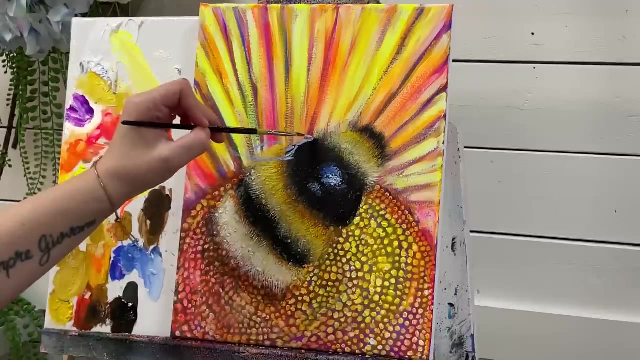 and i'm going to start the first one here. it's gonna start right here, so i'm just going to add little dabs and it's going to come in here. so So I'm gonna come out, create kind of like an almond shape, And then we're gonna come up. 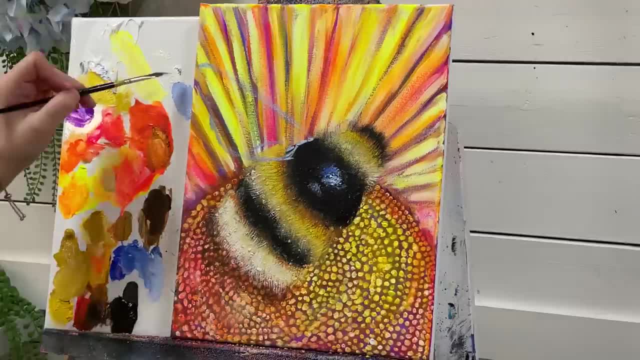 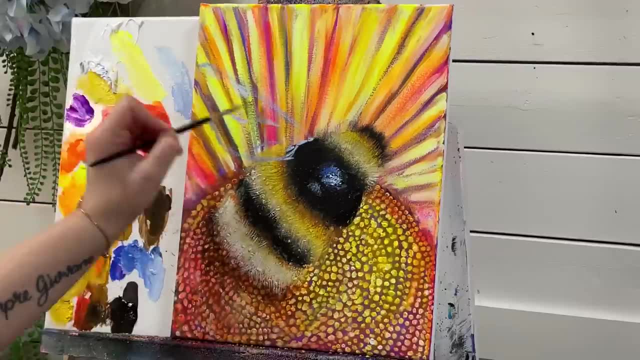 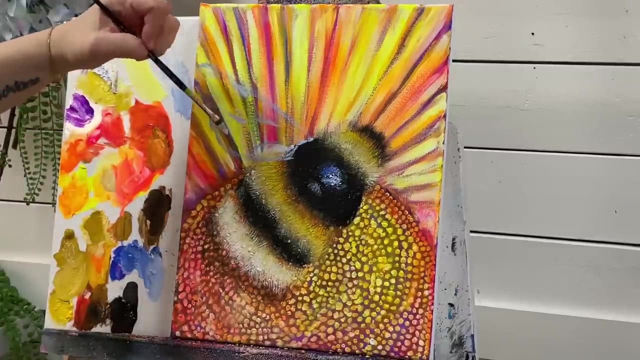 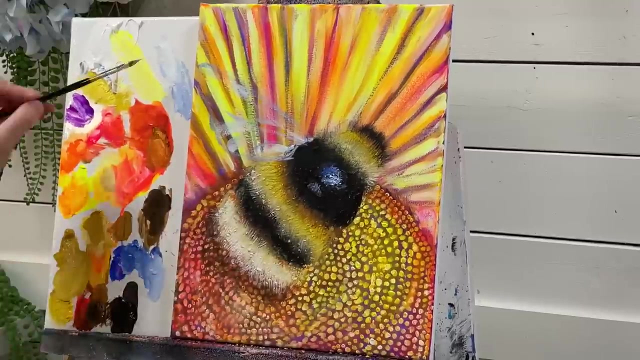 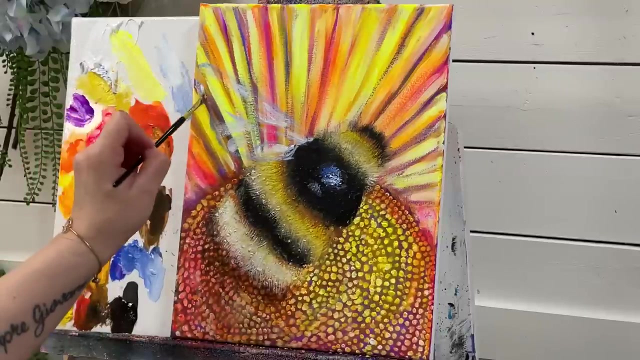 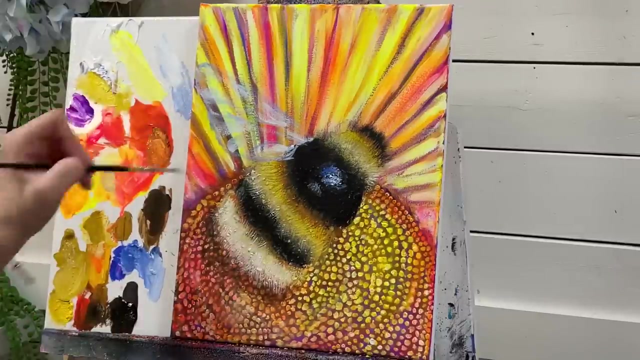 Like a butterfly wing. Take some extra white in with that And all we're gonna do a little bit more white, Kind of just dry brush over Little patches like this, Little lines. It'll show up a lot more when we come in with our black. 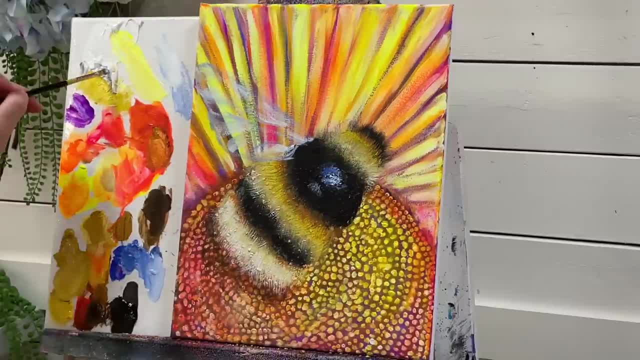 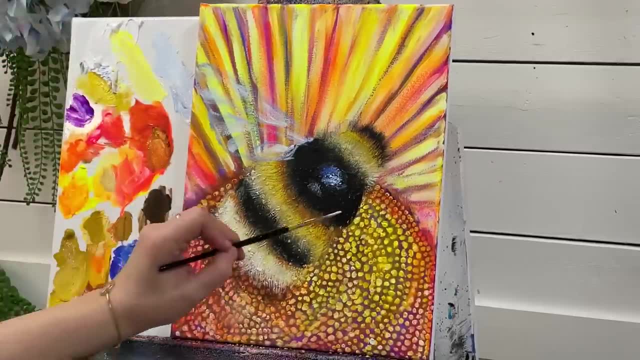 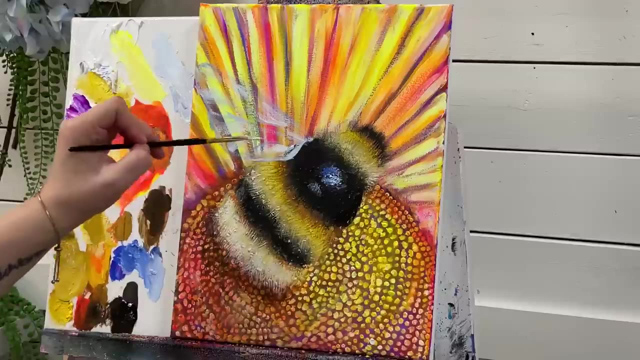 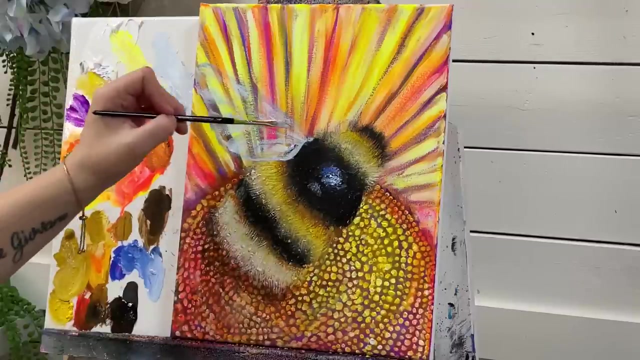 But let's move on to the next one And leave that for a little bit. We've got a little bit of blue in there And this other one's gonna come just There. that's a little bit more visible. But, like I said, we're gonna. 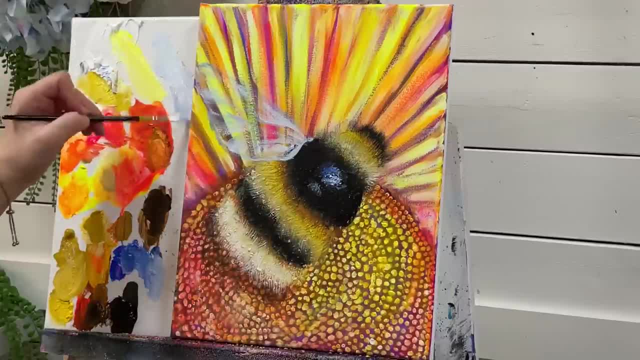 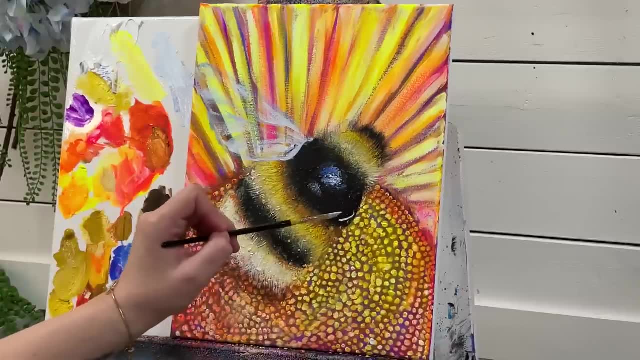 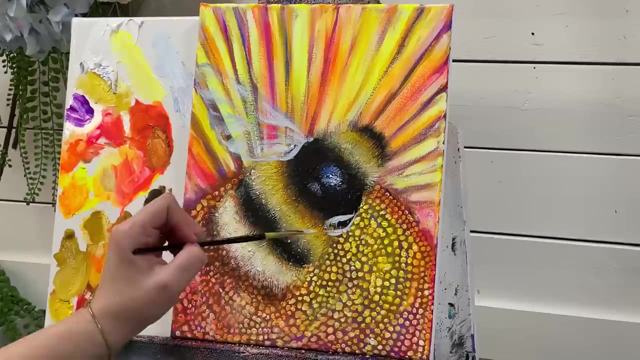 Add the black lines pretty soon And then add a few more highlights. So we're gonna come in here And add the wing. Coming up here, Add a little kind of raindrop shape right there And then bring another one down. That's bigger. 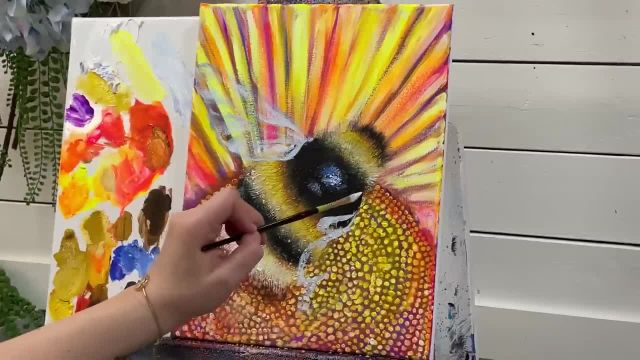 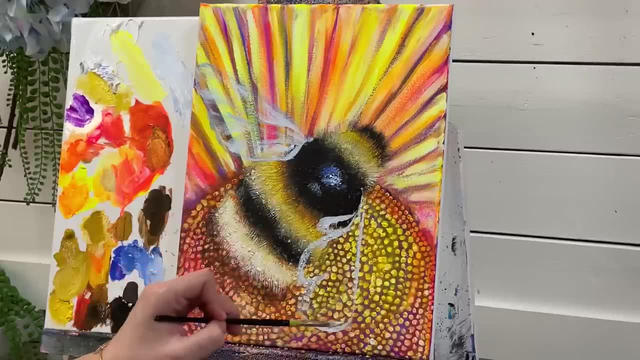 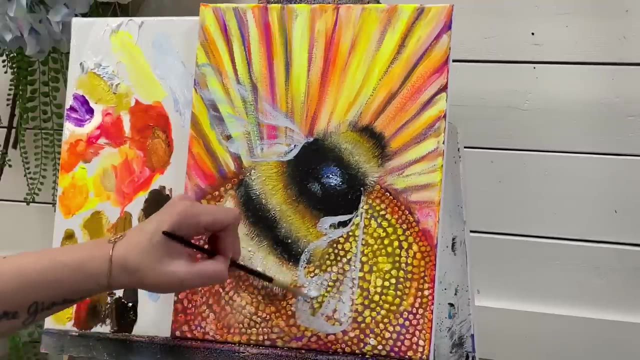 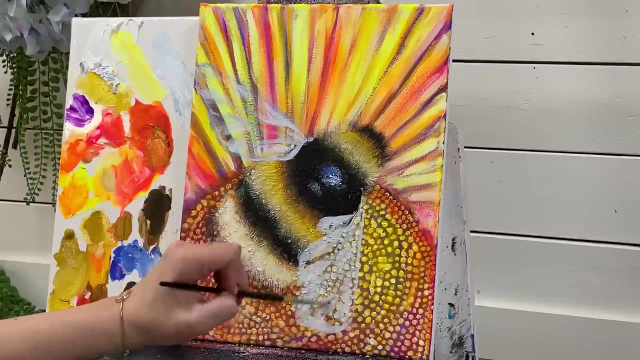 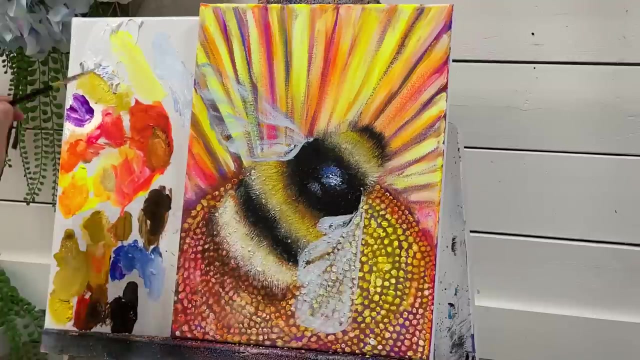 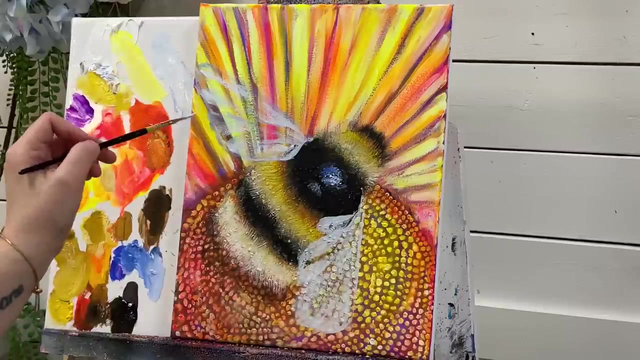 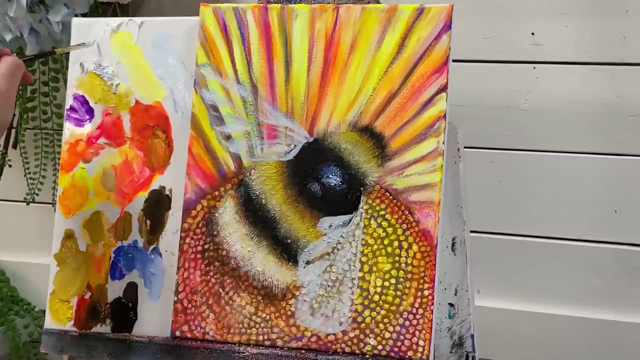 Give you a little bit of water on my brush. We're gonna come from here Straight down And then bring it over A few little shimmers on the wing there with Some of that white and blue. 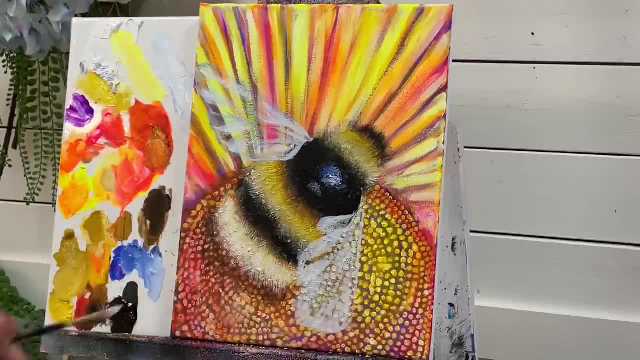 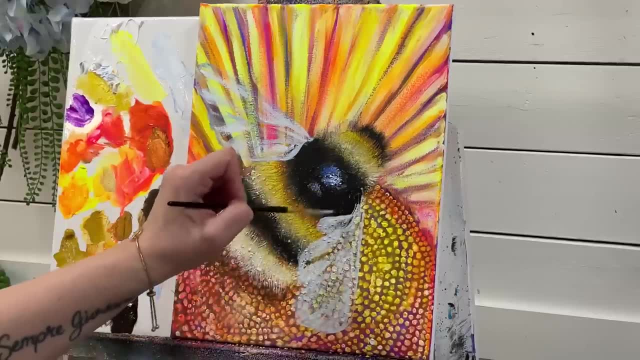 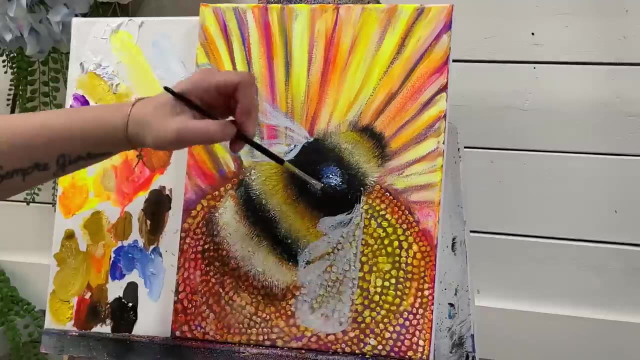 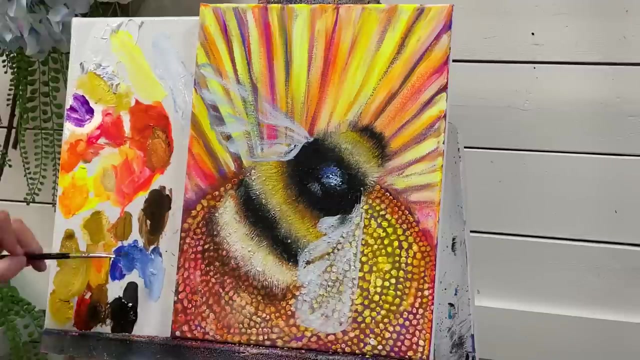 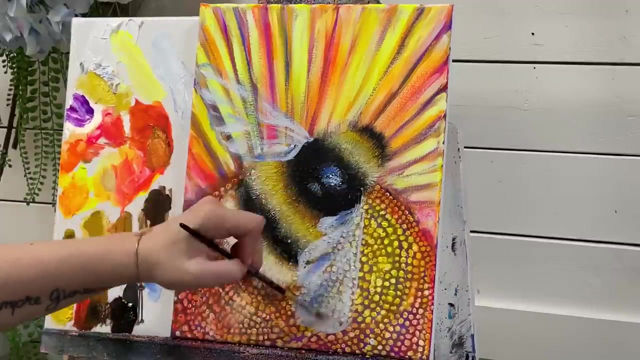 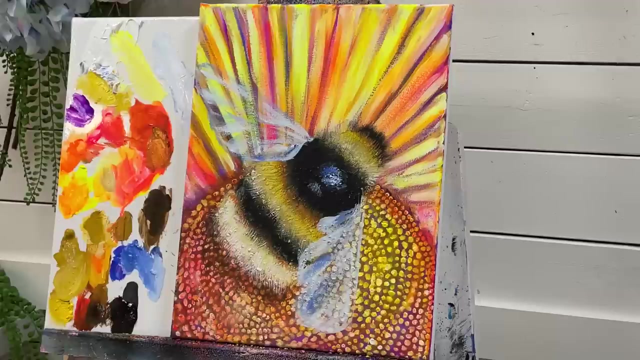 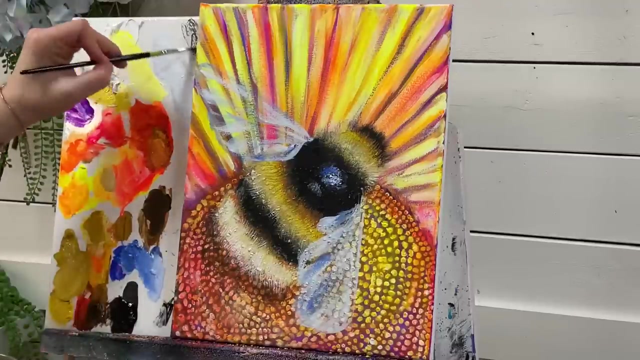 I'm going to rinse my brush out, loosen off a little bit of that, take extra blue this time, Add a little bit of that. Okay, now we're going to take some black water it down, thin it out. 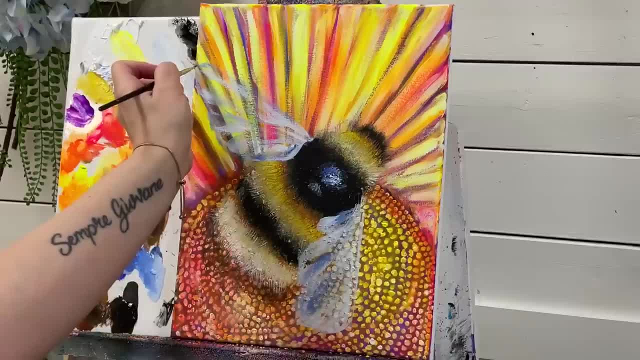 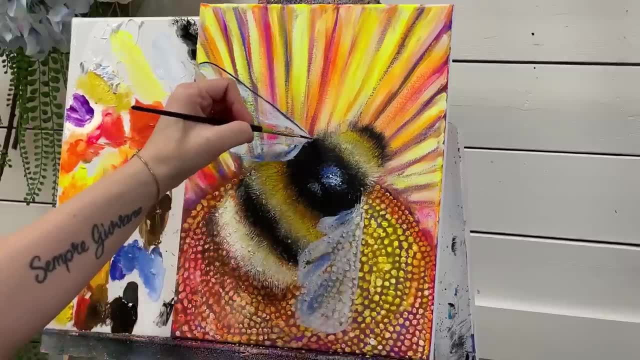 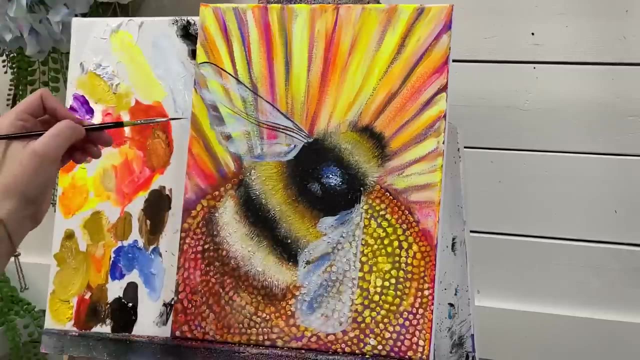 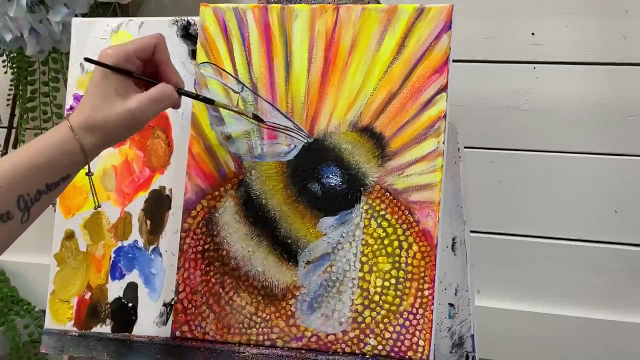 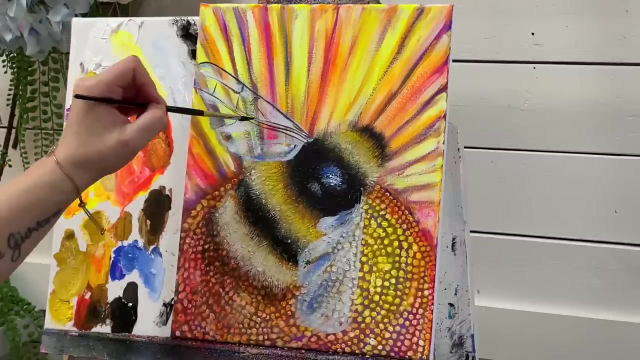 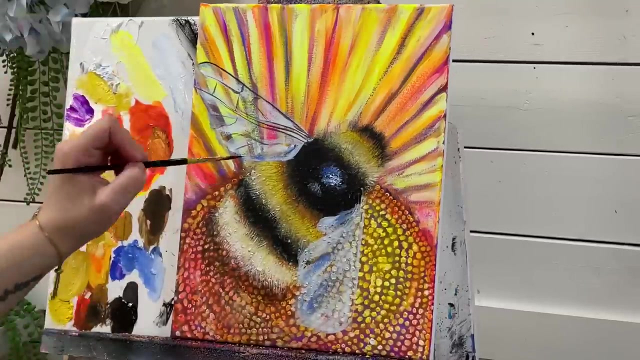 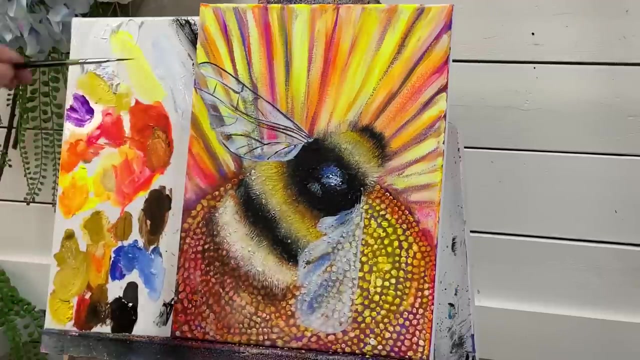 and I'm going to start up here and we're going to bring it all the way down to the body and we're going to add a few little lines and just feel free with it, Make your own pattern. I'm going to do the same thing here. 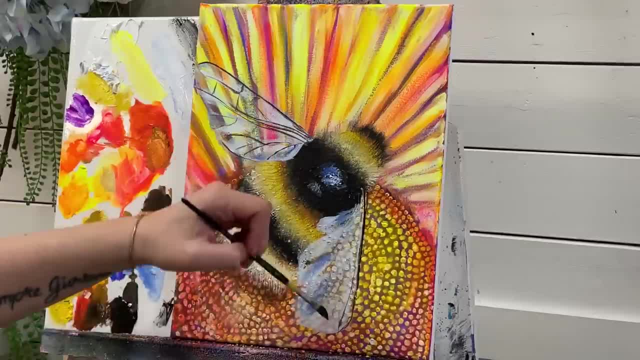 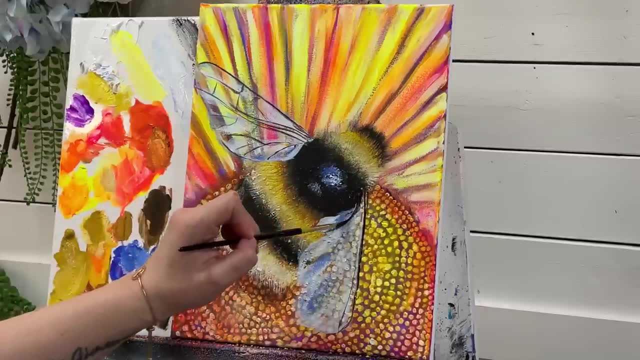 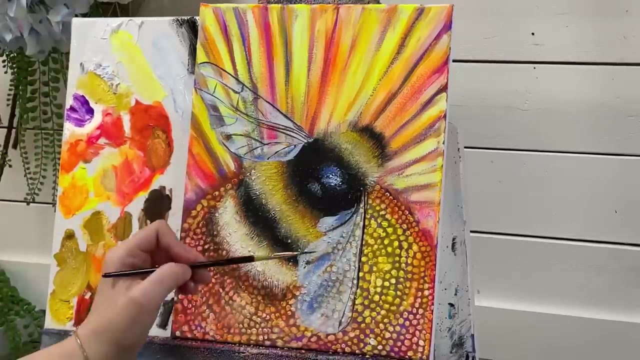 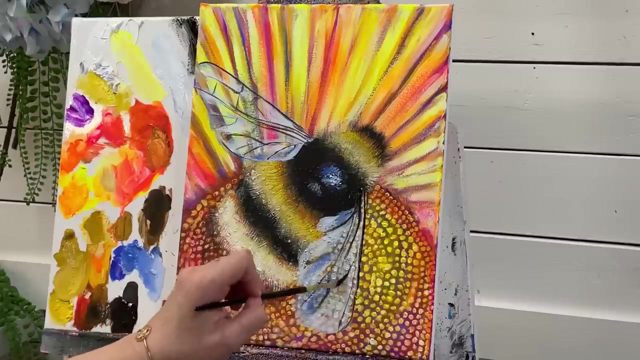 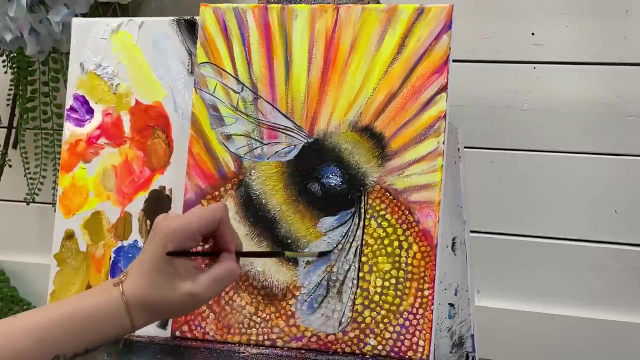 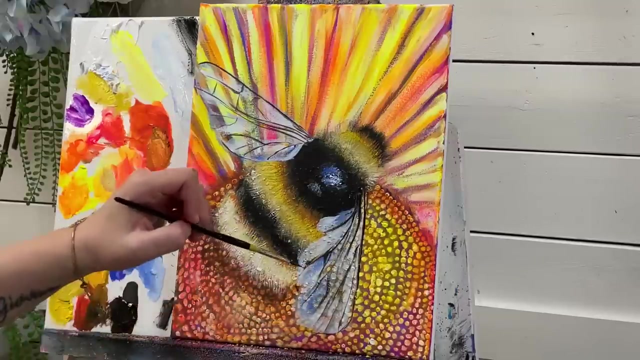 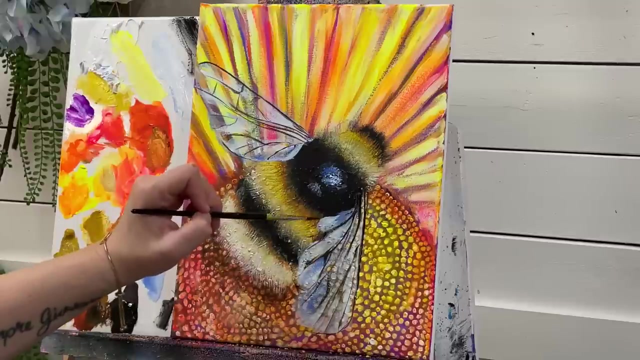 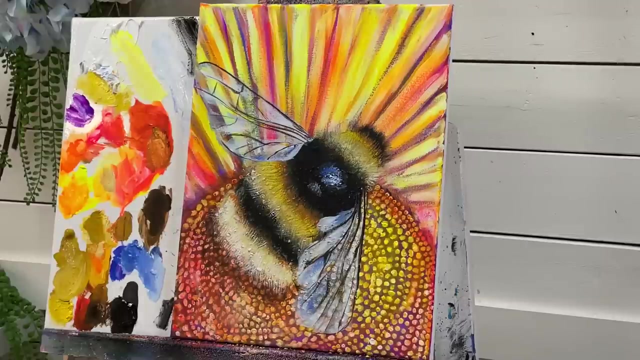 Remember to thin your paint out with a little bit of water so that it makes it easier. Add those little lines and brush strokes. I'm going to add a little bit more of this. Okay, There we go, There we go, We're done. 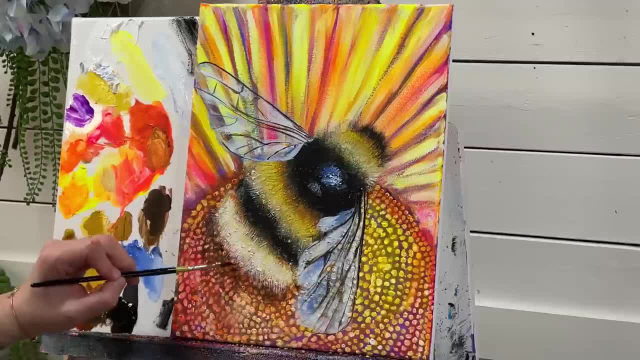 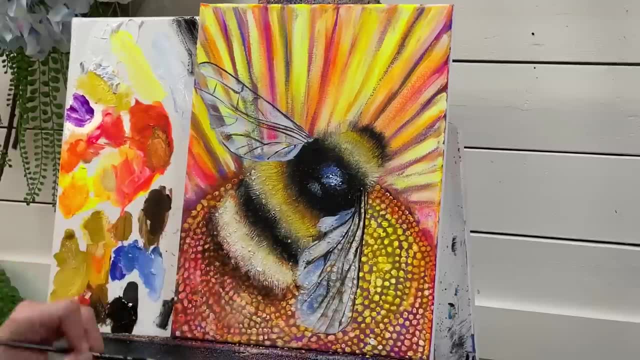 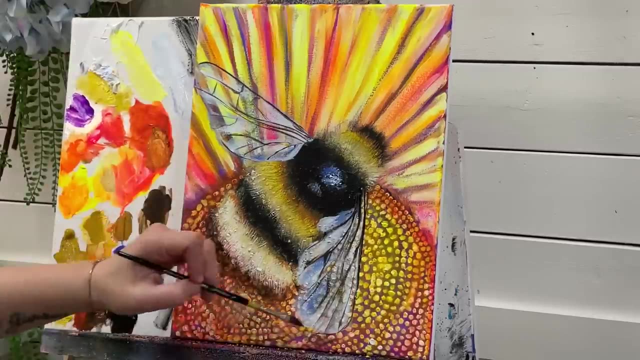 Okay, Okay, my black just around the back here, thinned out for shadow. okay, you don't want it to be too solid. I'm going to add a little bit here for a shadow by the wing or from the wing. that's even a little bit too heavy, so I'm going to. 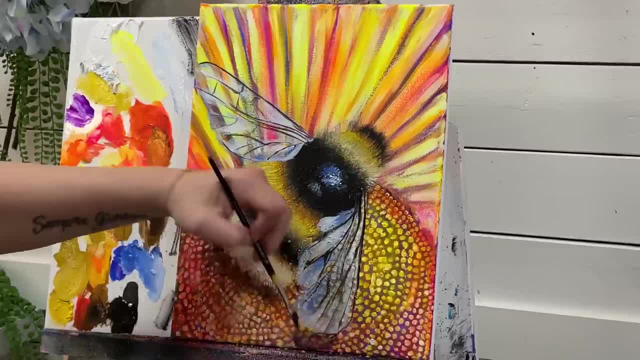 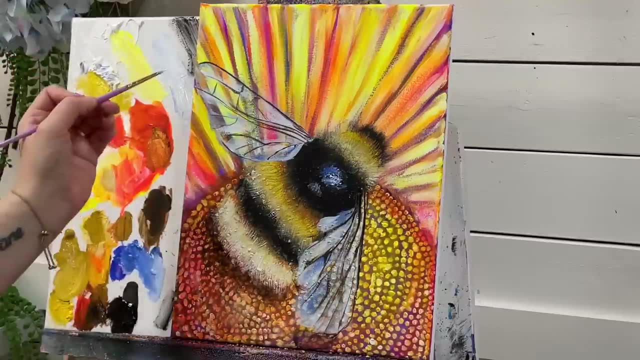 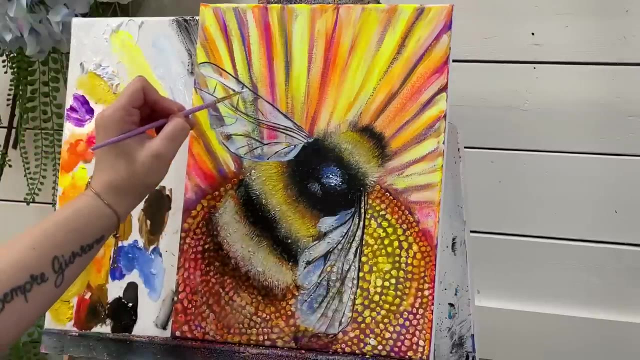 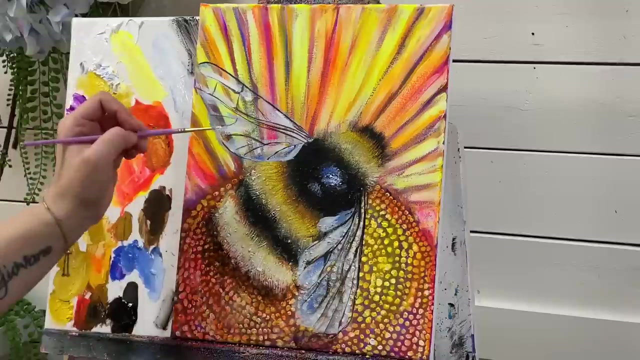 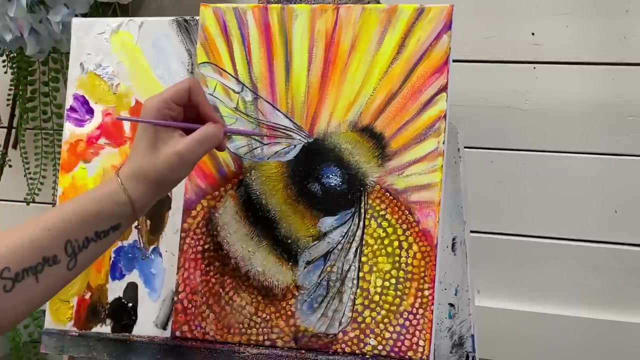 take some of it off. I'm going to use my round brush now and white, and I'm going to add some brighter highlights. you want to keep these looking shimmery and transparent, so you're not going to add white over all of them, we're just. 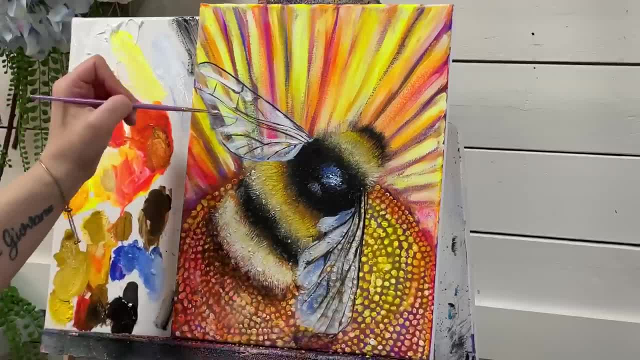 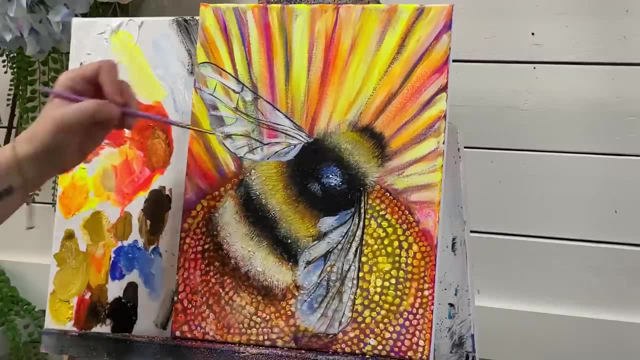 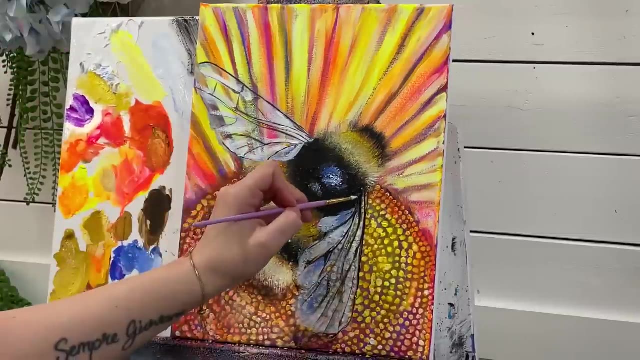 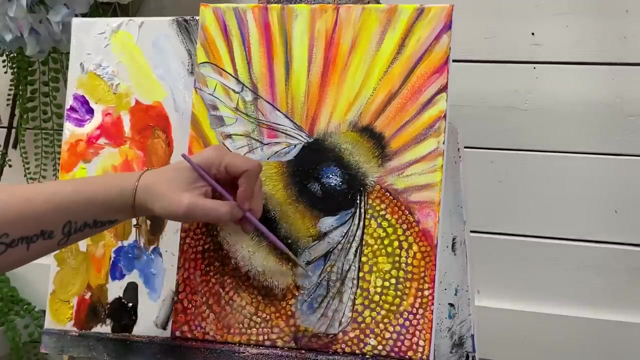 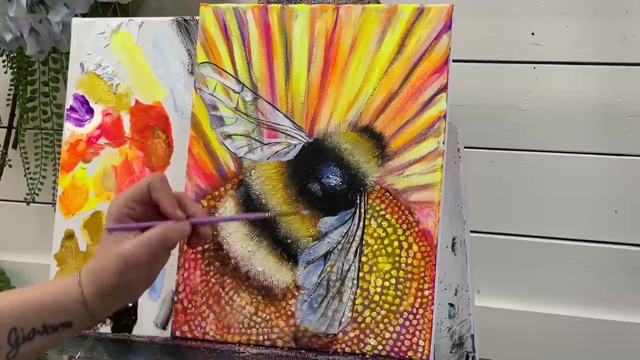 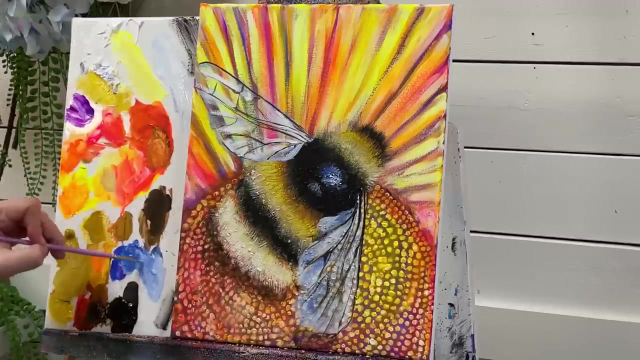 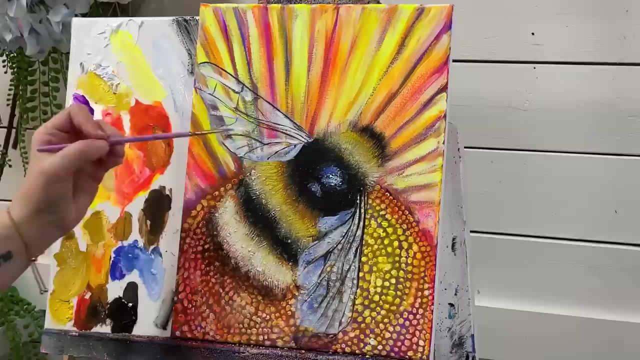 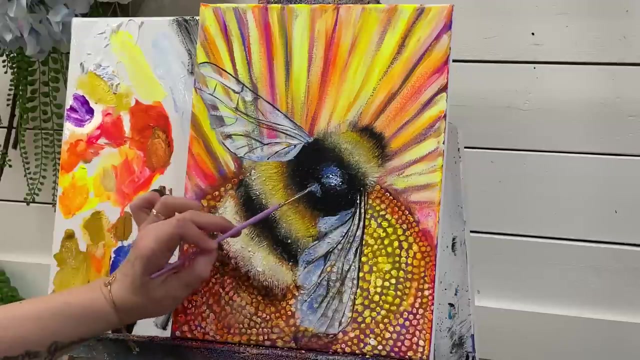 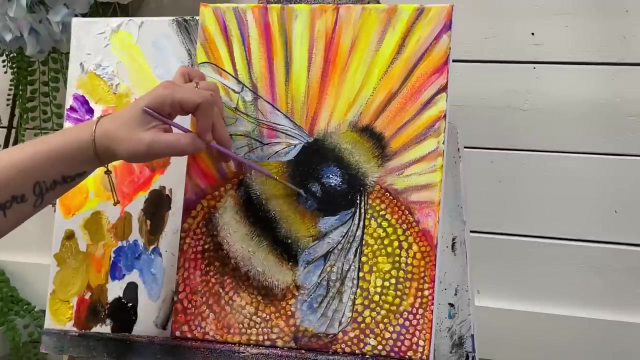 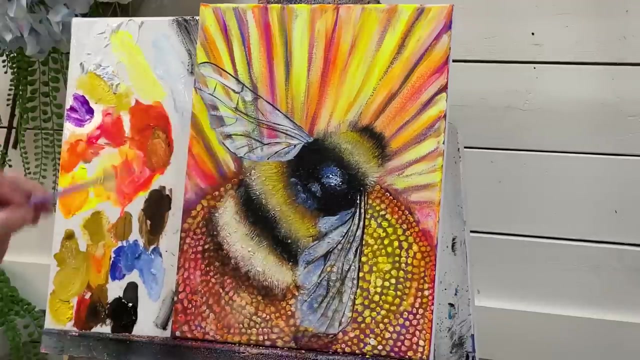 going to pick a few spots a little bit more. a little bit of blue in there. there's just a little bit of blue around here as well, trying to start with some medium, so I'm going to add a little bit of blue here, a little around here for a pop back here. 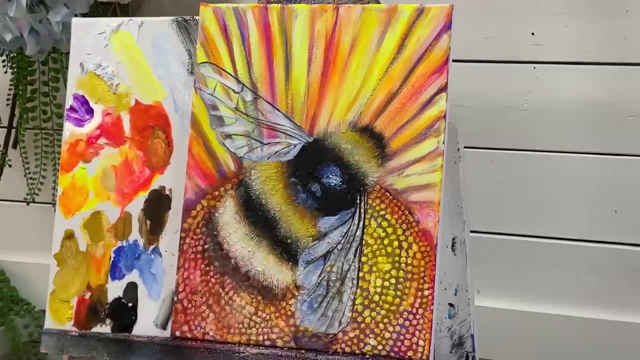 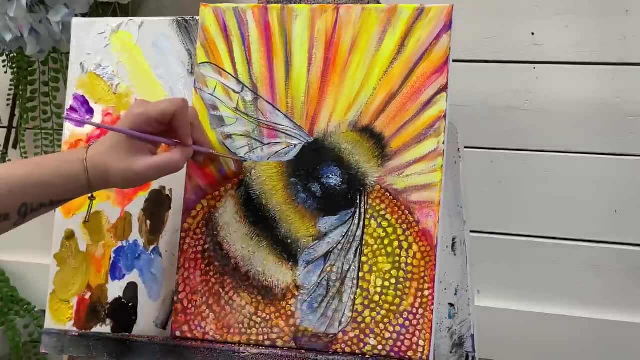 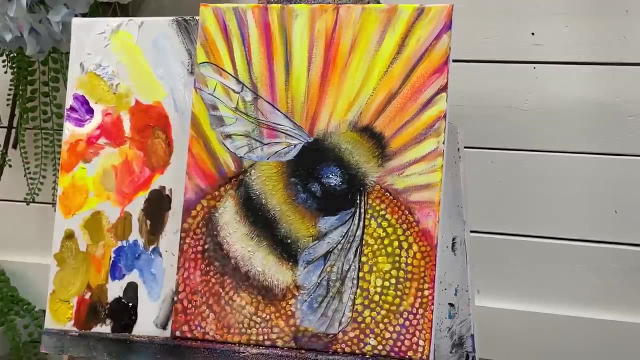 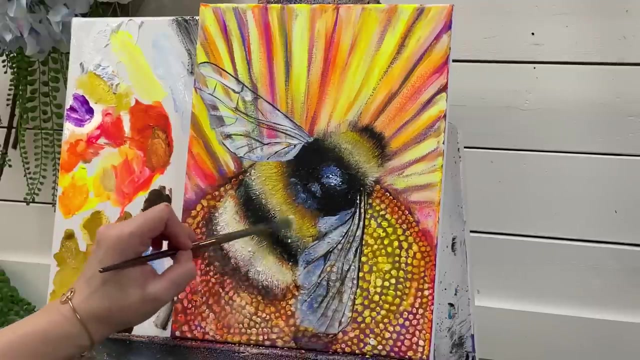 just to get that wet. for some more of a shadow color, I'm going to take a little bit of black. I had just a little bit there and a little bit here, Okay, so now I'm going to add some more highlights using my Zen Filbert. A little bit of water there on there if you have to. 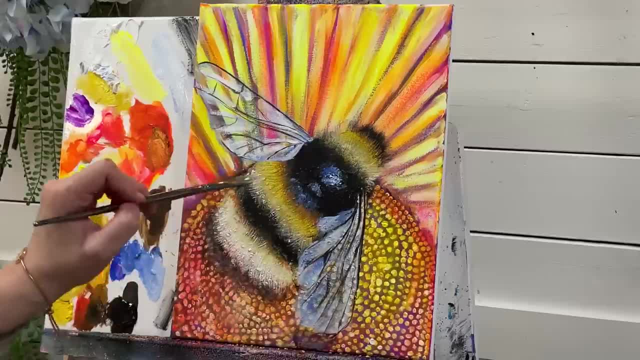 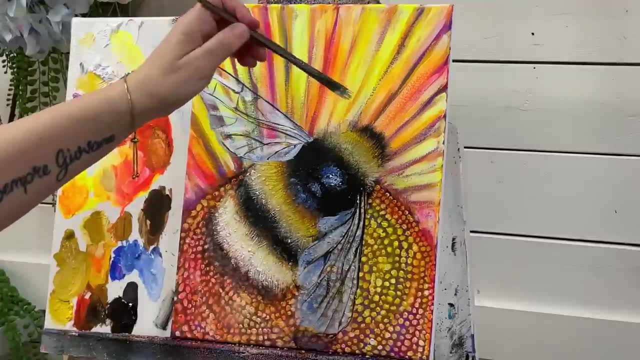 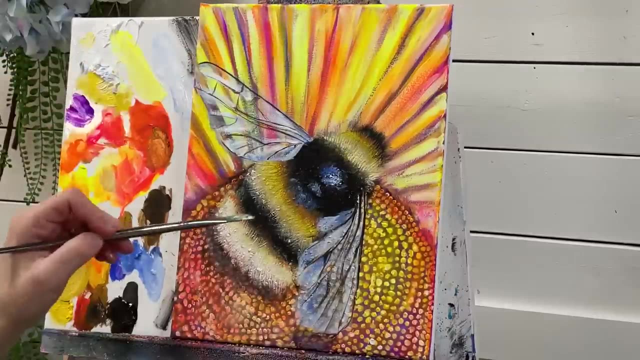 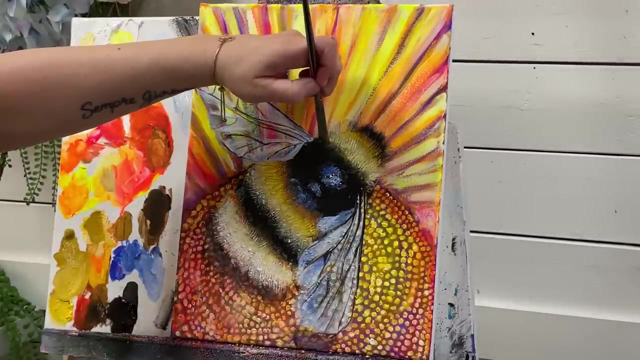 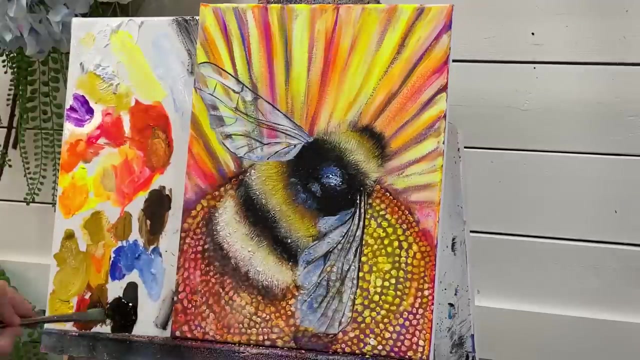 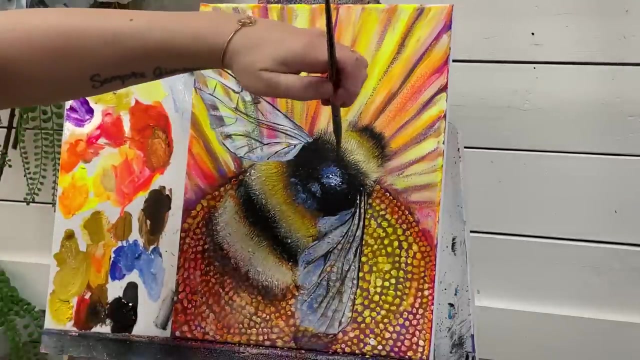 Take some more of the yellow and the white And take a little bit more black, and we're going to go this way Barely touch. So we need a little bit of water on there to release it. It's like using a bunch of liner brushes. 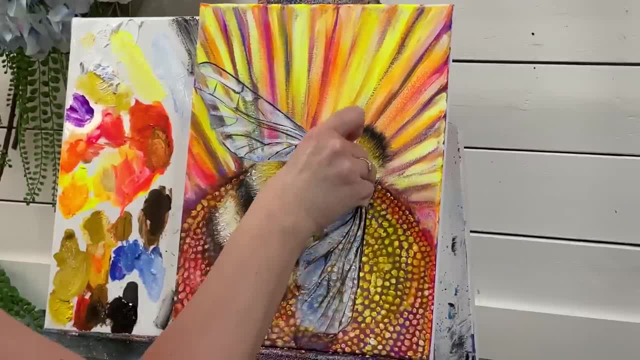 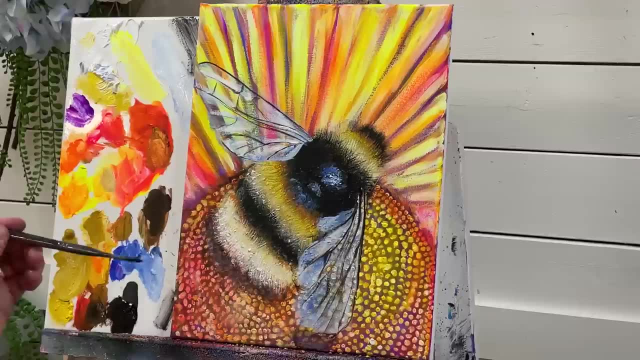 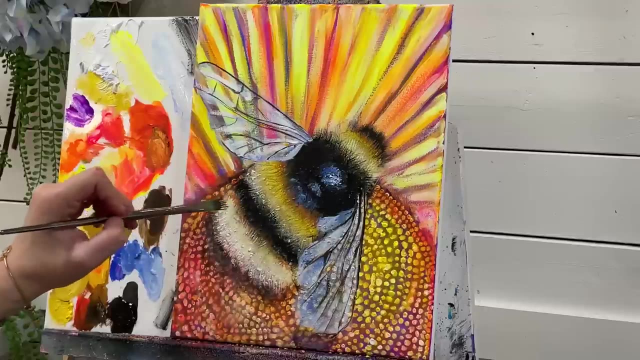 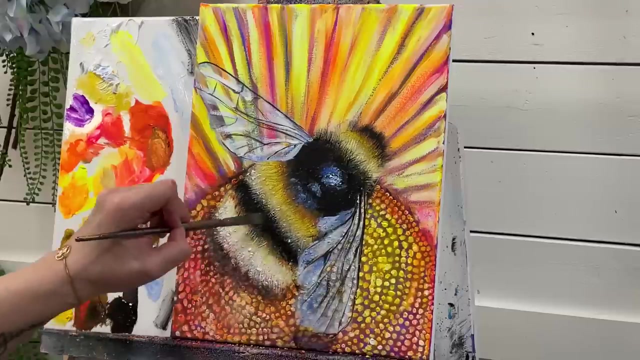 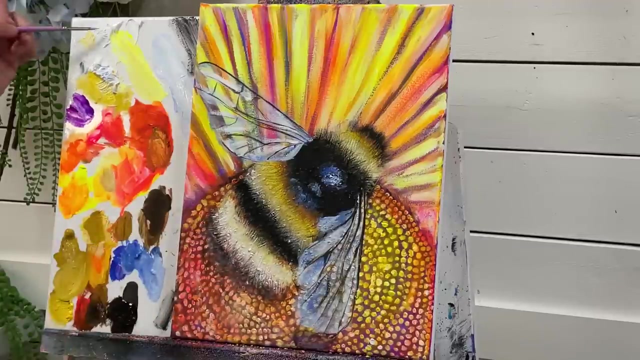 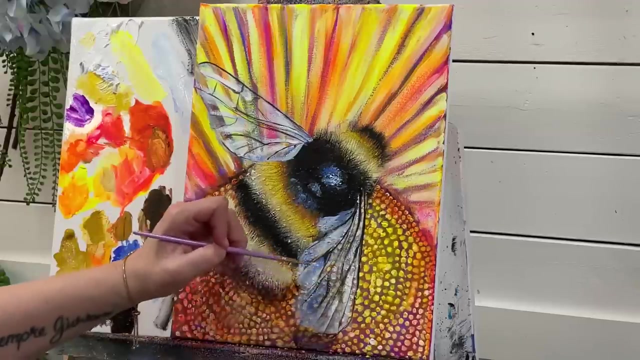 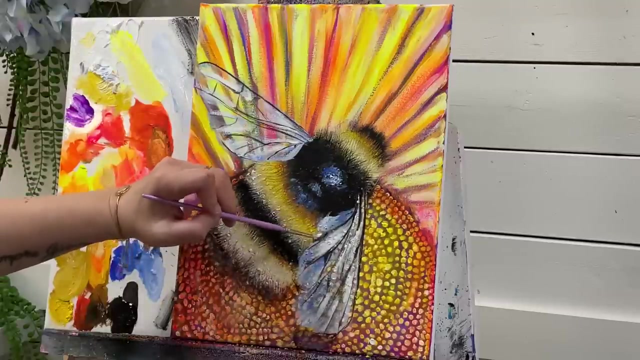 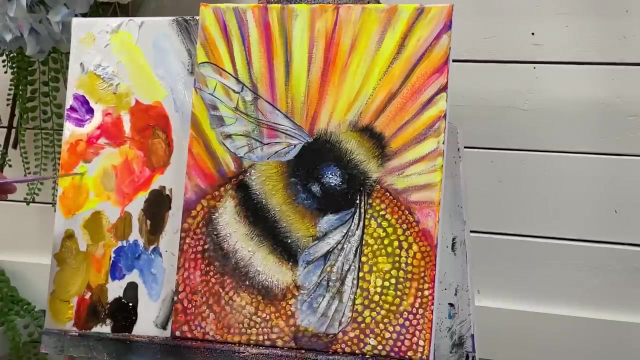 A little bit too much water on there, so I'm going to catch these A little drips and go back over to my round white. we're gonna pick a few spots to add a brighter shimmer to now. i'm just going to add a little bit more. the rest of my it's kind of drying up, but 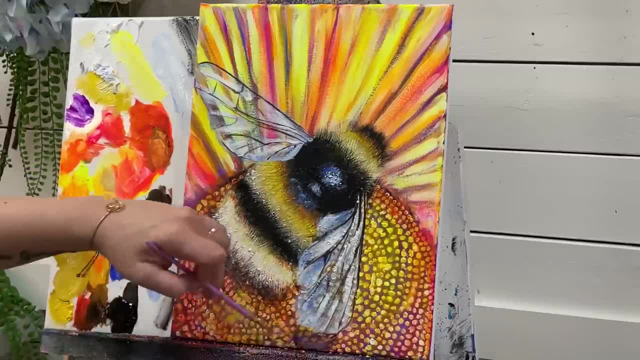 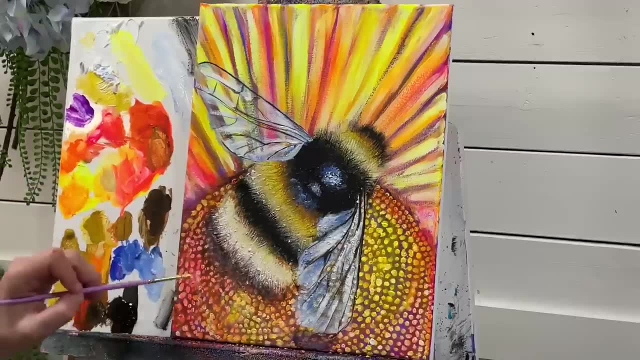 i can still thin it out with some water, not over the shadow area, okay, and then i'm just going to go back over to my round white. we're going to pick a few spots to add a brighter shimmer to, and go back over to my round white. we're going to pick a few spots to add a lighter 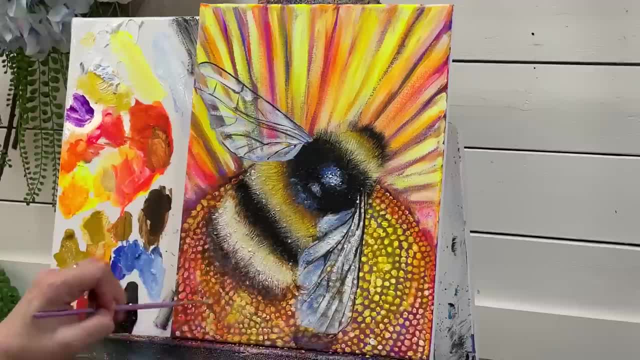 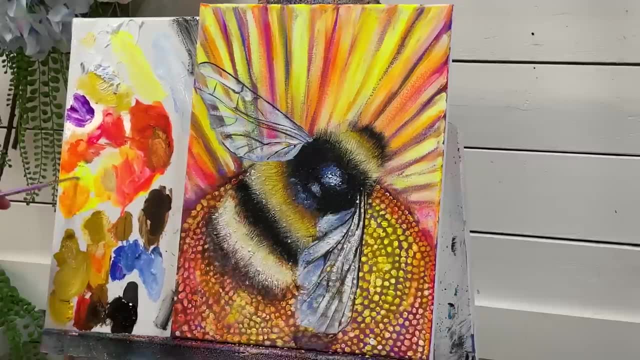 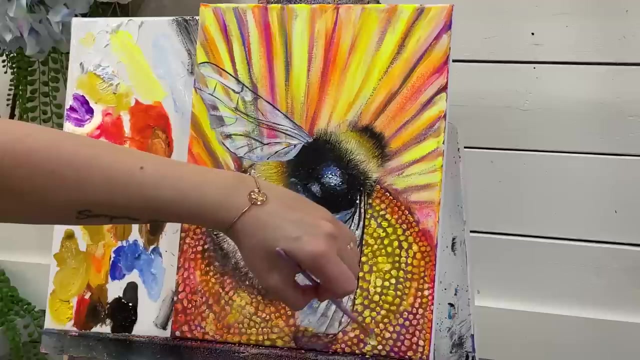 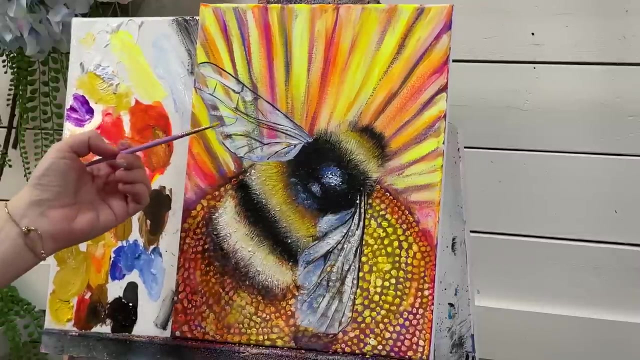 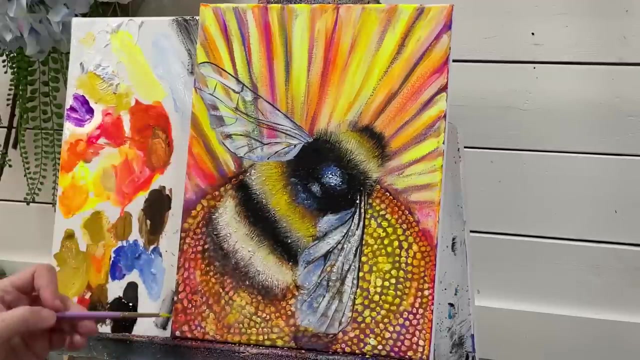 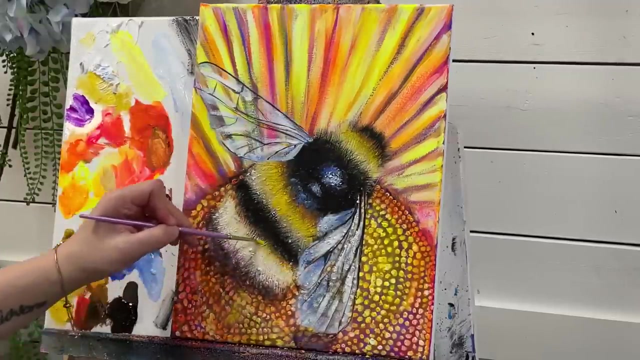 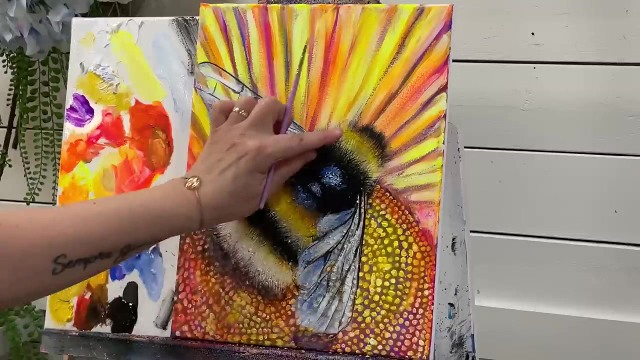 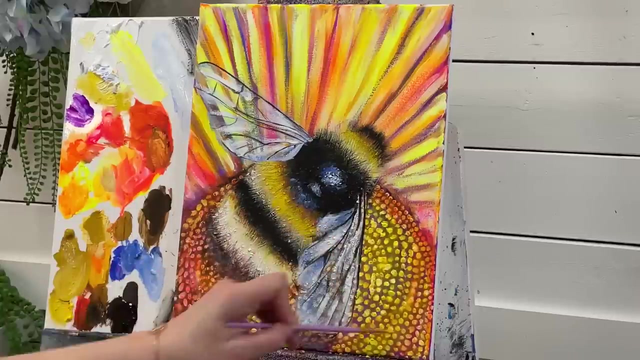 shimmer to just glazing over with my lemon yellow. just glazing over with my lemon yellow, just glazing over with my lemon yellow. Take a tiny bit of cadmium yellow, just add a little bit right over the burnt sienna, a little bit over here and a little bit right here. 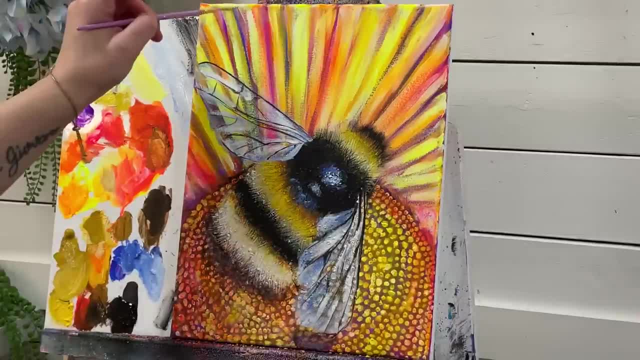 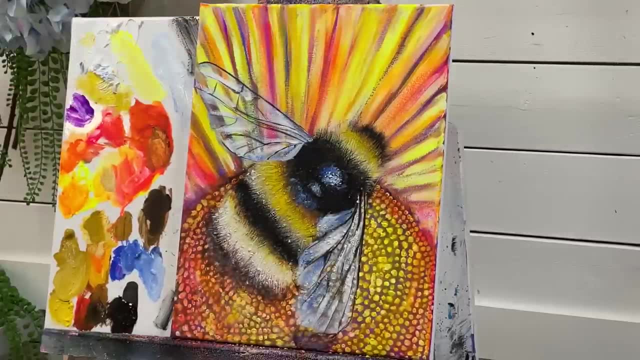 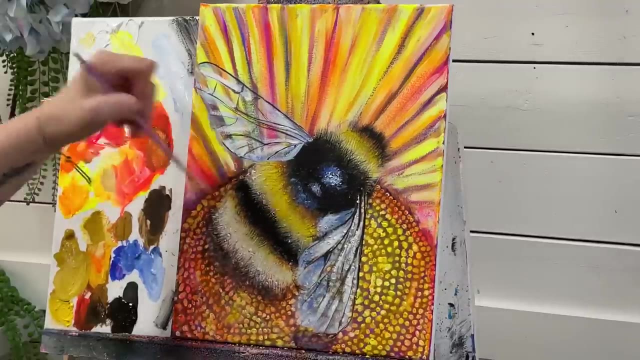 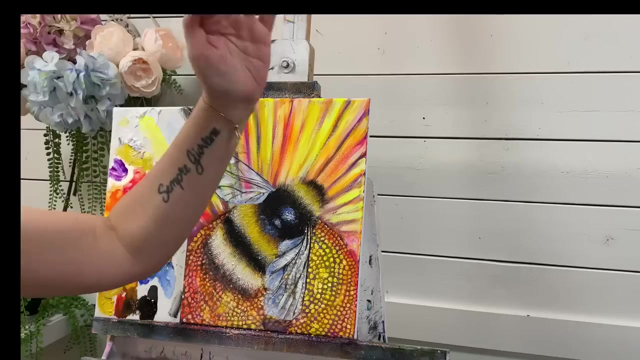 Okay, I hope you guys have enjoyed watching this one. This is my very first bump And I want to wish you guys all the best. take care, and I will see you very soon in my next video. Bye.